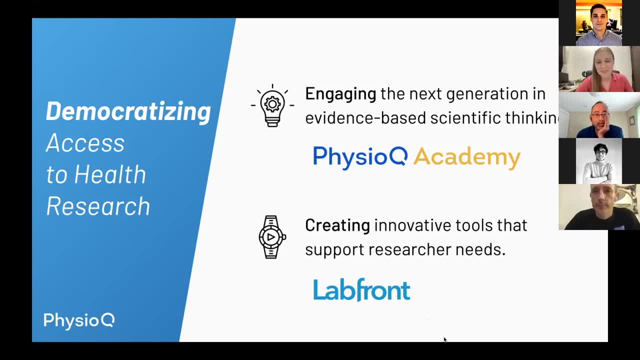 And actually, in fact, about Andrew. he was the lead medical advisor for the team dynamical biomarkers, the runners-up winners for the famous $10 million Qualcomm XPRIZE tricorder competition, So we are extremely grateful to have him here today with us to share his knowledge on HRV and Dr. 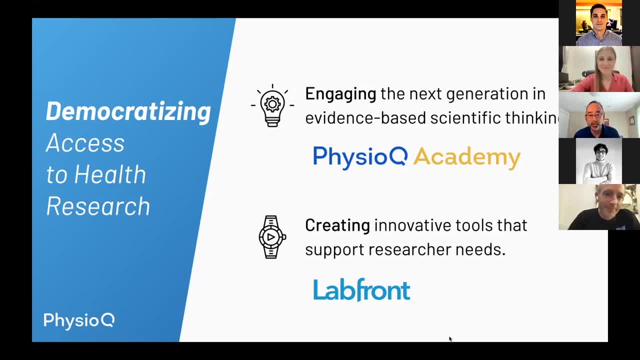 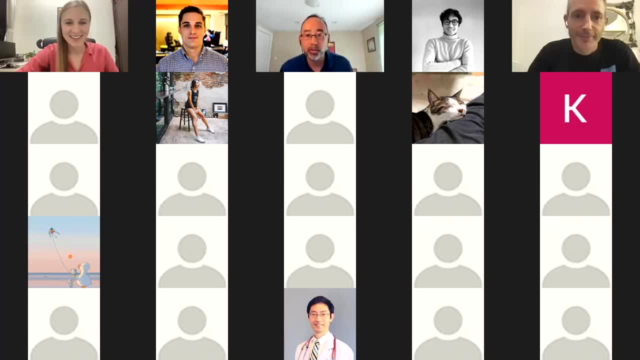 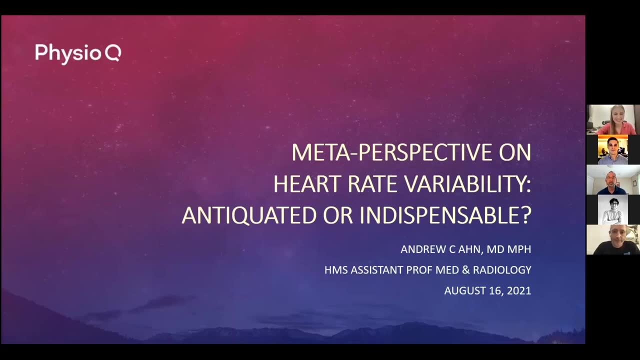 Andrew Ahn, you have the virtual floor. Welcome, Great Thank you, Jess. Thanks for the introduction. Let me see if I can share my screen real quick. okay, let's see, all right, so is that? can you see the the screen? yeah, it's perfect, perfect, okay, so um hold on. 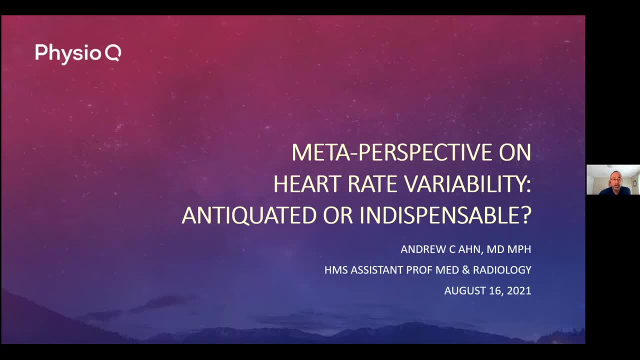 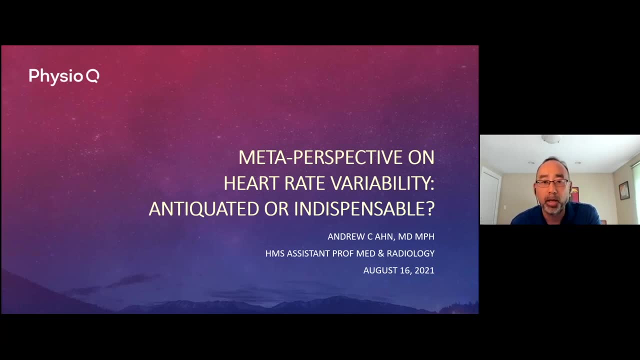 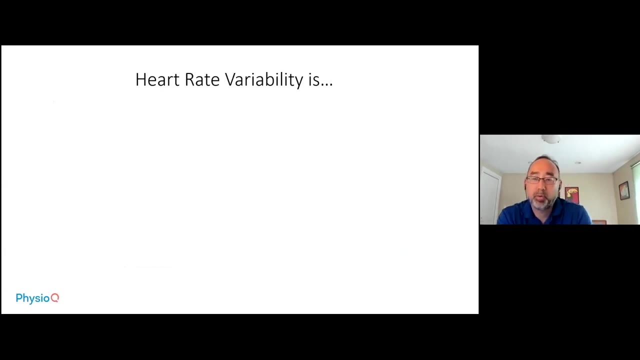 so the title of my talk is meta perspective and heart rate variability antiquated. is heart rate variability antiquated or indispensable? and um, this is my quick disclosure slide. and um the reason i titled the talk this way was to highlight the differences in views towards heart rate variability, the views that are often divided along occupational 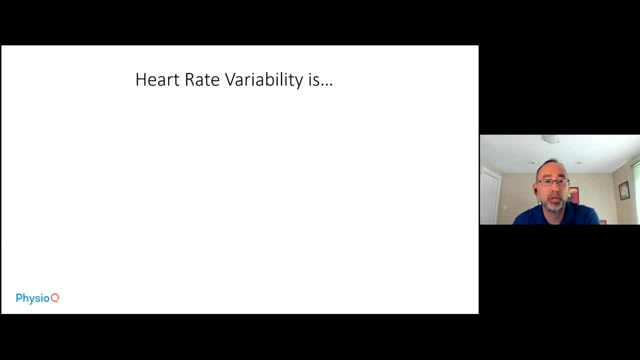 disciplinary lines. so if you ask a clinician in health care setting the uh, the response you may say you get is that heart rate variability is antiquated. on the other hand, something's going on with my slides, okay. on the other hand, if you ask an athlete or a silicon entrepreneur seeking to optimize physical or cognitive performance, 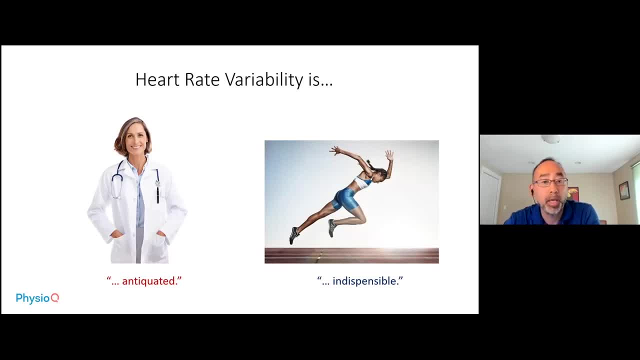 they may say their heart rate variability is really important and indispensable. personally, as a clinician and a researcher of wearable devices, i find this divide really fascinating, and i'm also acutely aware that the divide is larger than many will recognize, because many physicians are simply not aware that heart rate variability is widely espoused as a marker of 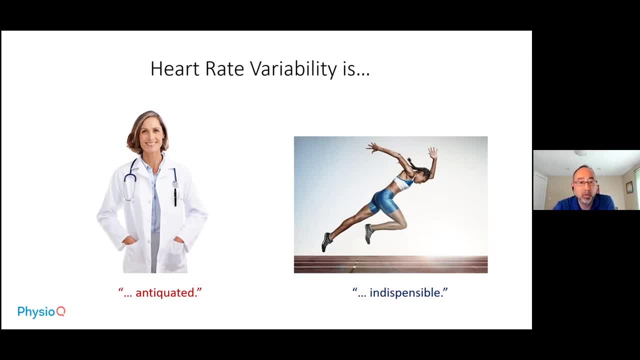 health and performance, while many athletes have little idea how skeptical the medical community may be towards heart rate variability. the other day i was listening to a podcast on heart rate variability and one of the speakers was saying that heart rate variability is sort of commonly used in the clinical setting. 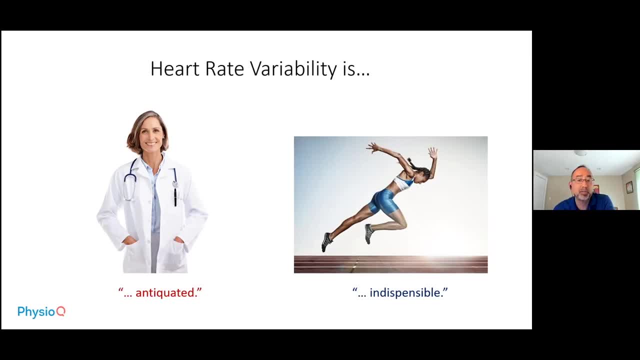 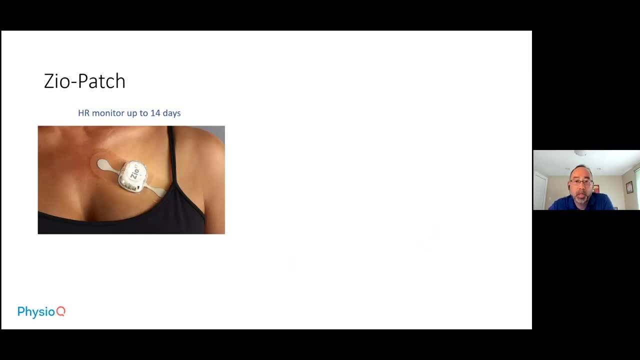 for diagnostic and prognostic purposes- and i have to say that's really not the case- and to to show that um sort of indicate to illustrate this in the hospital a lot in the hospital we utilize something called the xyle patch. it's an fda approved heart rate monitor which can you can keep on for up to 14. 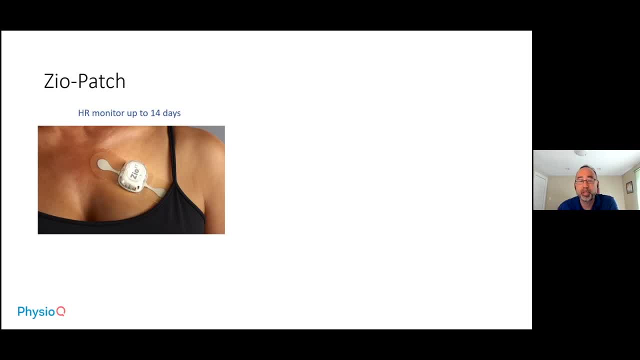 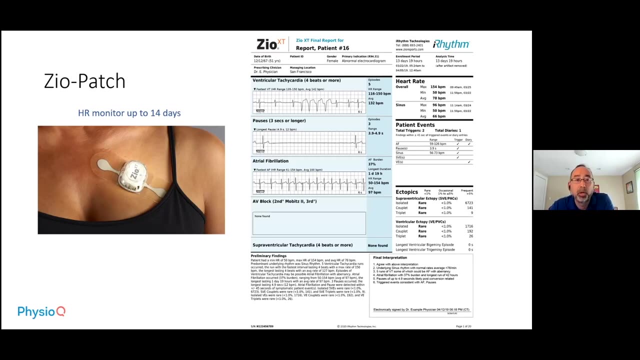 days, and when someone gets admitted to the hospital for syncope, which is loss of consciousness, chest pain or palpitations, we send people home with this xyle patch. and when you get the actual medical report- this is the actual medical report. actually it's a sample of someone- you can see that. 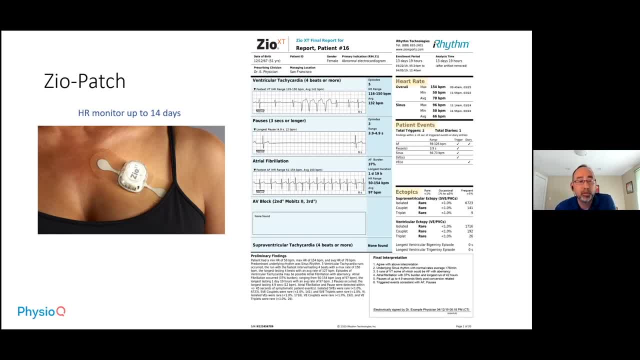 they present a lot of the information, such as heart rate variability. they include arrhythmias such as ventricular tachycardia, atrial fibrillation, sinus pauses and various activities, but nowhere in there is there anything about heart rate variability. and you would think that with something like this device, which is a perfect instrument for heart rate. 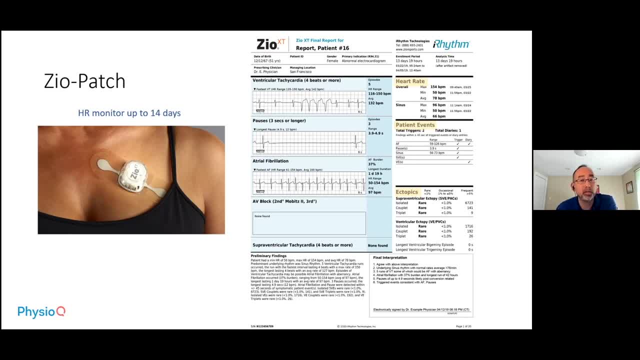 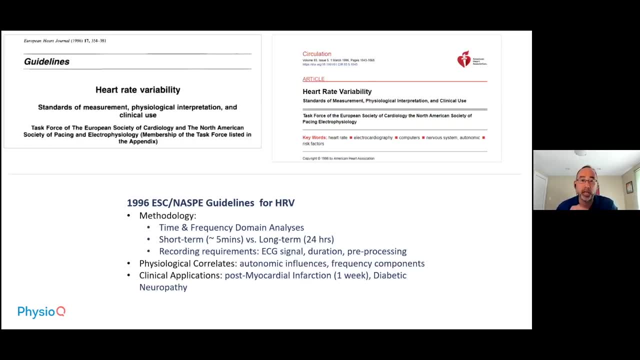 variability that that would be included in this, but simply it's not included because it's heart rate variability is not used in the clinical setting. the last time any medical professional put up a major position or a consensus paper in heart rate variability was in 1996.. it was a joint. 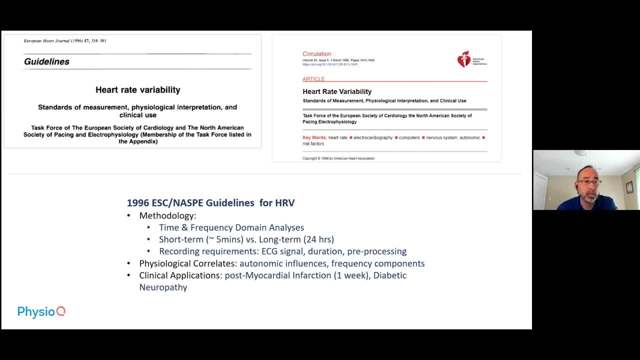 statement placed, put out by the european society of cardiology and the north american society of pacing electrophysiology and published in the two big journals, european heart journal and the circulation journal, and it sort of quickly went over, uh, reviewed some of the literature and provided some guidelines. they talked a little bit about the methodology of heart rate variability. 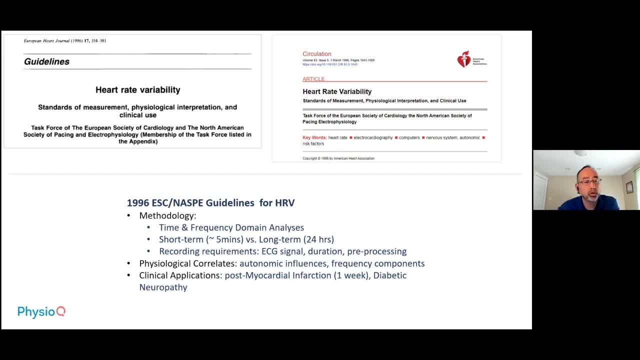 uh time and frequency domain analysis, short-term versus long-term acquisition of heart rate data and some of the recording requirements, such as the ecg signal, the duration, the pre-processing that you needed of the signals. they also talked about the physiological correlates, including autonomic influences, the frequency components and then some of the clinical applications. actually, 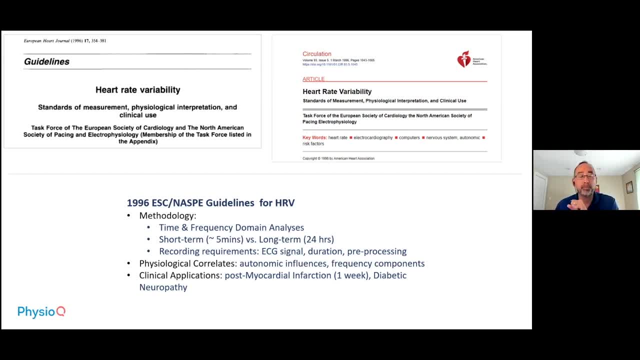 they only identified two post-myocardial infarction, so you could obtain heart rate variability one week after an acute end-life, and that information was found useful to determine whether someone was at risk of arrhythmia or death. and then the the diagnosis of diabetic neuropathy. now, this was highly cited, but again, this was in. 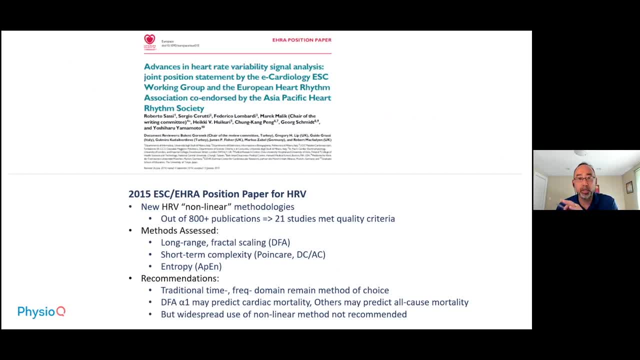 1996.. the only follow-up was done of this paper was done in 2015 and it talked largely about non-linear methodologies, which i won't be talking on this talk. it would be in subsequent talks for the series and this basically the same group, the european society of 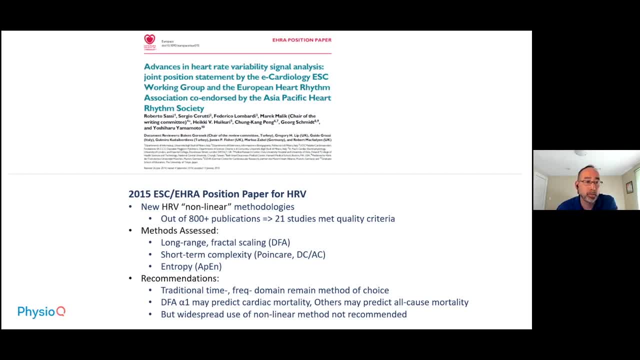 cardiology and another european heart rhythm association reviewed a number of heart rate variability, non-linear methodologies, publications- out of 800 plus, and found that 21 studies met quality criteria. and then these are sort of the various methods that were evaluated, including d100, frequency analysis, ponkari, deceleration capacity, acceleration capacity, entropy. i'm not going to go. 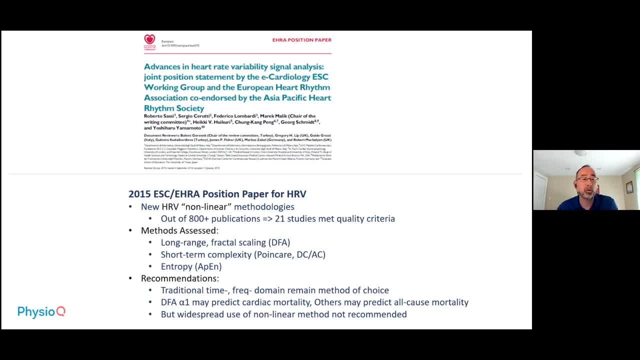 into too much details, but their recommendations was ultimately that traditional measures, which were discussed in the prior guidelines in 1996, was the remains the method of choice, and widespread use of non-linear methods was not recommended. so this was the most recent update that was given by any sort of large medical professional society and it was a 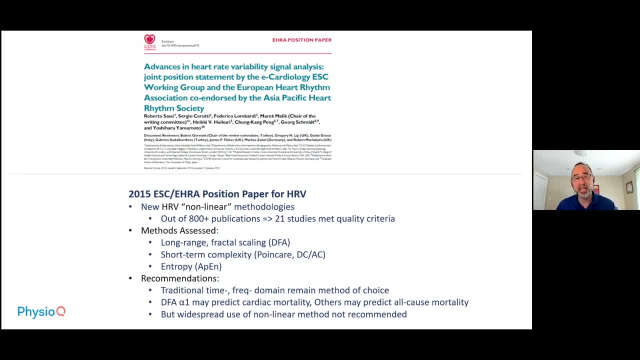 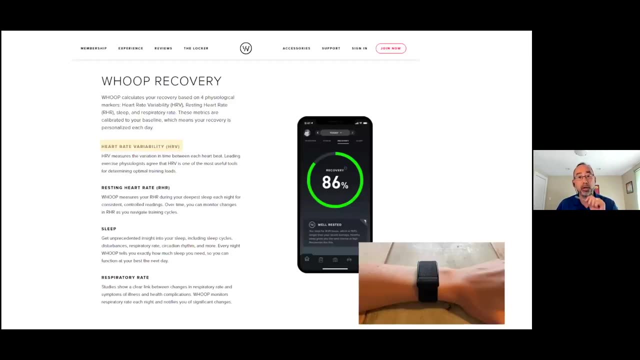 published in a much smaller journal called europace, and it really didn't get much citations. so, um, you know clearly the the importance of heart variability in medical establishment is in question, and so it hasn't been widely utilized. on on now, contrast this with how wearable companies use heart rate variability. 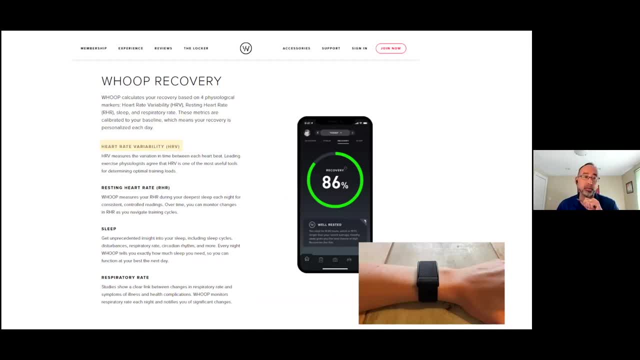 and often consider it as a cornerstone for the app functionality. so whoop is a well-known uh company that has its own device in its app and they have a measure called whoop recovery and one of the cornerstone of this measurement recovery is heart rate variability. in addition, 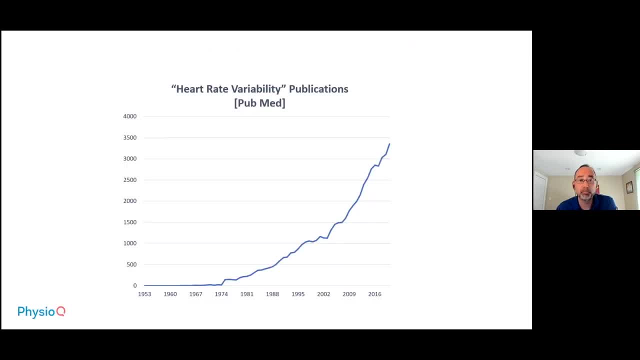 to resting, heart rate, sleep and respiratory rate. and this enthusiasm towards heart rate variability is not limited to wherever the world. in fact, heart rate variability has garnered a steady rise in interest in the actual peer-reviewed sciences, and if you do a literate research on the number of heart rate variability related publications, you will find that there. 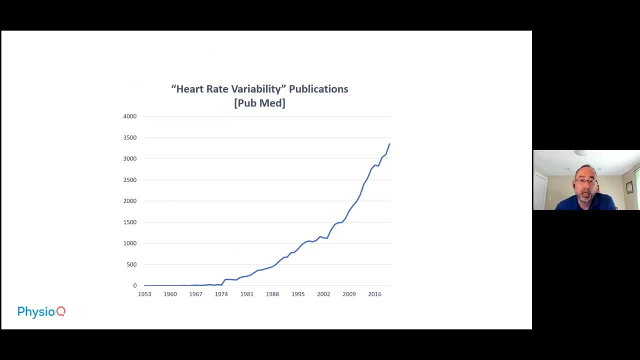 has been a significant increase over the past three decades, even more so than you would anticipate, based on the rise of number of journals and the growth of science alone. so where does the truth exist and why is there such a contrast in enthusiasm here and some of the hints as to why this growth has occurred and maybe how some of these disparities 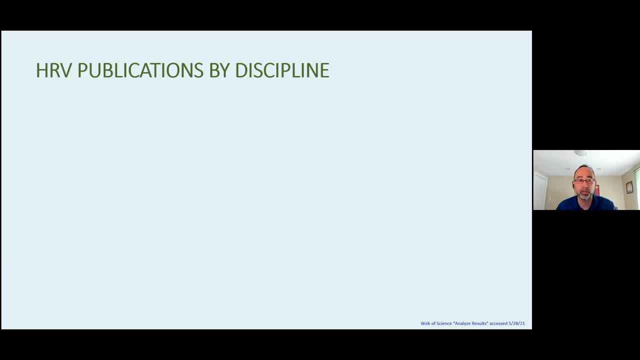 and this differences. in this perspective, heart rate ability has arisen from is to. you can take a look at the number of publications by discipline, and so what i did here was i took the number of publications divided, pulling to discipline by decades, and you can see here- sorry, i'm having trouble with my mouse. 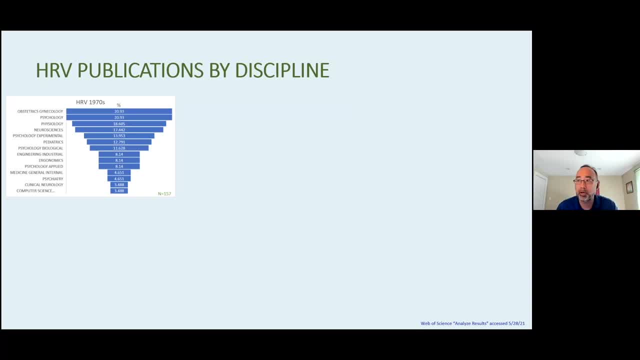 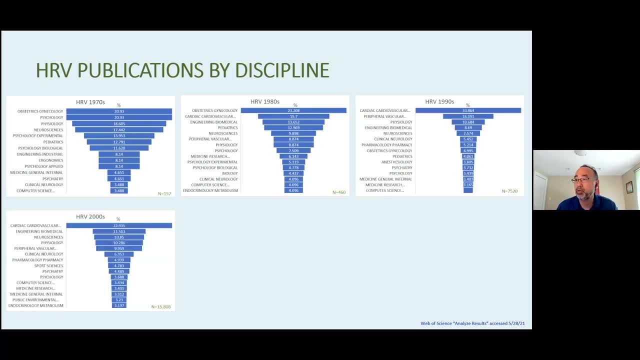 is that into 1990- 70s, you have 157 total publications. 1980, 460, 1990, 7000, 2000- about fifteen hundred fifteen thousand. heart rate variability, 2010- about twenty eight thousand. and then just in the 2020s alone, which is just 2020 and 2021, already we have nearly five thousand. 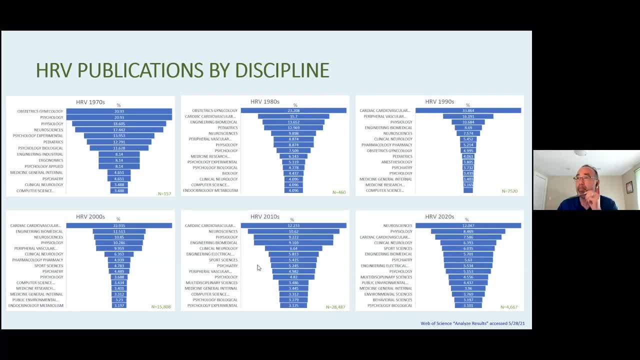 publications and if you take a look a little bit of the patterns of this heart rate variability publications, you can notice that in the beginning 1970s and 1980s obstructive gynecology was the leading discipline that published in heart rate variability. and why is that? 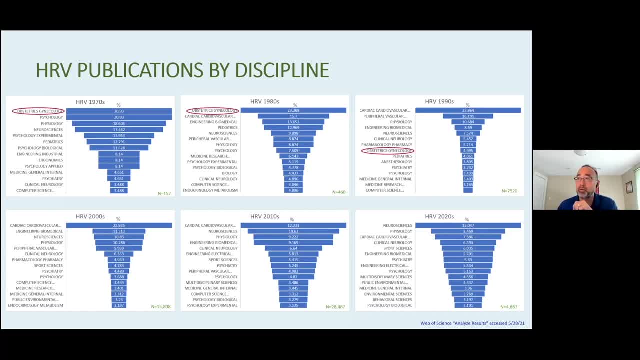 was because fetal heart rate monitoring was sort of became popular and now has become the standard practice and you can see that obstructive gynecology is no longer sort of the prominent discipline that publishes in heart rate variability. then came the cardiac and cardiovascular fields and in the 1990s and 2000s they essentially dominated in publications. 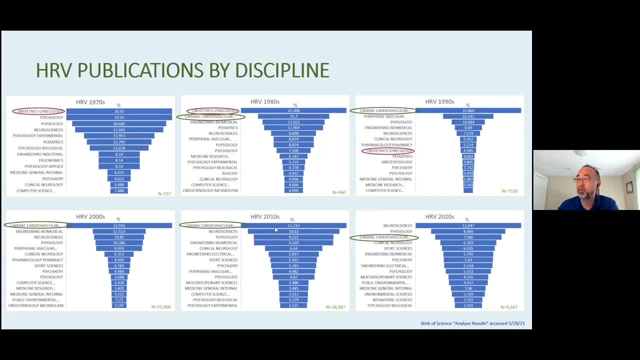 in heart rate variability, and then the domination slowly sort of withered away and then they lost their lead in 2020.. And if you take a look at the neurosciences, you can see that in the beginning they're, you know, continue to be present throughout the decades. but in the beginning, 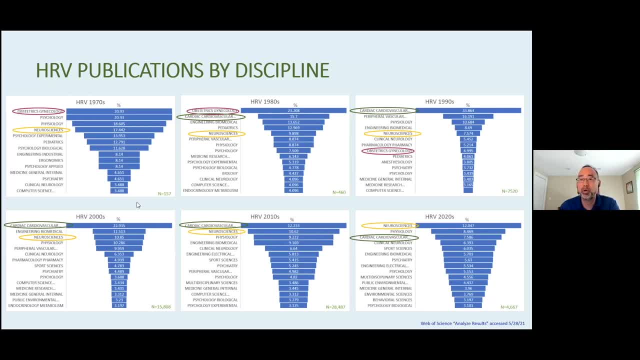 in the first three decades or so, a lot of the focus was on sort of autonomic nervous conditions such as diabetic neuropathy, the re-innervations of transplanted hearts and some other autonomic nervous conditions, But then later in the 2010s and 2020s, the reason it really sort of gained. 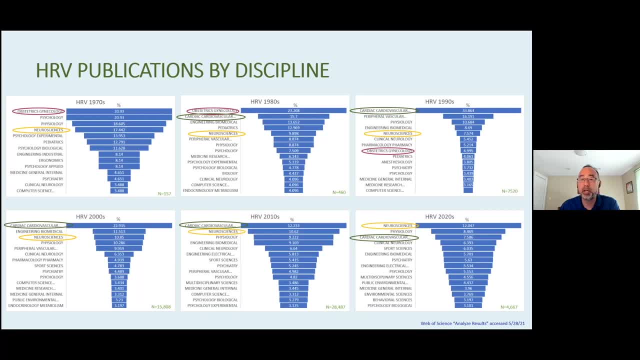 prominence was because of the development of neuroimaging and neurotechnologies in the recent decades. And then you can see that engineering and biomedical came into the foray and sort of came into view, And the 2010s and 2020s and in sports science also became significantly important. 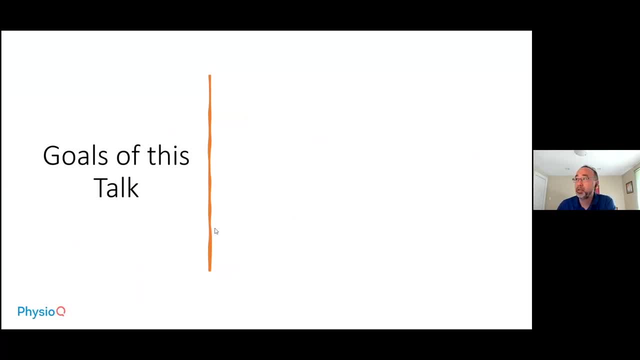 So the goals of this talk is to appreciate how science of heart rate variability has evolved over the past 50 years, recognize the various ways heart rate variability is measured, obtain a basic understanding of heart rate variability physiology, and to understand how different perspectives of heart rate variability has emerged. 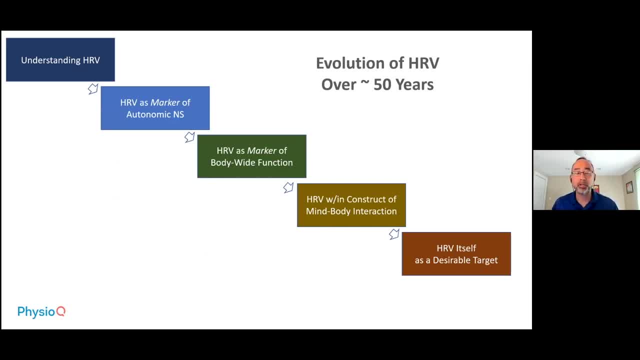 And to sort of illustrate the way I interpret how heart rate variability has evolved over the years, I have put together sort of divided into five stages, And this is based on the prevailing scientific paradigms that existed in each of these stages And unfortunately I won't be able to go. 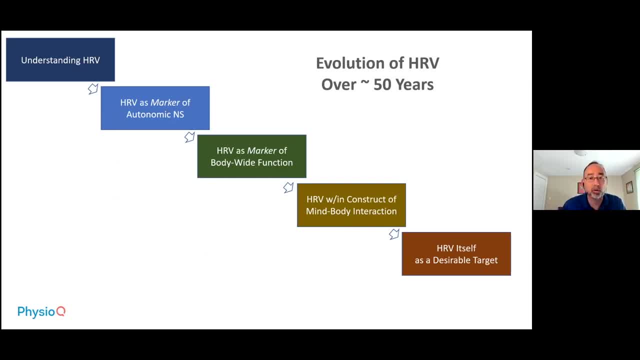 through all of these five stages. It will probably take three talks overall to go over all of them. But you know, I think as of today we're going to be able to go through all of them And I think, as of today, we'll just largely focus on part one: understanding heart rate variability. 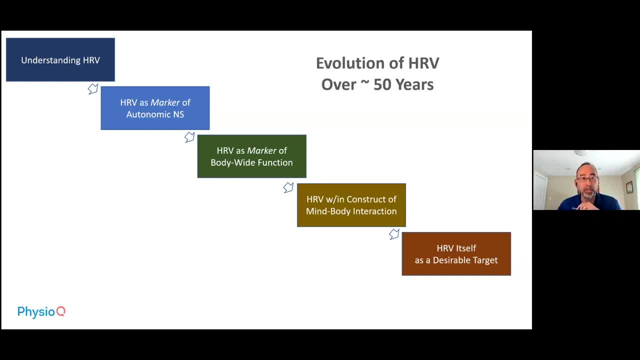 And the stages are: first understanding heart rate variability, and then heart rate variability as a marker of autonomic nervous system, then heart rate variability as a marker of body-wide function, heart rate variability within the construct of mind-body interaction, and then, finally, the heart rate variability itself as a desirable target. 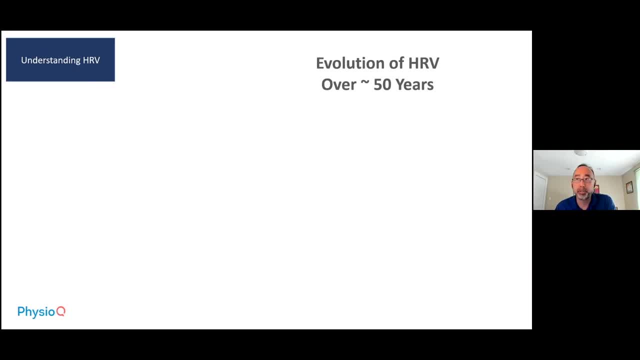 So the first stage understanding heart rate variability happened to the 1970s and 1980s predominantly, where there was a focus in physiology and development of methods. In my view, 1970s to 1980s was the golden age of physiology. 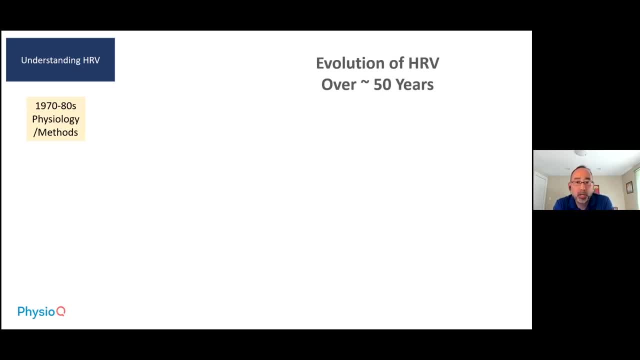 About. you know this occurred about 20 years after Hodgkin and Huxley finalised their axon signal transduction along the squggi axon. this was also 20 years, but still the golden age of hand оперations. So that's the turning point. But then of course t. So the first stage, understanding heart rate variability. 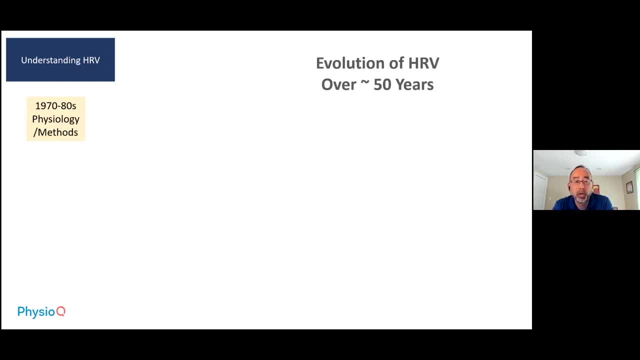 after Watson and Crick figured out the DNA double helix structure and there was enough time for development of imaging stains, such as ELISA in 1971, electrophysiology techniques such as voltage clamps and machines that were important for obtaining electrophysiological measures. 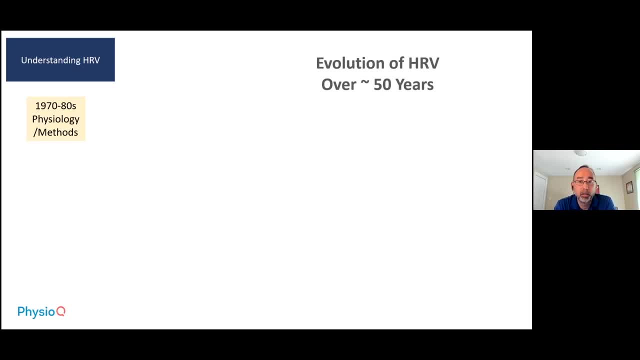 neurotransmitter blockades such as atropine and propranolol, and you also had infrastructure for animal studies, So it is only natural that you would see a significant development or advancement of our physiological understanding of autonomic nervous system around this time. 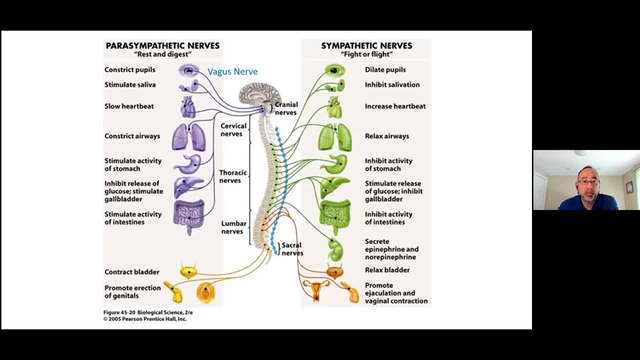 And by this time, by the 1970s, they really had a pretty good understanding of the autonomic nervous system and they have divided into two divisions. Actually there are probably three, because there's the parasympathetic nervous system. 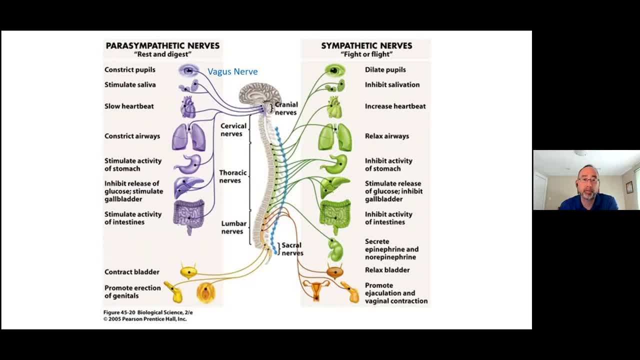 the sympathetic nervous system, and the third one is the enteric nervous system, which we don't talk about too much here, And during the 1970s and 80s. they've very much outlined the various physiological roles that each of these nervous systems play, and also 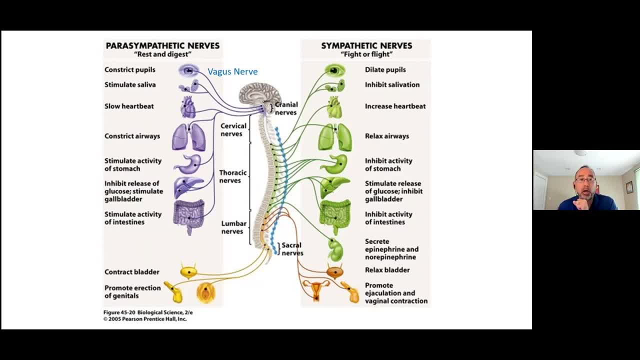 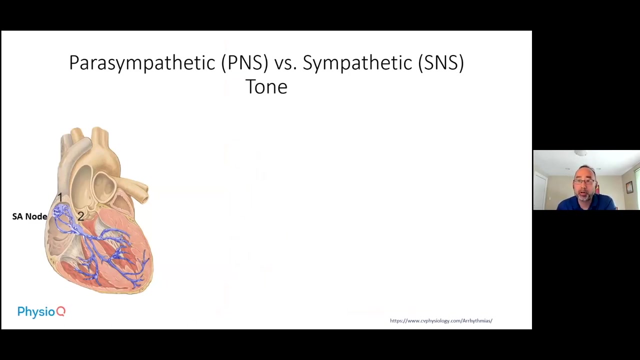 importantly, understood the anatomical pathways that were responsible for the execution and functions of both of these nervous systems. In regards to the heart, we knew that the parasympathetic nerves slows heart rate and the sympathetic nerves increases heart rate. Now the contracting functions of the heart are carried through, are coordinated, basically. 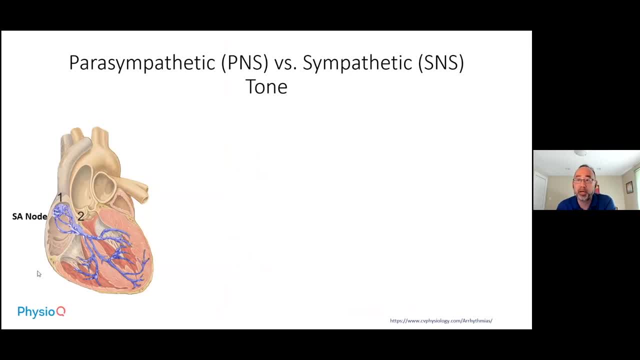 through the electrical conduction system, as depicted here in blue and purple. The part that sets the pace for the heartbeats is the sinoatrial node, or the SA node, located in the right atrium, And it helps set the rate of the heartbeat. The conduction, the electrical conductions: 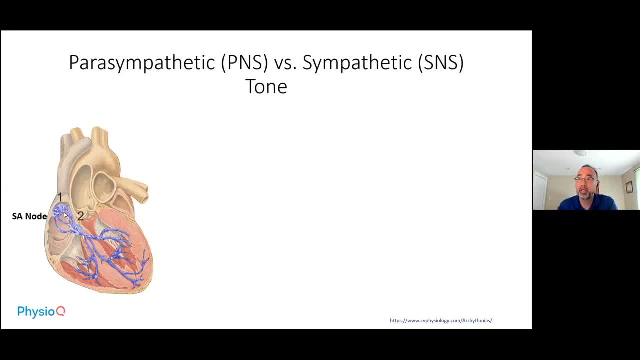 you have essentially pacemaker cells in the SA node, sends electrical signals down the atrium to the AV node and then down the Purkinje's of his, the his Purkinje cells and then down the bundles that led to the contractions of various chambers. And you, both the parasympathetic nerve and the parasympathetic nerve, both the parasympathetic nerve and the parasympathetic nerve, both the parasympathetic nerve and the parasympathetic nerve. 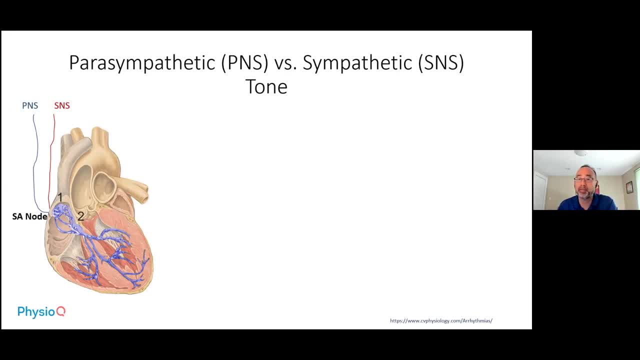 both the parasympathetic nerve. both the parasympathetic nerve and the sympathetic nervous system acts at the SA nodes and helps set the rate of the heartbeat And they both have sort of opposing effects. The sympathetic nervous system increases heart rate, which is shown here, you know. 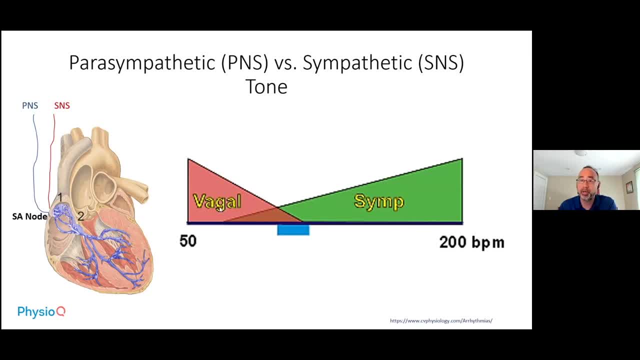 going up to 200 beats per minute. The vagal system, on the other hand, slow, slows heart rate. And if you have exact cancellation of each other and if you let the heart beat intrinsically on its own, it slows heart rate. And if you have exact cancellation of each other and if you let the heart beat intrinsically on its own, 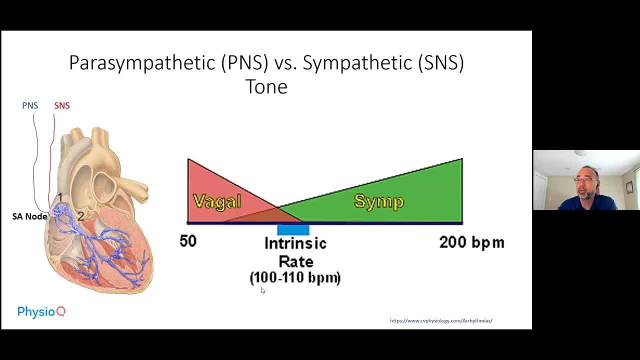 and if you have exact cancellation of each other and if you let the heart beat intrinsically on its own, the intrinsic heart rate is about 110 to 100, about 100 to 110 beats per minute, And since our resting heart rate is around 70 beats per minute, 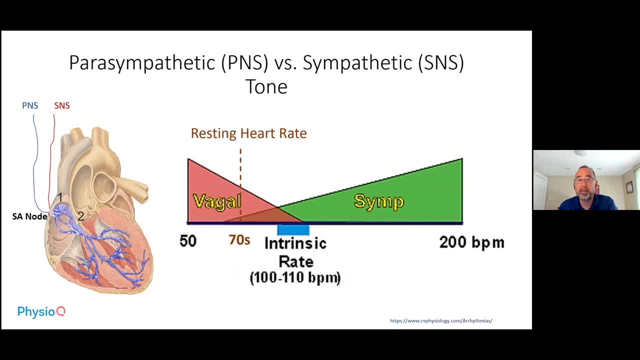 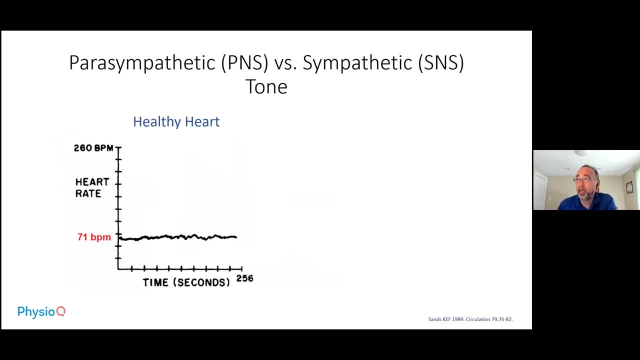 that indicates that the vagal tone is greater than the sympathetic tone at rest. And we knew that actually in the 1970s and even as early as the 1950s actually was because they had done some experimentations with transplanted hearts And you can see here the heart rate. 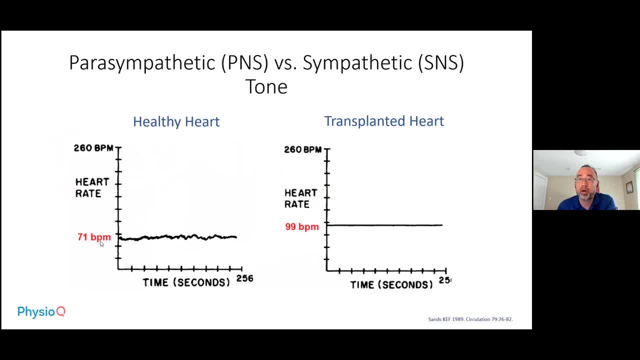 over time in a healthy heart. you can see that the average heart rate is about 71 beats per minute. And then, when they transplanted the heart, either in a dog or in a human, you can see that the heart rate was much higher, about 99 beats per minute. 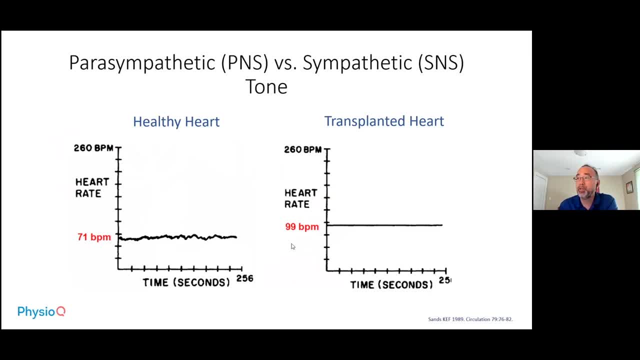 or even higher at 110 beats per minute. And the other thing that you note is that the variability that you see in the heart rate disappears in a transplanted heart, And the reason is that case is because a transplanted heart in order to 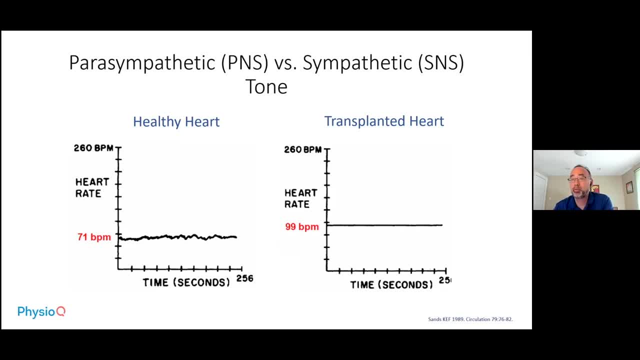 transfer that heart from a donor to the recipient, you need to disconnect all the autonomic nervous connections to that heart, So that includes the parasympathetic nervous system, sympathetic nervous system, And so you lose this variability and you have a significant rise in your heart. 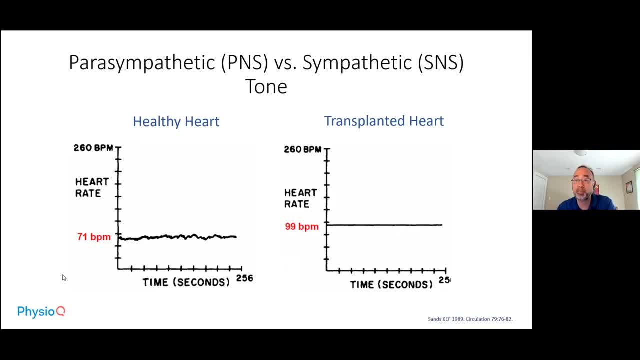 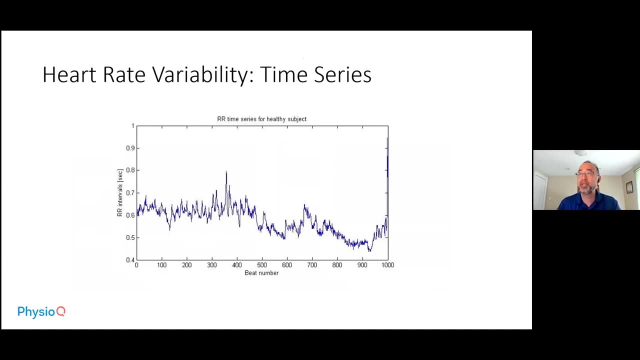 rate And this was known as early as the 1960s because the first human cardiac transplantation was done by Christiane Barner in South Africa in December of 1967. So we knew this way early on And this is an example of sort of the complexity that you get with heart rate variability. 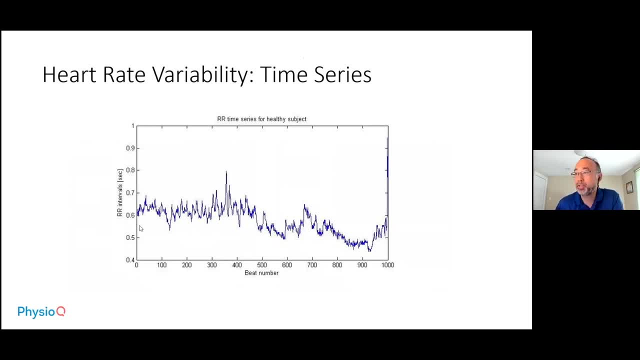 This is RR interval, which is the inverse of heart rate, And you can see the changes in the interval with time or with number of beats, And the average of this graph is the average of the heart rate, And so this is the average of the heart rate, And so this is. 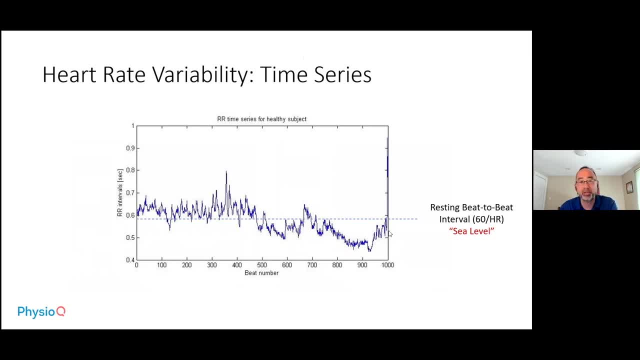 gives you the resting B2B interval or, in the analogy that I would like to say is sort of like the C level, The fluctuations that you can see around. this quote unquote C levels- is the tides and the waves, And this is the heart rate variability that we're talking about. 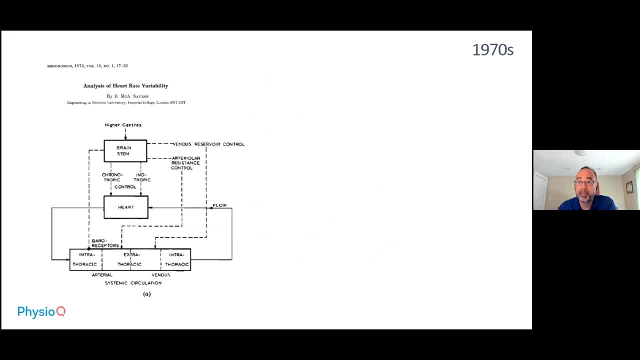 And as early as the 1970s, clearly, physiologists were able to identify the important factors that were involved in heart rate variability and even develop a schematic representation, And this is a pretty good representation And this was a publication in 1973.. They've identified sort of the central neural controls, which included the brainstem. 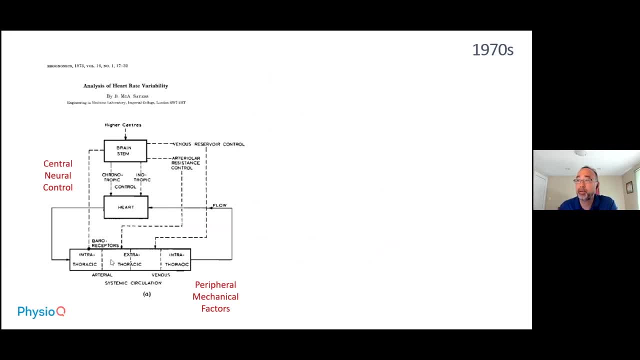 sort of control centers and peripheral mechanical factors, And they even developed a schematic to help understand how these various factors interacted with each other And, as noted, they identified the important factors which included the control centers of the autonomic nervous system in the brainstem. 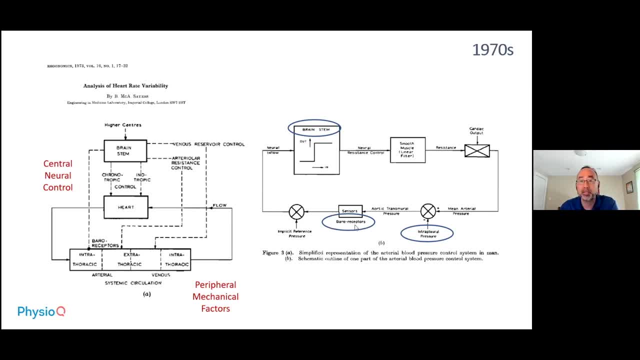 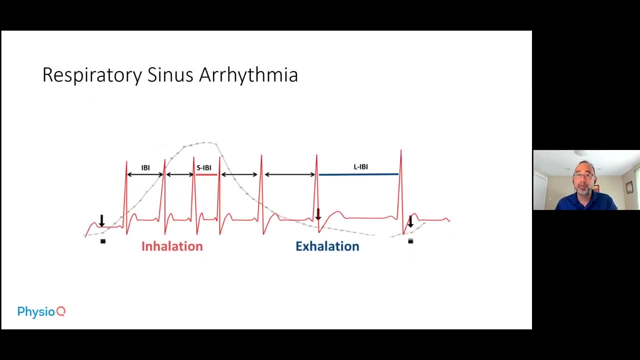 the baroreceptors, which were important for maintaining a stable blood pressure and also the effect of breathing by changing the intrapleural pressures, And so they've clearly developed a very good understanding of this in the 1970s And one of the important parts. 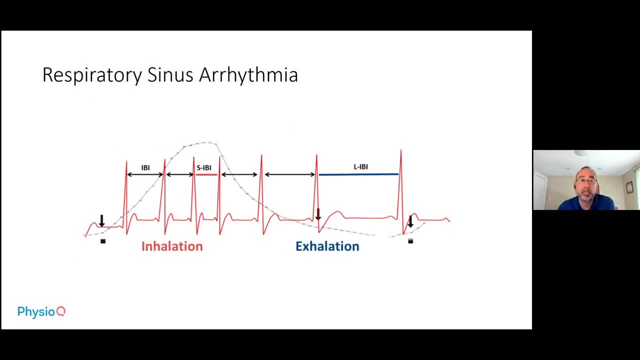 sort of physiological contributions to this. heart rate variability is respiratory sinus arrhythmia. This is the changing your heart rate as you take a breath in and out. And you may notice as you breathe in your heart rate which is sort of illustrated here by the gray increases. 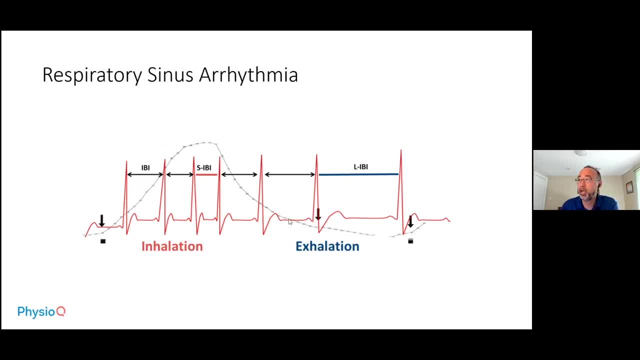 with inspiration or inhalation and it goes down with exhalation And there are certain sort of time, dynamical time parameters or information about this. typical time scales as about every three to seven seconds that you take a breath, or about 9 to 24 cycles per minute. 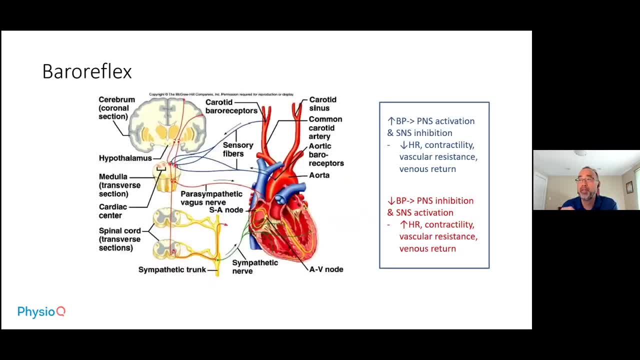 So this is the respiratory sinus arrhythmia, And then the other important physiological factor in heart rate variability is the baroreflex. Baroreflex is a way to control or stabilize blood pressure, And you have essentially these mechanical receptors located in the aorta and the carotid. 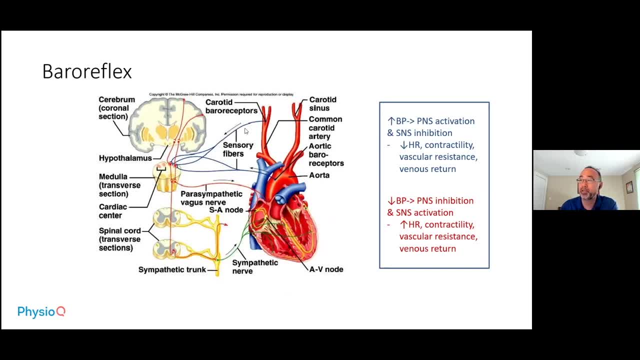 sinus And then through the vagus nerve and the glossopharyngeal nerve you have signals sent to the brainstem And then this brainstem signals then get sent to the autonomic nervous system nuclei, including the parasympathetic and the sympathetic systems. 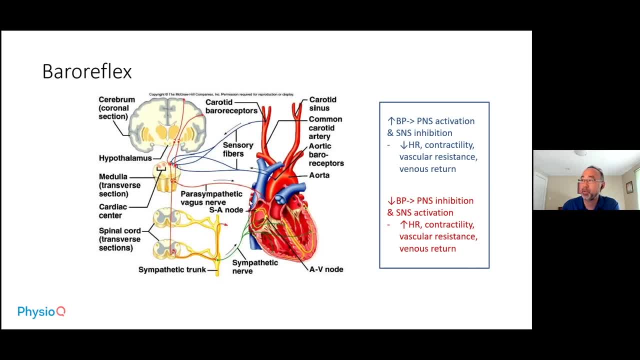 And then they feed back that response, So that affects the SA node and other regions of the heart. The time scale for the baroreflex is a little longer. It's about 3 to 20 seconds and it happens to be greatest approximately about 6 cycles. 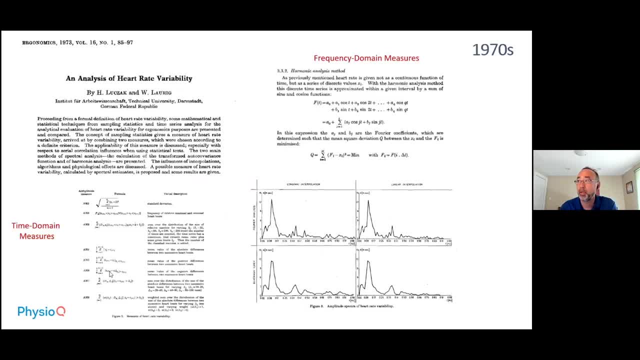 per minute or every 10 seconds, And around this time in the 1970s. in order to capture these variability dynamics, physiologists began to create multiple measures, And it's very hard to see sort of this in sort of granular detail here. 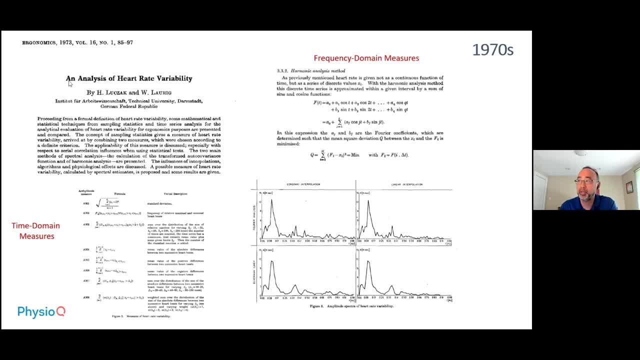 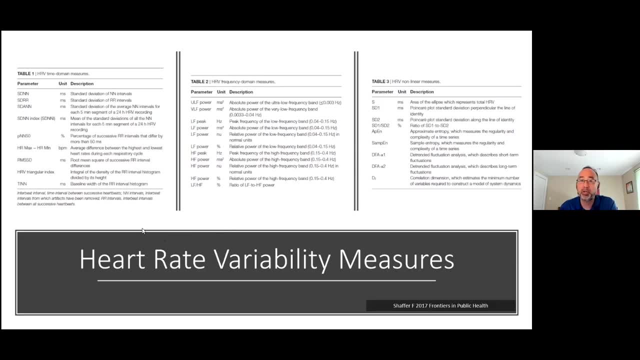 But what's important to note is already by the 1970s they've established important time domain measures, And this is a summation of the multiple heart rate variability measures that are out there in the literature right now. This was in Schaefer in 2017.. These are sort of highlighting the most important ones. There are at least 60 to 70 different heart rate variability measures now And they're categorized into three big buckets. One is heart rate variability by the time domain measures. The second is heart rate variability by the time domain measures. 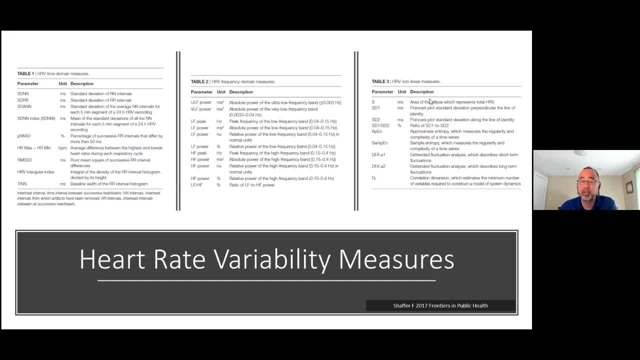 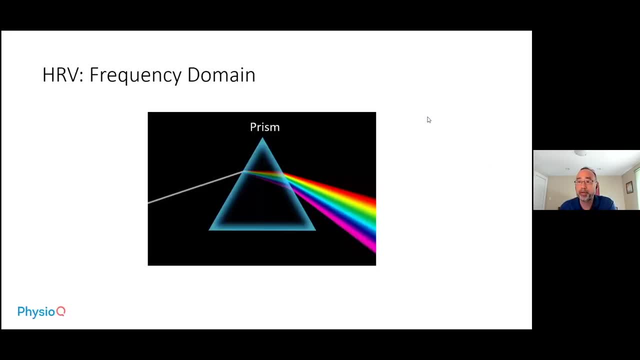 The third one is heart rate variability by frequency domain measures, And the third one is nonlinear measures, And I'm going to talk about each of these in a little more detail. The first one, the first category that I want to talk about, is the frequency domain. 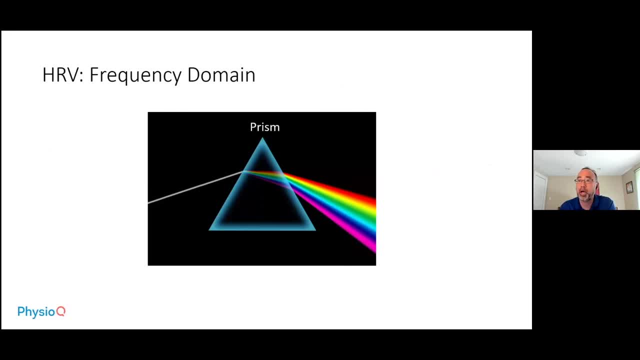 And the way I want to help you understand how this works is to sort of imagine light. So if you take prism and then you shine white light onto it, then the prism actually does breaks down the white light into its different components of spectral light. 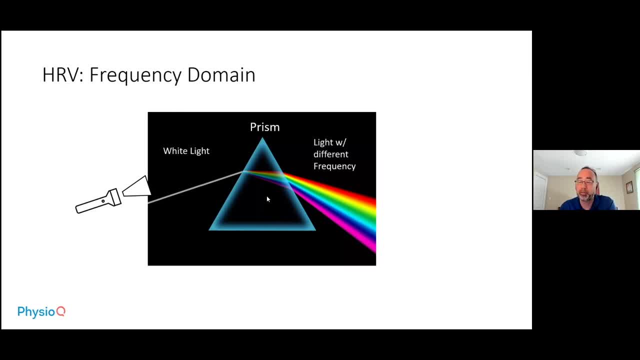 And it's, you know, the prism, based on its ability to sort of. you have different speed of light secondary to the refraction within the prism And, as a result, it divides the light into its different frequencies. And you can imagine that if you had a photo sensor in this wall and you let that photo 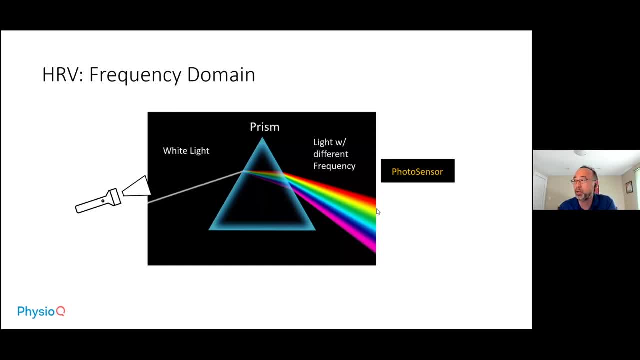 sensor accumulate the amount of light That goes onto that sensor. Over time you will develop an idea of how strong each of these individual components of light are. You could do the same thing with heart rate, time series, And we use different techniques and sort of analogous to the prism. 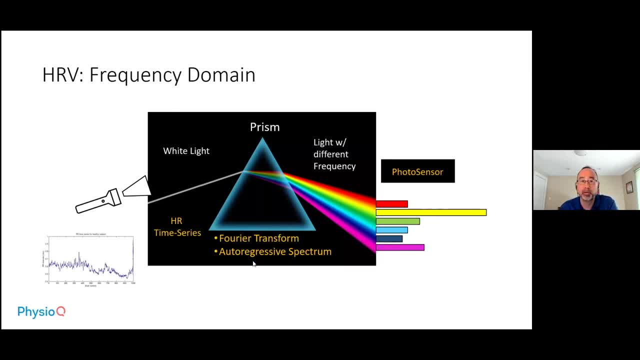 You have something called Fourier, transform and autoregressive spectrum analysis. There are some others as well, And what these techniques do is that, Okay, It permits us to identify the spectral firepower, each frequency range. so you can imagine this: heart rate variability is composed of multiple signals with different frequencies. 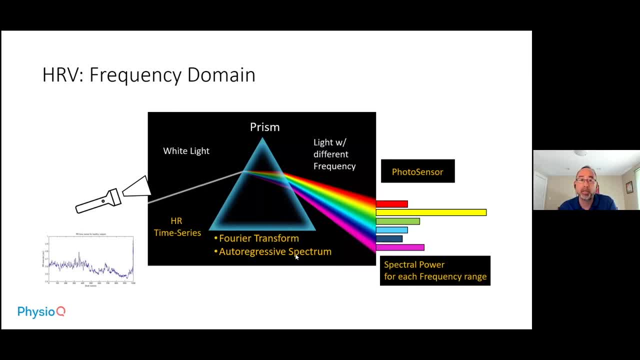 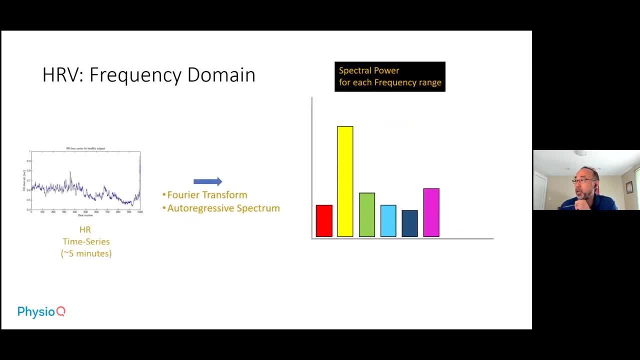 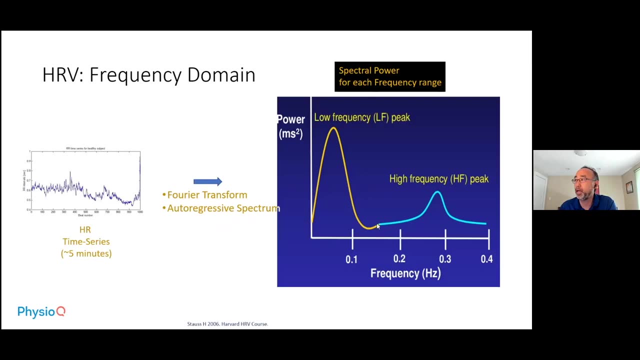 And these techniques enables us to sort of divide them into identify which component is the strongest. And what you see here is you can essentially produce a spectral power And you can see that the spectral power is divided um according to the frequency. The frequency: the higher it is, that means the faster the cycle. 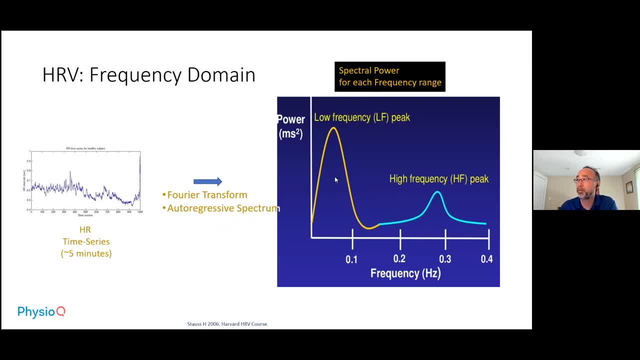 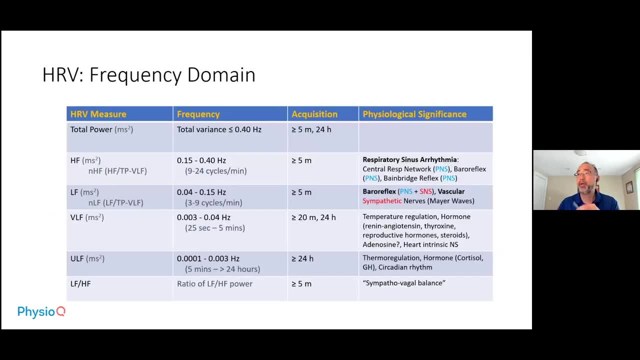 So the higher frequency is on the right here and the lower frequency is on the left, And over time they have we've got a pretty good understanding of the various categories of the cycles of the frequencies that are involved in heart rate variability, and we've 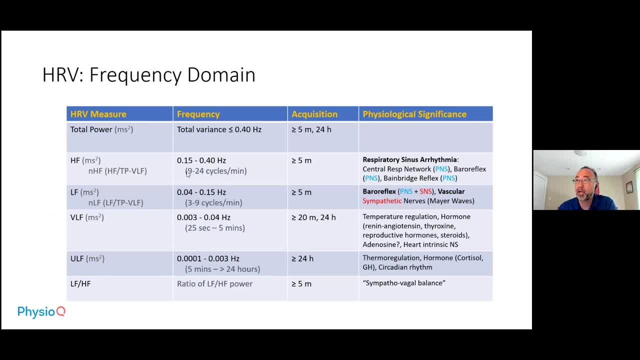 divided them into several categories. There's high frequency, low frequency, very low frequency and ultra low frequency, And then we have a ratio of lower frequency versus higher high frequencies, and the frequencies that are associated with each of these frequency ranges are listed here. 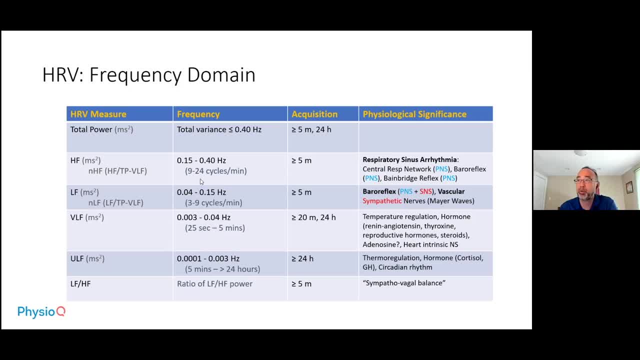 The ones that I want to have you pay attention to is the high frequency and the low frequency. So high frequency is 0.15 to 0.4 hertz, which is about nine to 24 cycles per minute. Uh, low frequency is three to nine cycles per minute. 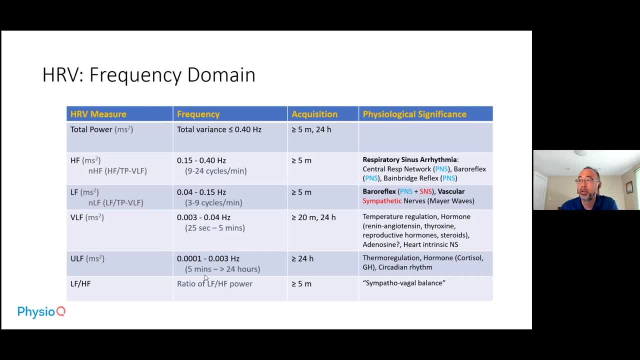 Very low frequency is 25 seconds to five minutes per cycle, five minutes to 24 hours for the ultra low frequencies per cycle. And in order to evaluate these cycles you would need to acquire the heart rate over time. And because these cycles are shorter- uh, high frequency, low frequency oftentimes. 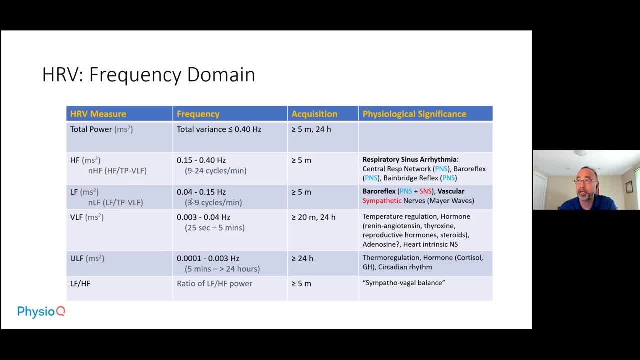 you just need five minutes in order to get information about these cycles, Whereas for longer um cycles you would definitely need to require as as long as 24 hours. And each of these cycles are associated with have have the physiological significance. 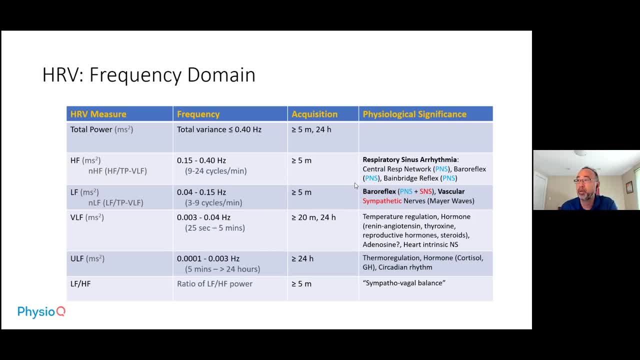 So high frequency is associated with respiratory sinus arrhythmia. The low frequency is associated with baroreflex intravascular sympathetic nerves, um, and there's something called mayor waves, which is the oscillations, the intrinsic oscillations that you see in the vessels, um, when I'm talking about the arteries, 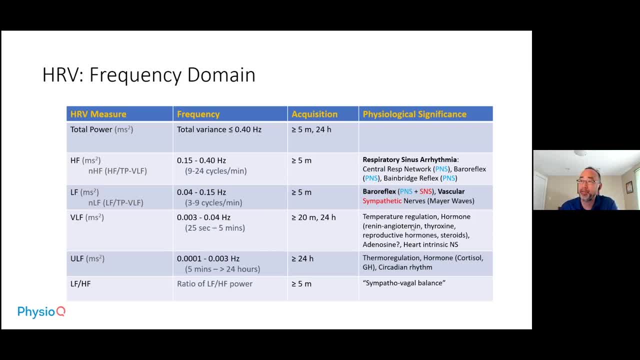 Okay, Now, when we think about the arteries, where they're centered the arteries are? they're located in the heart. The heart is the center of the nervous system. It's at the heart that the heart is, And the heart is the central nervous system. 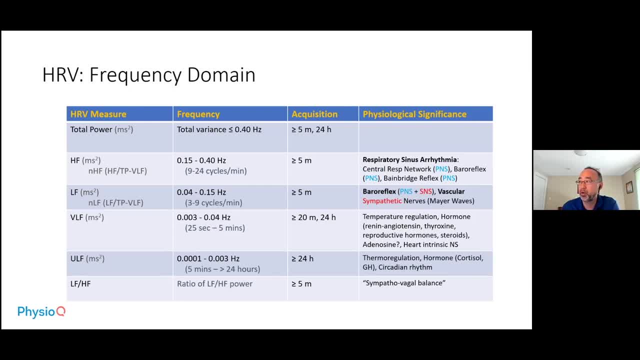 Very low frequencies have slower um physiological systems involved, such as temperature regulation hormones such as re engine tension, thyroxine, reproductive hormones and steroids. And then the heart has an intrinsic nervous system as well, which is believed to have a very low frequency range. 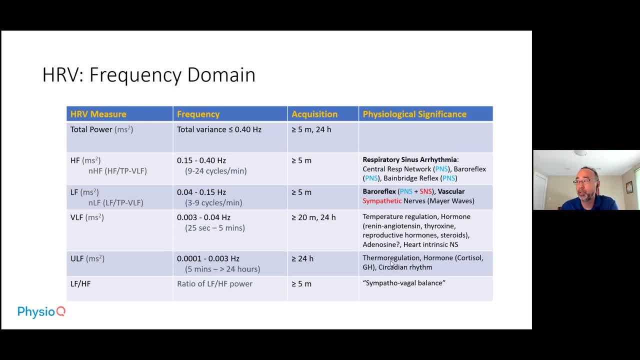 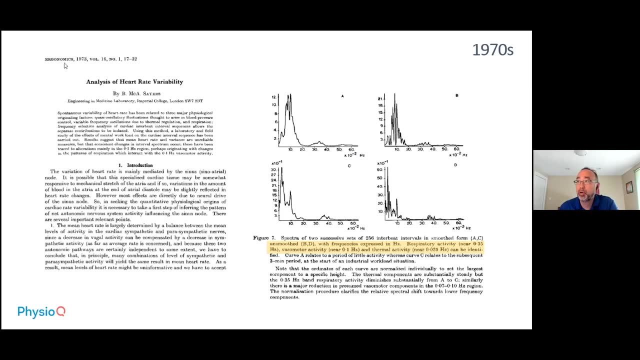 And then at the ultra low frequency range. it involves thermoregulation, other hormones such as cortisol and growth hormones and the circadian rhythm, and they knew a lot of this as early as the 1970s, and this is a publication in ergonomics. 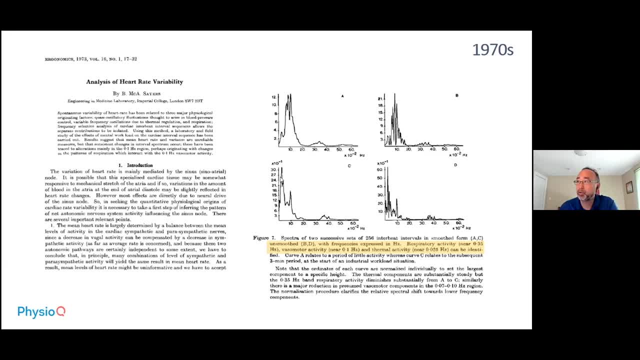 and again. they have sort of created this frequency spectral analysis of heart rate variability, and I'm going to read this to you because it may be small on your screen, but they have already noticed that the respiratory activity is largely, predominantly, near 0.35 hertz. 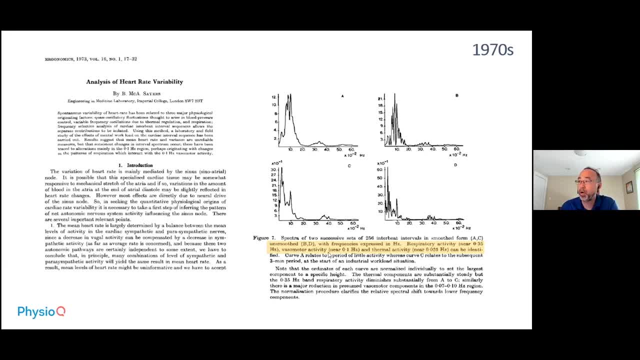 which falls into our high frequency range. The vasomotor activity lies in the 0.1 hertz, which lies in the low frequency range, and thermal activity at 0.025 hertz, which is in the very low frequency range. so already they knew this in the 1970s. 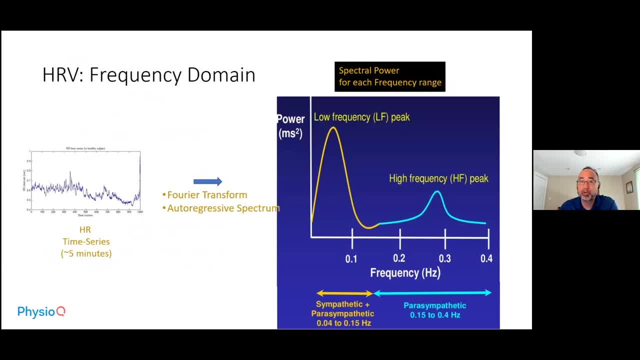 and one thing that you'll come to realize is that the high frequency of the spectral power of heart rate variability is very low, and that's because the heart rate variability is very low and so is associated with the parasympathetic system, whereas the low frequency is associated with 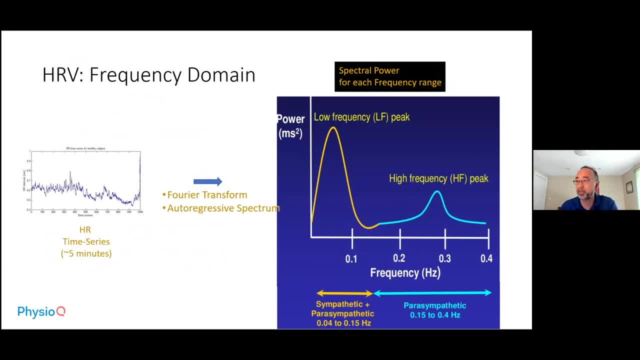 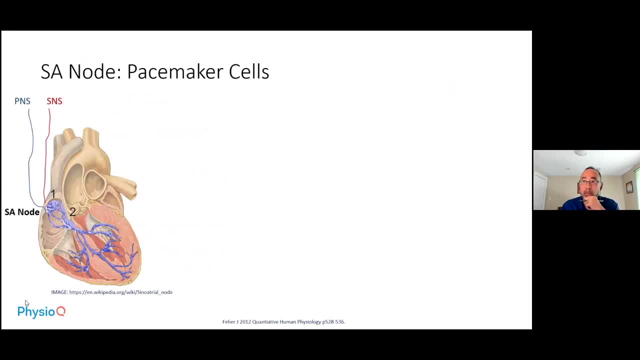 both the parasympathetic and the sympathetic nervous system- and I'm going to explain to you why that is So- in the SA node, which is, as we know, the pacemaker. oh, sorry, a little lag. okay, there are four important ion channels. 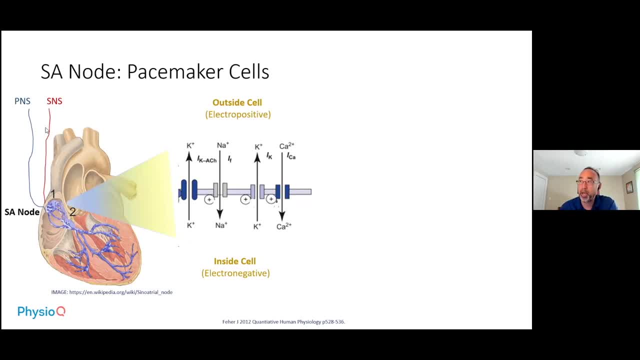 on the SA node cell membranes You have the sodium channel, potassium channel- actually two potassium channels and a calcium channel- and within the cell it is electrically negative relative to the outside of the cell, and so there's a 65 millivolt difference. 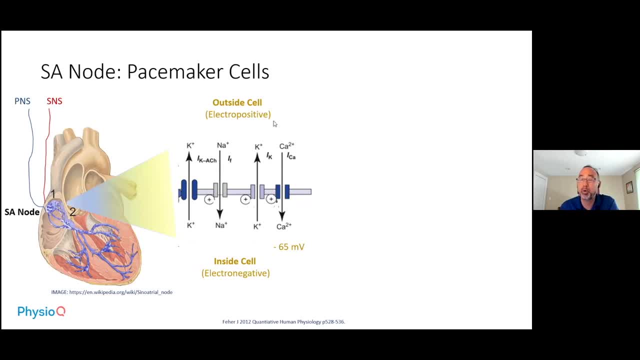 so that the inside is 65 millivolts lower than the outside of the cell. So when you have positive ions move across the cell membranes through the ion channels, it neutralizes or decreases this electrical potential difference. and so what you say, what we say, is that it depolarizes. 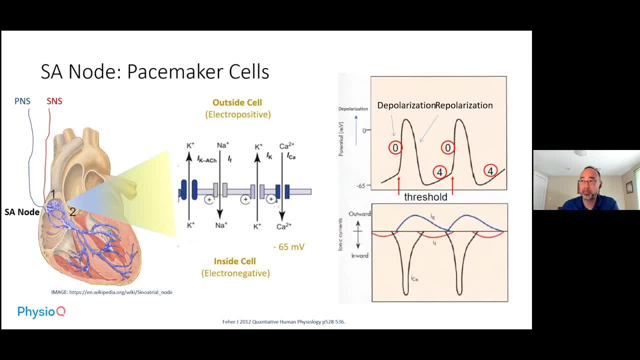 the cell membrane or the cell. On the other hand, if you have potassium channels, which goes in the opposite direction, it enhances this polarization or it repolarizes or hyperpolarizes the cell membrane, And this is sort of a diagram to illustrate this. So you have 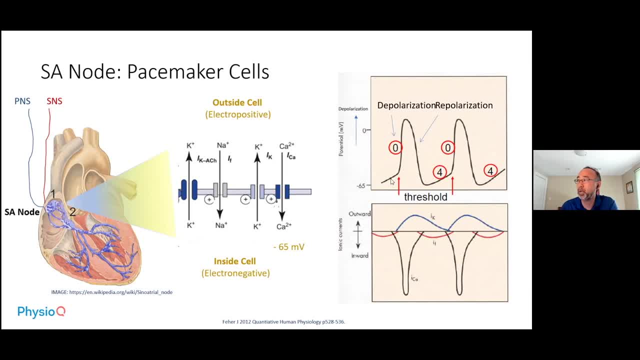 a measurement of the voltage potential difference across the cell membrane and as it goes up, you know, from negative 65 millivolts to zero and even positive potential difference. it's depolarization and as it goes down, it's repolarization. 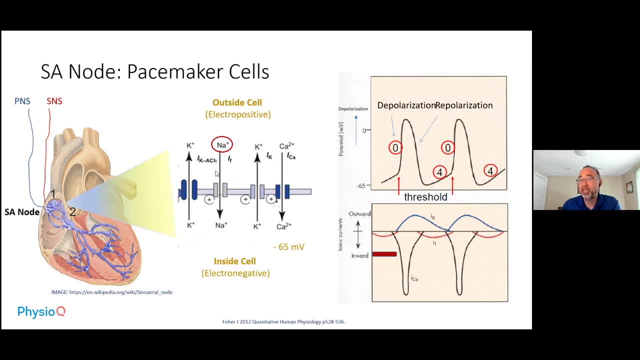 The sodium channel has what's called a leaky current, and this leaky current will cause it to depolarize. It causes a depolarization, a very slow depolarization, of the cell membrane, And what happens is that slowly as it reaches a threshold, as denoted by this dashed line here. 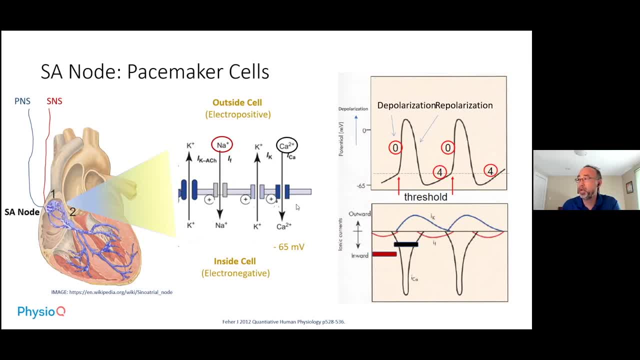 it causes the calcium channel to open up and this causes a rush of calcium channels into the cell and then actively leads to depolarization of the SA node cells. Subsequently, the potassium channels open up and then it leads reverses this polarization, this depolarization. 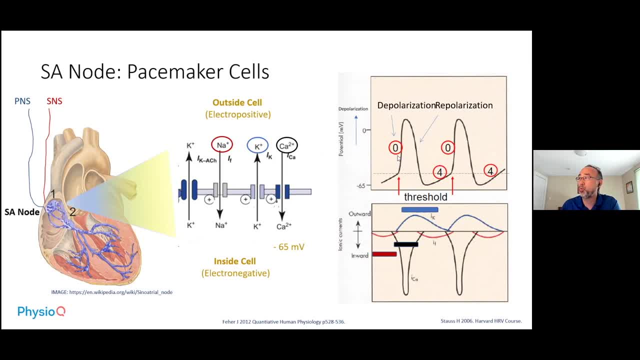 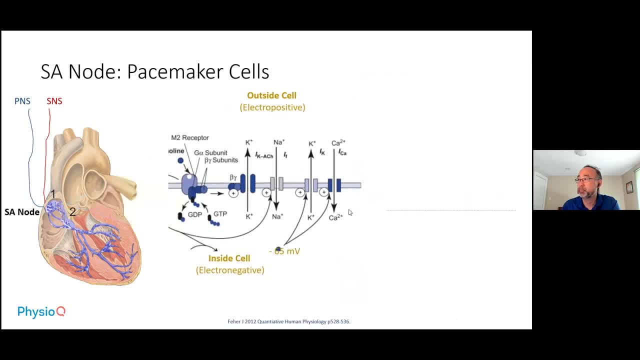 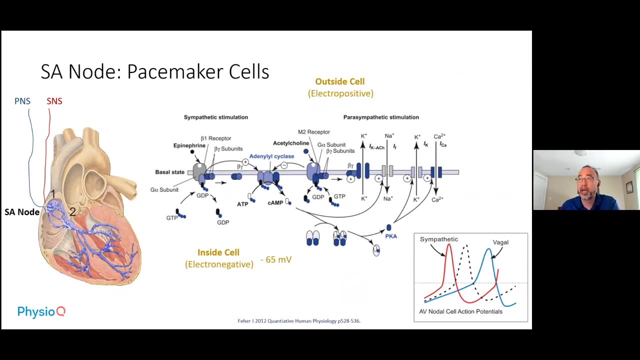 that is caused by both the sodium and calcium channels, and you get repolarization, as denoted by this downslope of this potential difference. Now, taking this within the context of the autonomic nervous system, you could see how the autonomic system affects this pacemaking ability of the cell. 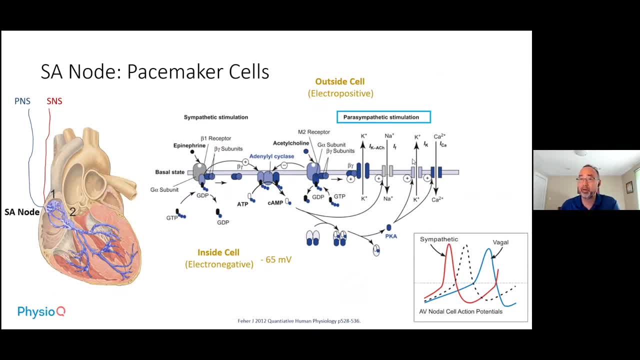 So the parasympathetic nervous system involves the acetylcholine coming from the postganglion of the parasympathetic nervous system, binding to the M2 of the muscarinic receptor, activating the G protein which then subsequently activates this potassium-associated acetylcholine. 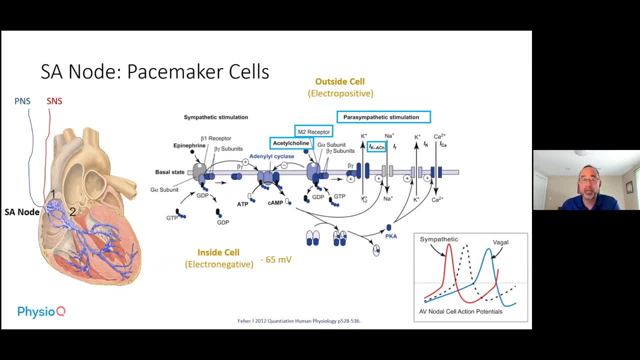 channel And because this is a potassium channel that goes in the direction that enhances the polarization. what it does is that, during this stage of this slow leak of this sodium channel, it leads to this very slow rise of the depolarization. Now this is in the dashed line. 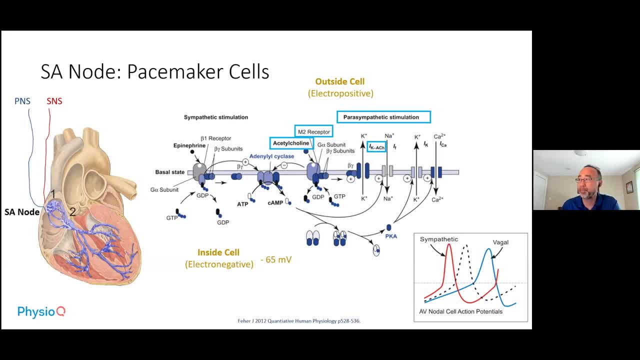 is what is considered a normal heart rhythm. So if there was no intervention from either the sympathetic or the vagal system or the parasympathetic system, you would have this type of automaticity of the electrical potential. So the parasympathetic nervous system might have this. 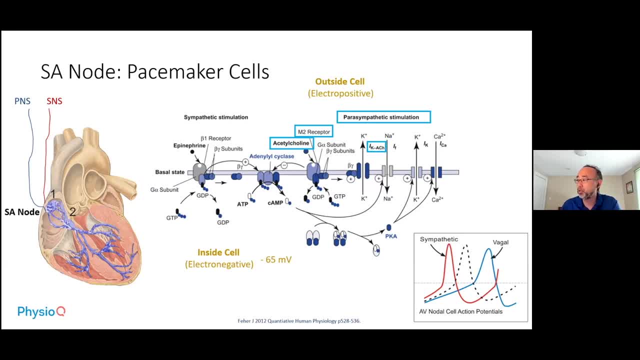 automaticity of the electrical potential. So the parasympathetic nervous system would go through this, but with the vagal nerve it slows this depolization and subsequently leads to a slower heart rate. Essentially, you're not having firing of these cells happening more frequently. 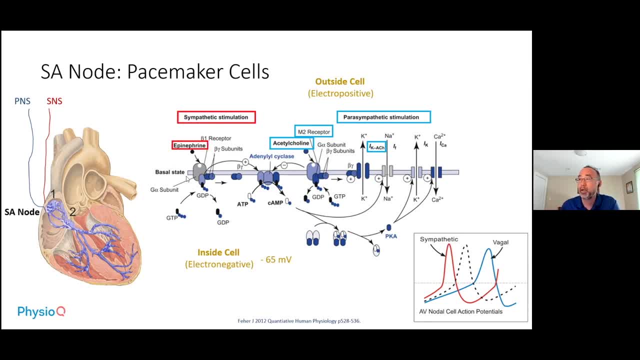 The sympathetic nervous system, on the other hand, operates through norepinephrine or epinephrine that binds to the beta-1 receptors. The beta-1 receptors then bind to adenylal cyclase, which converts ATP to cyclic AMP. The cyclic AMP hastens or enhances this leaky current. 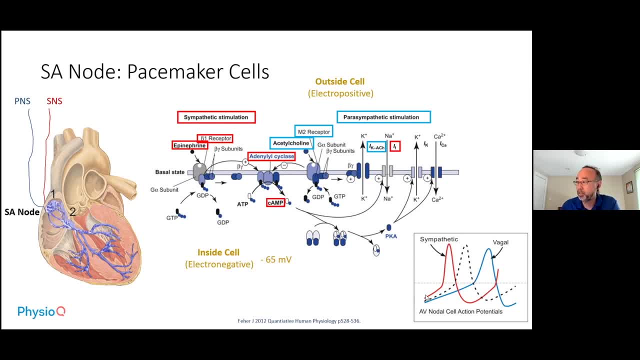 in the sodium channel. This leads to a rise of this depolarization, this steady leak, and then leads to a faster polarization or a faster heart rate. The other thing that it does is that the cyclic AMP activates protein kinase A, then activates potassium channels and calcium. 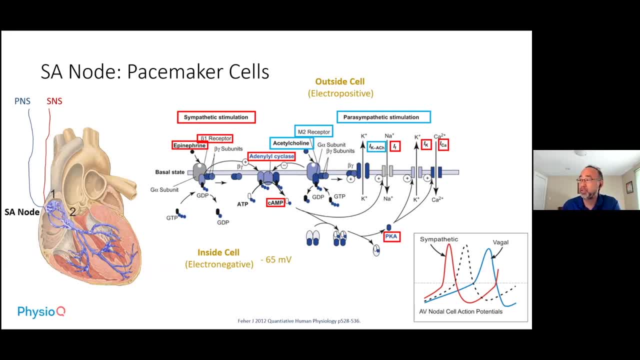 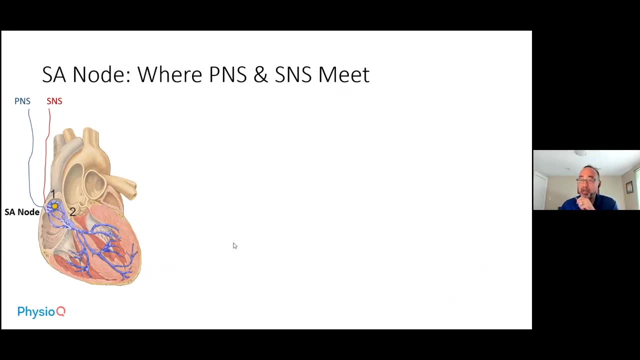 channels. What it does is it increases the fast depolization and fast repolization, so it enables a faster beating of the heart. Why am I harping on this and why am I bothering you with all these details? Because it's really important to know this physiology, to understand what you're seeing when you're. 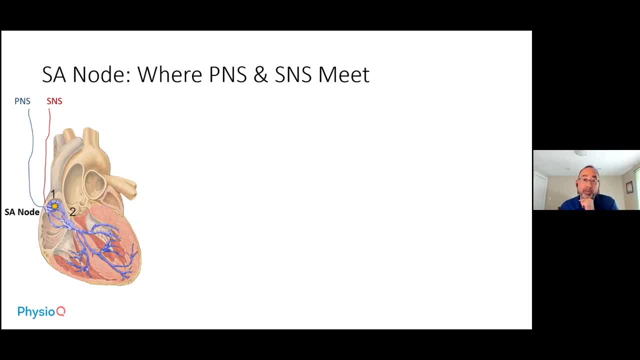 obtaining the heart rhythms that you get from your various devices. The SA node is, as you can see, where both the parasympathetic nervous system and the sympathetic nervous system meet. We can gain insights in the activities of the autonomic nervous system based on the heart. 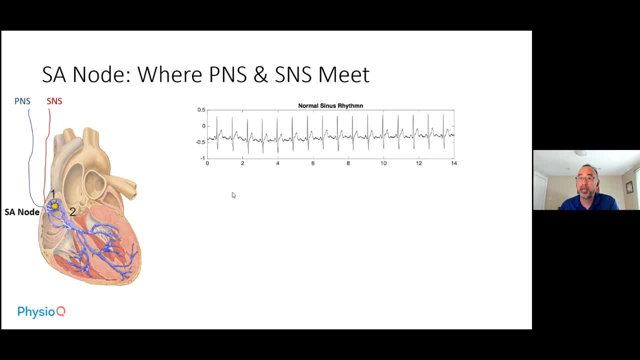 rate over time. What we look at is the interbeat interval interval or the RR interval. This is an example of an EKG of a normal sinus rhythm. We designate the RR interval, so R indicates the peak of this QRS segment, and then we identify the RR interval, the time between these intervals, and then 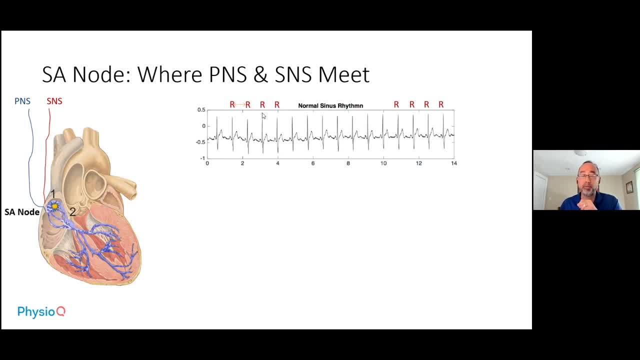 we can obtain a calculation, a graph- which I've shown before- of the RR interval over time, to get a better sense of what is happening with the parasympathetic and sympathetic nervous system. What happens, though, if you have a? 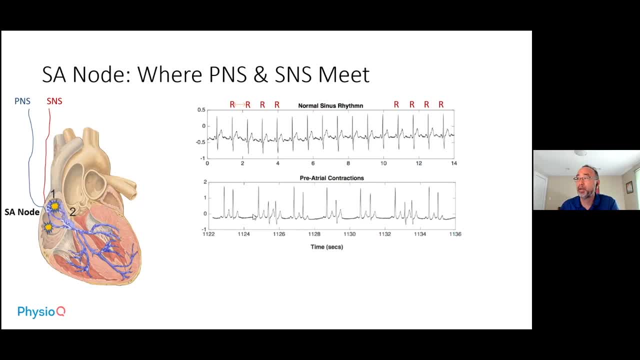 Right, okay. So what happens, however, when you have pre-atrial contractions, where you have contractions that's happening at not only the SC nodes but also in the other parts, ectopic sites, of the right atrium? You would see that the 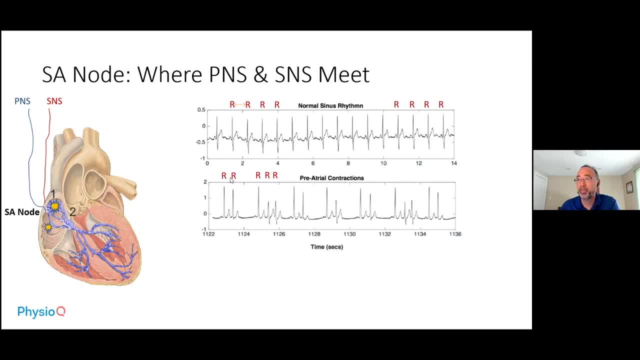 RR is designated here, but does the RR interval actually provide any information about the autonomic nervous system And what happens if you have something called atrial fibrillation, where you have multiple ectopic sites throughout the right atrium and sometimes the left atrium? 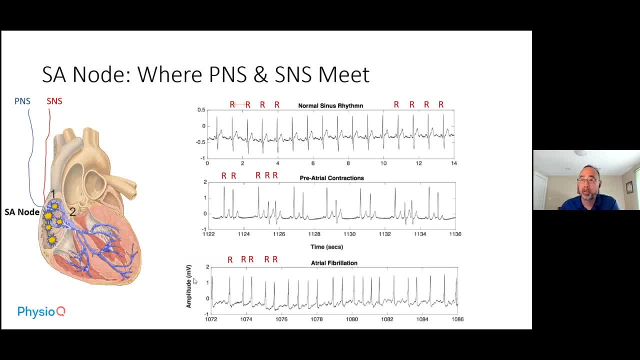 that leads to this erratic part rhythm, And what we recognize is that, because a lot of these extra nodes occur outside the SC node, we consider them as noise and not reflective of what's happening in the autonomic nervous system. So the important thing to note is that heartbeats originating from the SC node are the only ones. 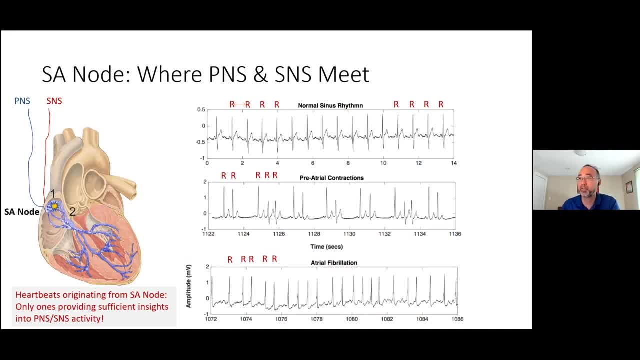 that provide sufficient insights into the parasympathetic nervous system and sympathetic nervous system And to delineate what are sort of the normal rhythms. through the SC nodes we change R into Ns or normal rhythms And the way we know on an EKG whether it's a normal rhythm or not. 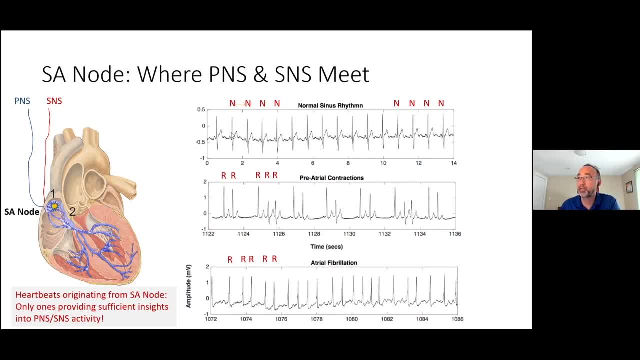 is. we know that the heartbeats originating from the SC node are the only ones that provide sufficient insights into the parasympathetic nervous system, And we can see something called a P wave. before this QRS, You can see these P waves And these P waves are the electrical contractions or electrical signals. 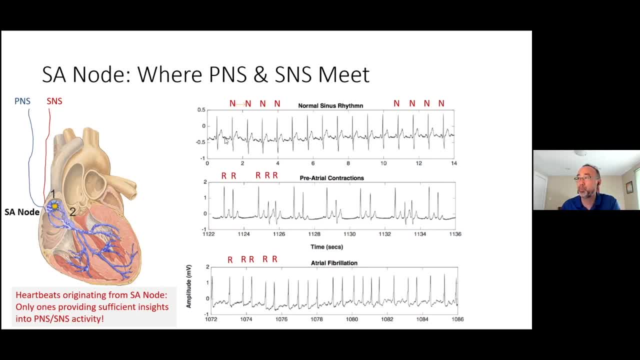 going through the right atrium And we know through the axis or the morphology how it's shaped, that it's going through the right system. In the preatrial contractions we notice that the normal sinus rhythms are occurring here because we see the P waves here. We don't necessarily 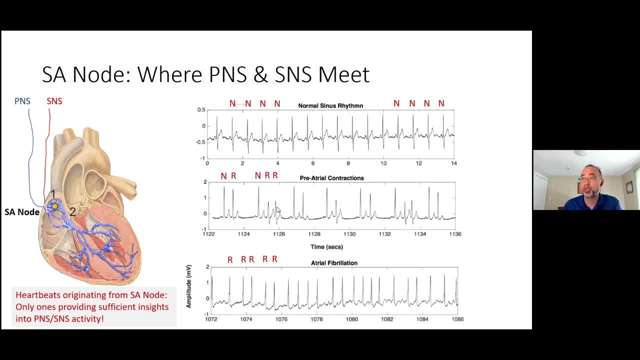 see the P waves that occur before these preatrial contractions And, as a result, we eliminate these R waves. And sometimes what we do is we interpolate the N between the normal ones to get an idea of what the SC node would have done if it hadn't been for these ectopic. 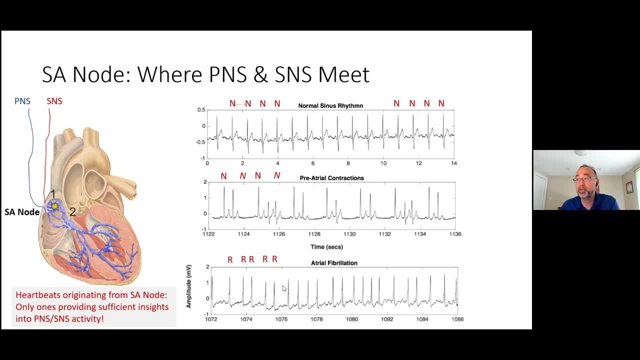 beats. Preatrial fibrillation, on the other hand, is so inundated by all these signals that are coming from these other parts of the right atrium that we can't get enough information in the SC node. So we can't really get much information. 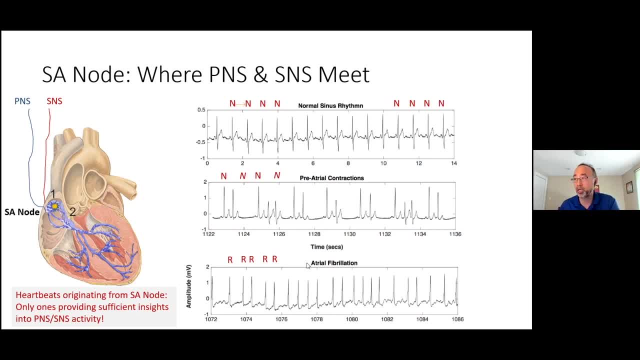 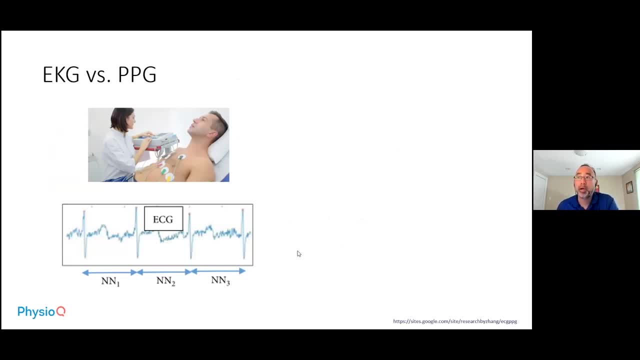 In patients with atrial fibrillations about their autonomic nervous system. So this is something that you can get from your EKG. However, in many of you, we're getting heart rhythms from use of watches, And the watches don't use, you know, obtain EKGs. What we obtain. 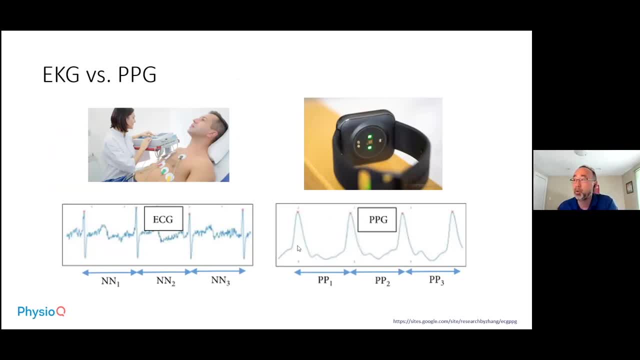 are the PPGs or the photoplethysmography, which measures the flow through the microvasculature in your skin, And it has. you know, it doesn't have this rapid upstroke that you can see in the electropolization. It's a slow rise, And the other thing to know is that you can't tell whether these 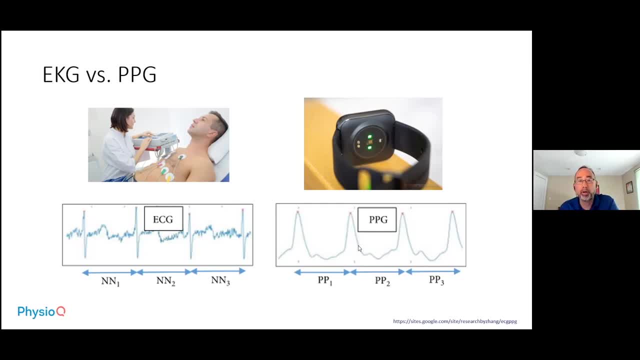 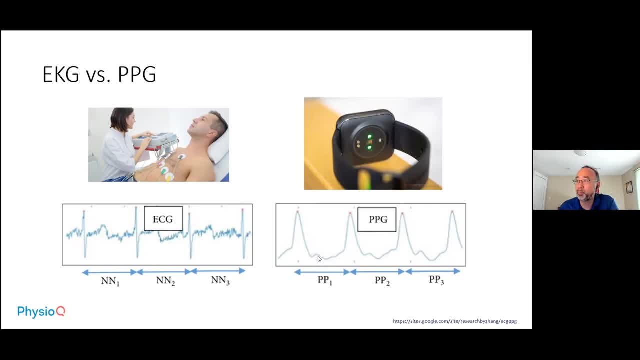 It is a reflective pulse wave, So it's not a P wave. So this is one of the challenges that you may encounter as you do your research- is that the PPGs won't give you information about what or directly won't give you information about what kind of rhythm you have. 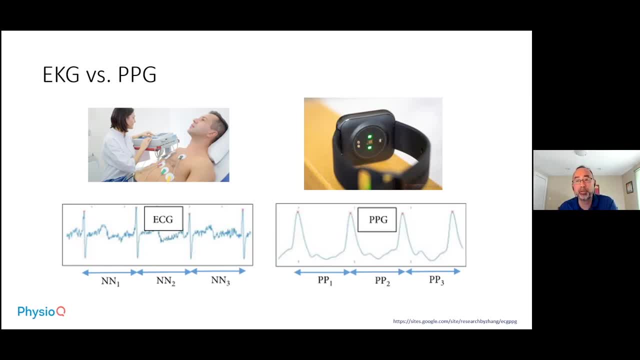 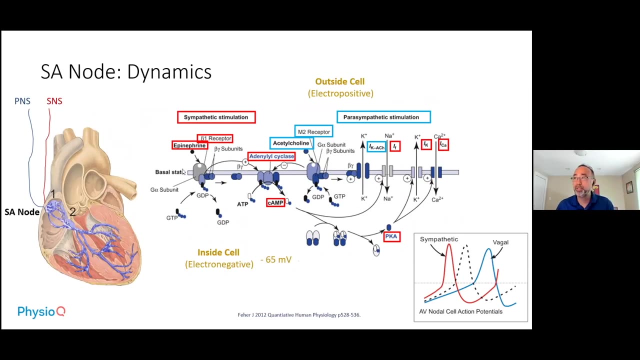 And sometimes if someone has a lot of ectopic atrial beats or atrial fibrillation, it falsely gives you a higher heart rate variability And it doesn't give you a reflection of your autonomic nervous system. The next thing I wanted to the reason that this diagram is really important is to really give you an 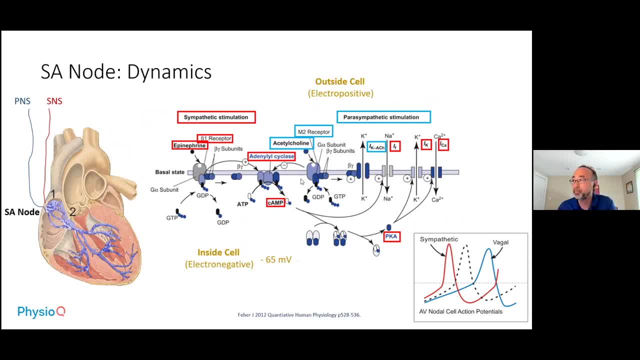 understanding of the dynamics of the SA node. In the SA nodes the acetylcholine receptor operates very quickly. So the acetylcholine, after it binds to the M2 receptor, the G protein, acts literally in few milliseconds to activate this potassium ion channel. 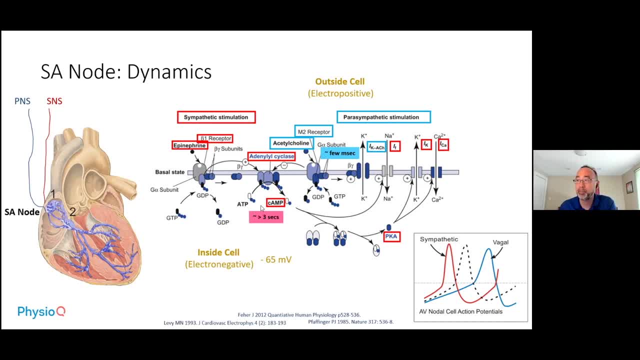 On the other hand, the sympathetic nervous system it has to it's intubated through this enzyme called etanolyl cyclase, And this cyclase operates at much slower timescales- approximately three seconds or more- And as a result, it is much slower to respond. 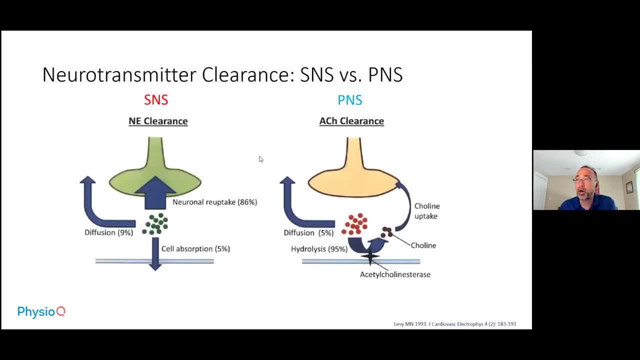 The other thing to note is that there are different dynamics in the neurotransmitters associated with each of these autonomic systems. The other thing to note is that there are different dynamics in the neurotransmitters associated with each of these autonomic systems. The other thing to note is that there are different dynamics in the neurotransmitters associated with each of these autonomic systems. 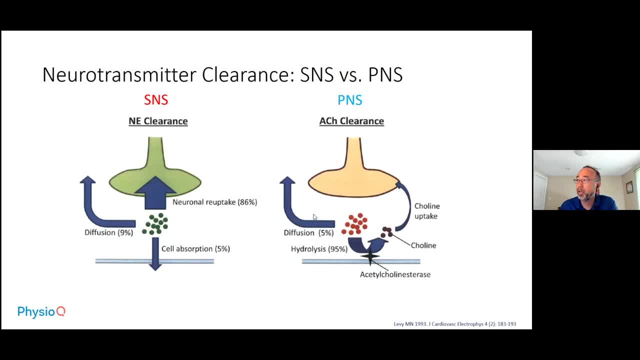 The parasympathetic nervous system utilizes acetylcholine and the sympathetic nervous system utilizes norepinephrine or epinephrine And the acetylcholine when it's released from this bulb of the preganglionic neuron. 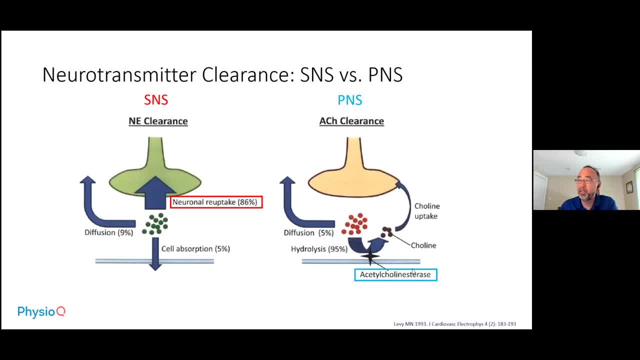 it is quickly eliminated by abundant presence of acetylcholinesterase within the gap junction. On the other hand, the sympathetic nervous system has to- not has to- uptake these norepinephrine within the gap junctions, And the timescales are much different. 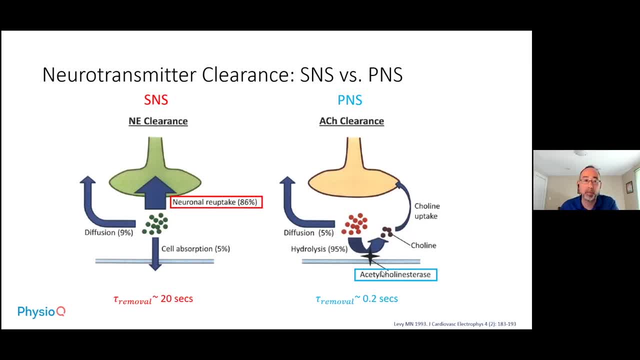 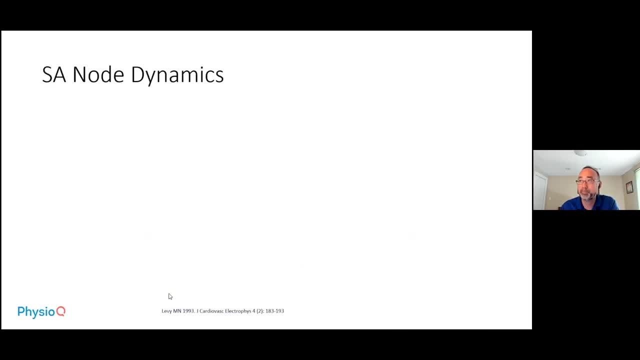 So the parasympathetic nervous system removes these things about every you know point two seconds, whereas the sympathetic nervous system removes it in 20 seconds. And what this leads to is a very different, is a very different dynamic for each of these branches of the nervous system. 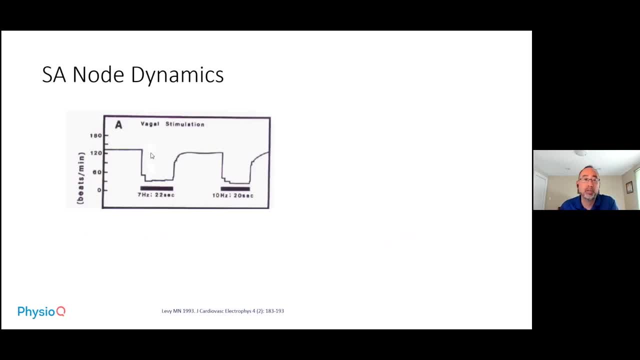 For the parasympathetic nervous system. they've done this in dogs. they've stimulated the vagal nerve and you can see the stimulation right here. They essentially give seven hertz electrical stimulation for about 22 seconds And right away you can see that the beats per minute or the heart rate significantly decreases. 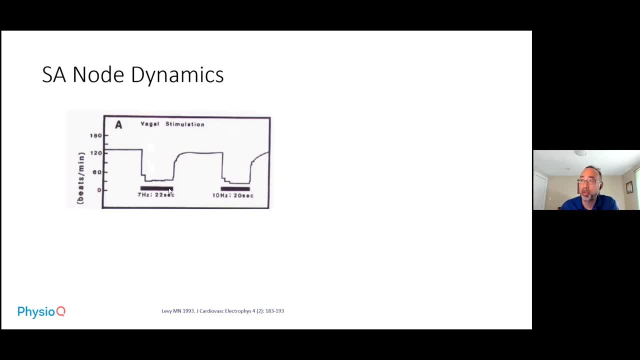 And almost immediately after you initiate the stimulation and the moment it stops, you stop the stimulation, the heart rate jumps back up nearly close to its original heart rate rhythm, And the same after you do this, And so the parasympathetic has a rapid onset, quick execution and a short recovery time. 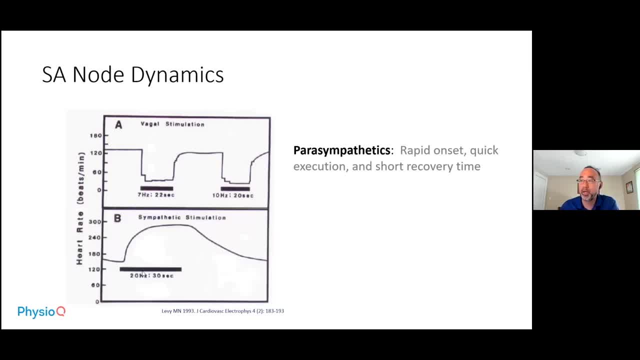 The sympathetic nervous system. on the other hand, when you're delivering 20 hertz stimulation to the sympathetic nerve and take a look at the heart rhythm, you can see that it doesn't kick in right away. There is a little bit of a lag, about seven seconds or so. 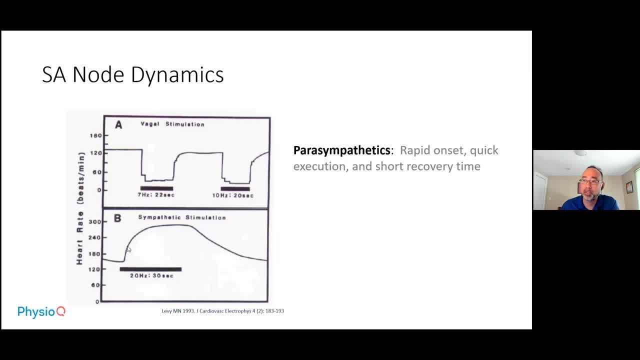 from the initiation of electrostimulation and then the rise of the heart rate. And this rise in the heart rate is not immediate, like you see in the vagal system, but it's very slow. And after you stop this stimulation there is also a lag and it's a very slow recovery time. 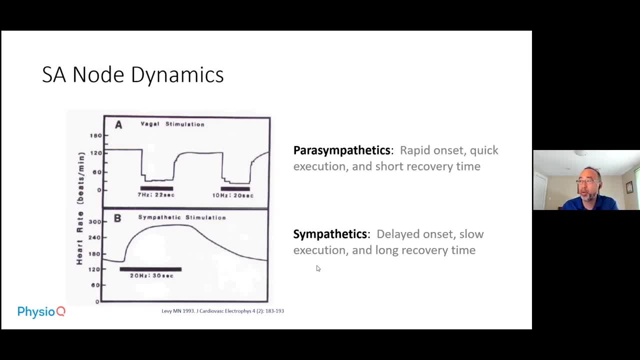 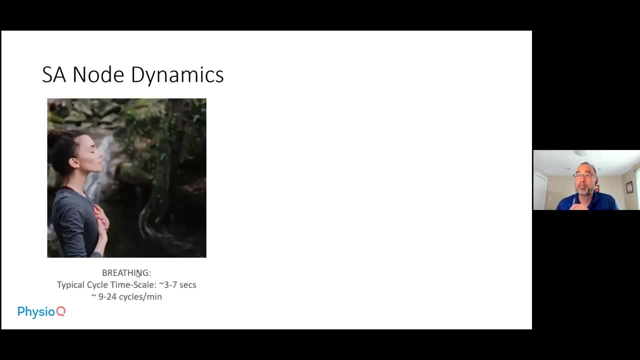 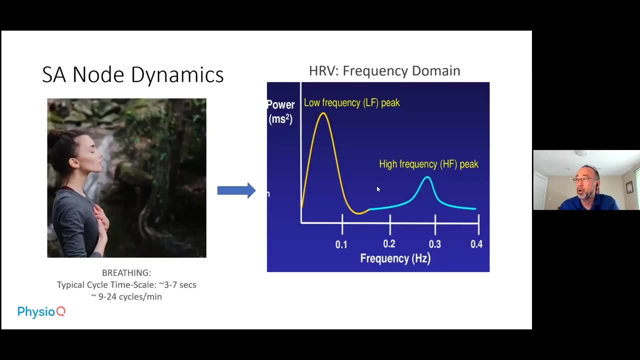 So the sympathetic has a delayed onset, slow execution and a long recovery time. So what does this mean? Is that when we're breathing, and are breathing every three to seven seconds or nine to 24 cycles per minute, we're operating in the high frequency range? 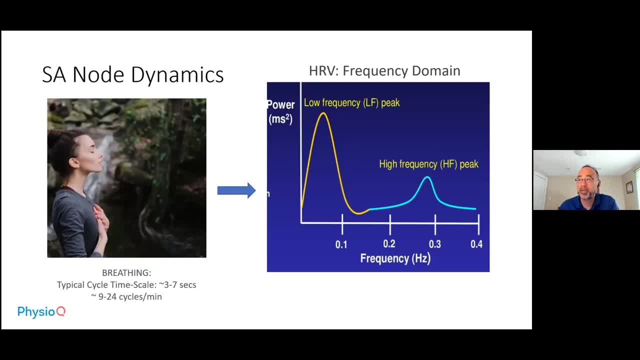 And, as noted, parasympathetic nervous system is the only one that really is able to operate in the higher frequency range. due to this dynamics- Quick onset, quick execution, rapid execution, rapid recovery time- whereas the sympathetic nervous system is simply too slow. 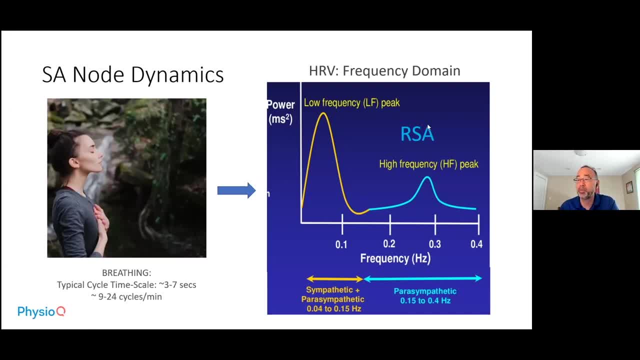 So when you have something like respiratory sinus arrhythmias, the changes in your heart rate- with respirations it's predominantly slow. So when you have something like respiratory sinus arrhythmias, the changes in your heart rate, with respirations it's predominantly slow. 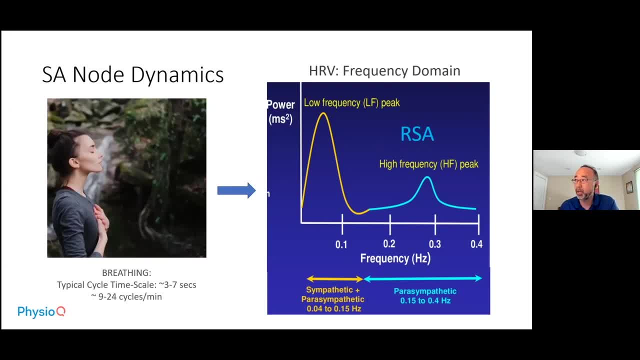 So when you have something like respiratory sinus arrhythmias- the changes in your heart rate with respirations- it's predominantly a parasympathetic phenomenon And it's simply due to the fact that the SA node has a filter which inhibits the sympathetic nervous system to operate at a faster frequency. 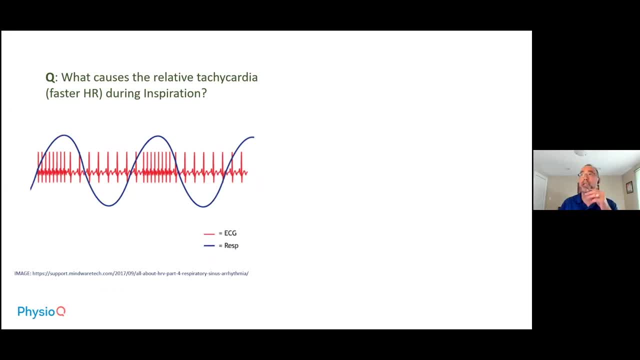 So the question for you is: what causes relative tachycardia during expiration then? So we know that if you breathe in, you have rising heart rate. If you breathe out, you have a decrease in your heart rate. So if it's not, because I had heard on a podcast someone saying that as you breathe in, you entail, this directly, stimulates the sympathetic nervous system, and this is how you get a rise in your heart rate. 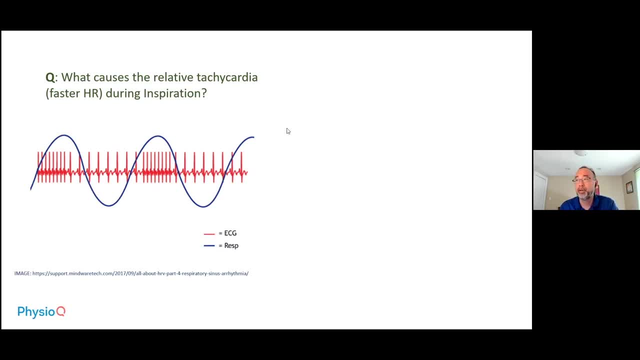 We know that's not true, based on our understanding of physiology. In fact, what happens is: is that actually your parasympathetic nervous system is withdrawn? And we know this is there. There was a recent study done by McTaviani in the Journal of Physiology in 2020.. 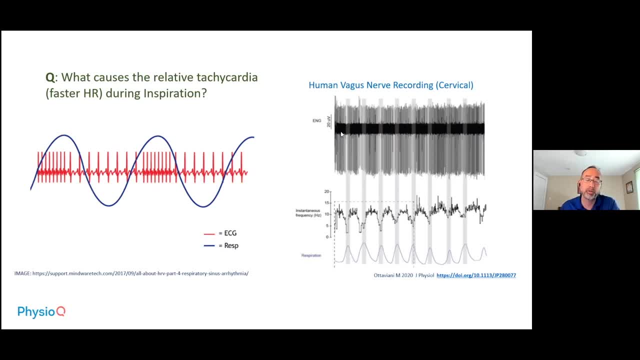 And they've actually done this in human live, human beings, where they inserted an insulated electrode needle into the vagus nerve. And you know, I'm surprised they were able to find volunteers for this, because it's a relatively dangerous procedure because the vagus nerve is right by the carotid artery in the internal jugular vein. 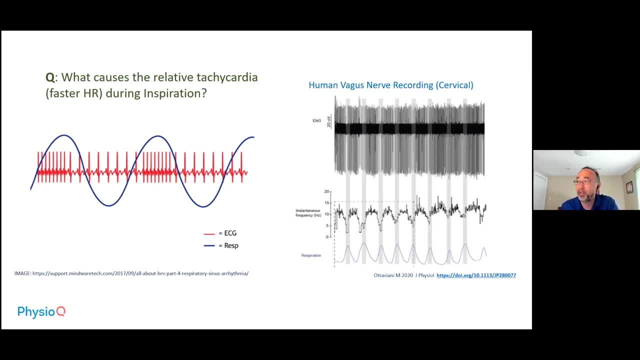 But they were able to do it. They found three volunteers. How did they do it? Actually, I think they were the study investigators And they were able to measure the number of sort of the activations of the vagus nerves And you can see here by the instantaneous frequency, basically the number of stimulations that you get per second. 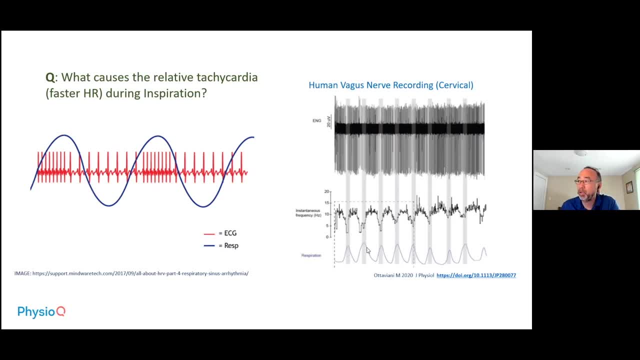 And they measured it with respiration. And so, as they're expiring, the vagus nerve is active, But when they're inspiring, they're not. When they're inspiring, the vagus nerve is silenced, And so that's where you get the rise in your heart rate. 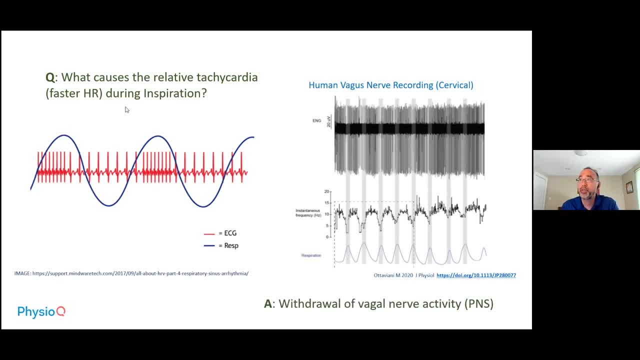 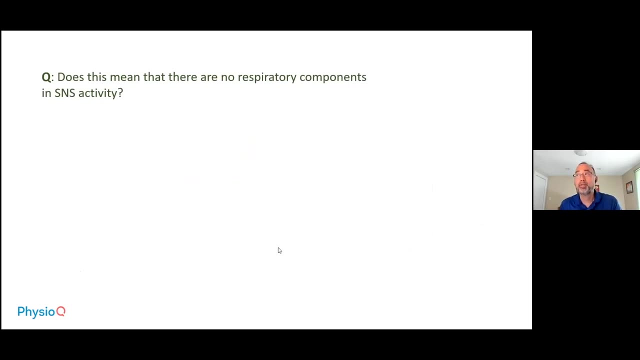 And so you see this cycle as you breathe in and out. So the relative tachycardia that occurs during inspiration is due to withdrawal of the vagal nervous activity and not to increase or enhance sympathetic nervous activity. Now, does this mean that there are no respiratory components in the sympathetic nervous system? 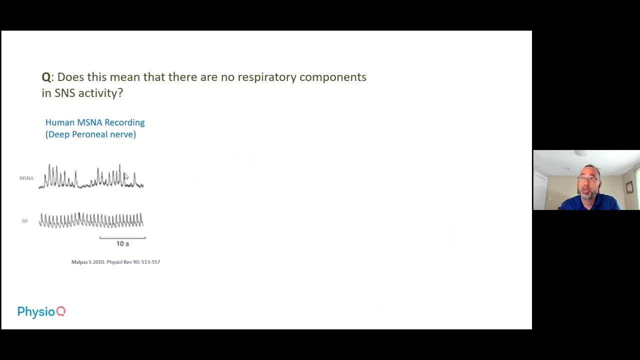 And the answer is actually no. In human beings you can insert a little electrode into the deep corollary nerves and obtain the sympathetic nervous activities. And this is an example of this And you can see sort of the heart rate as represented by the blood pressure here. 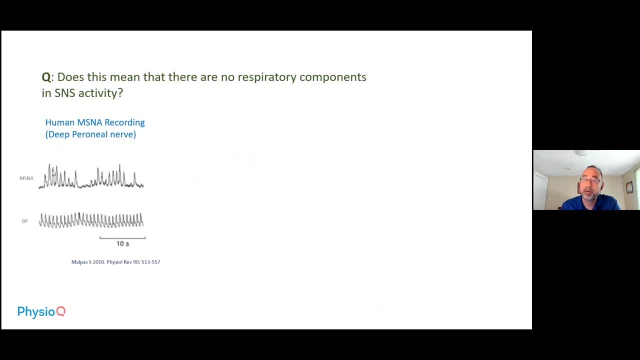 And you can see the heart rhythms manifested in the or shown in the sympathetic nervous system activities. But you could also see a respiratory component in here. And if you decide to really directly measure the sympathetic nervous system, either with a deep corollary nerve recording, which is invasive, or using electrodermal skin conductance, 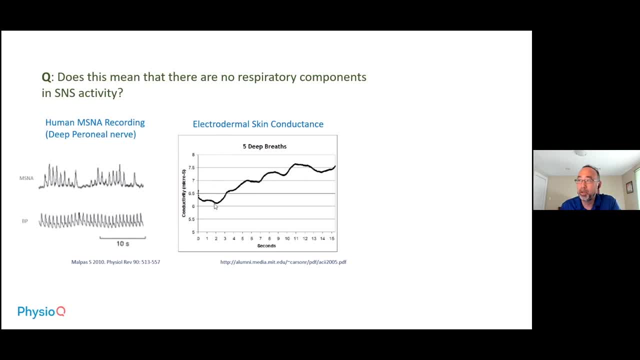 you could see here that you know this is a study that was published by MIT. They took five deep breaths evaluating the electrodermal skin conductance. You can already see these five deep breaths, And I forgot to mention that the sweat glands are operated by the sympathetic nervous system. 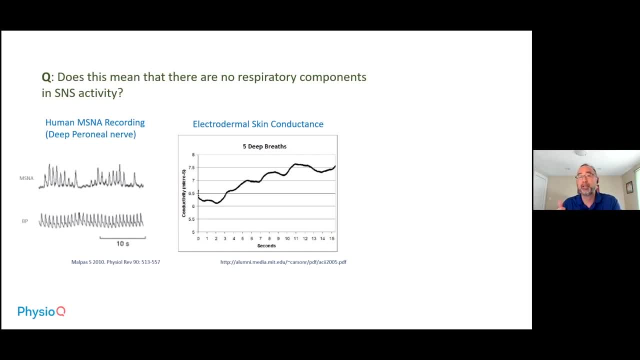 So when you have these inspirations, it activates the sympathetic nervous system, which enhances or increases the sweat gland activity, and that increases connectivity, And so that's what you see of the In this graph here. So the fact is, there are respiratory components in sympathetic nervous system. 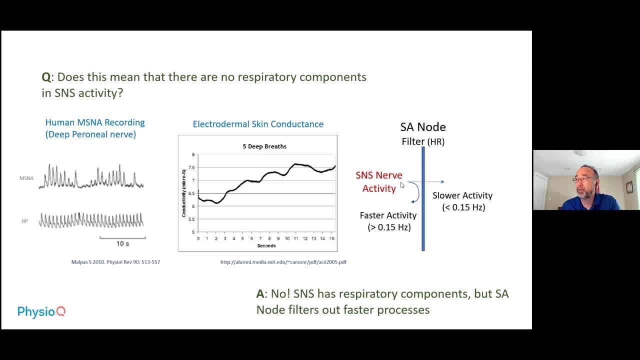 However, the SA node again filters out the faster processes, the faster activities that are greater than 0.15 hertz, And so the only thing that you see in regards to the heart rhythm because of this AC node filter is the slower activity of the sympathetic nervous system. 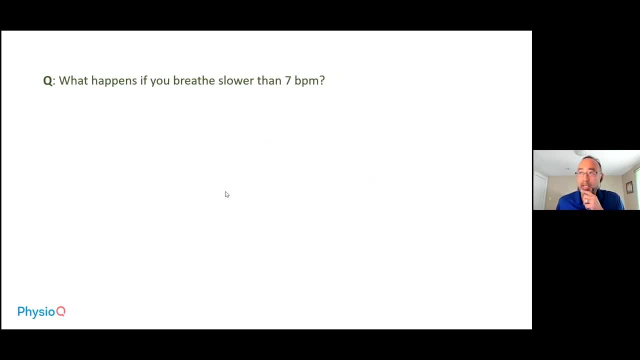 The next question. So what happens if we breathe slower than 7 beats per minute? Now that leads to the RSA, the respiratory sinus arrhythmia, then moving into the low-frequency range And so this respiratory influence effect onto the SA node. now has now a both a parasympathetic nervous system and a parasympathetic nervous system. So the respiratory influence effect on the SA node now has now a both a parasympathetic nervous system and a parasympathetic nervous system. 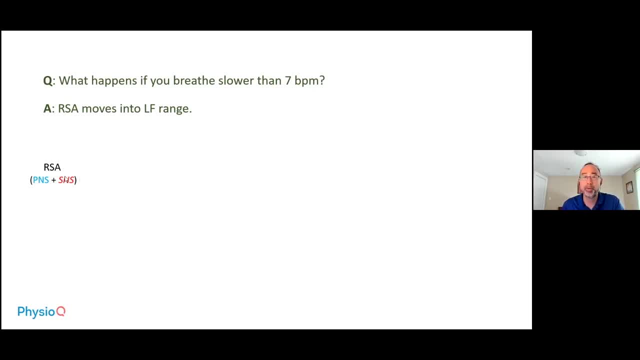 parasympathetic nervous system and a sympathetic nervous system component, because it is slow enough to invoke the sympathetic nervous system And when you are at the slower range, it enables this RSA effect to subsequently work with the baroreflex which operates around the 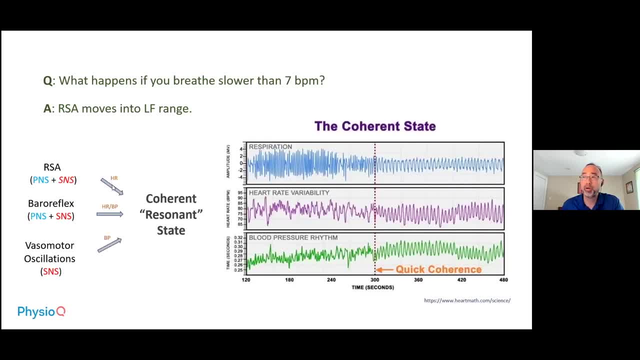 same range and the vasomotor oscillations And through the heart rate and blood pressure interactions it causes what's called this coherent or the resonant state. And if you see in this graph here which put out by HeartMath, you see sort of normal respirations and you can. 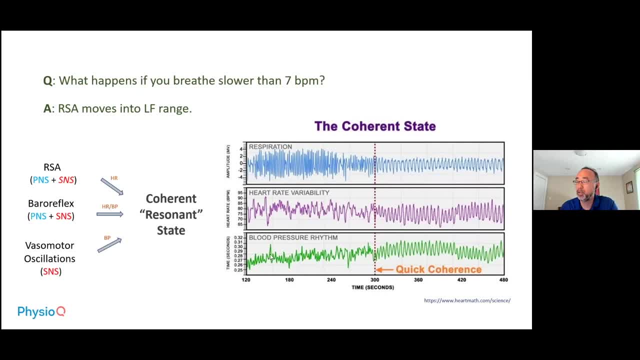 see sort of the various heart rhythms and the blood pressures. But the moment you set to a 10 second breathing rhythm or 0.1 hertz, you see this locking in of the frequency, locking of all the time series, Not only of respiration, heart rate and blood pressure as well, And some argue that this is an important way to retrain your autonomic nervous system. I don't know the detail of the literature behind that quite yet, But you know some have suggested that this resonant system is why meditation, breathing at slower rates, are really beneficial to your health. 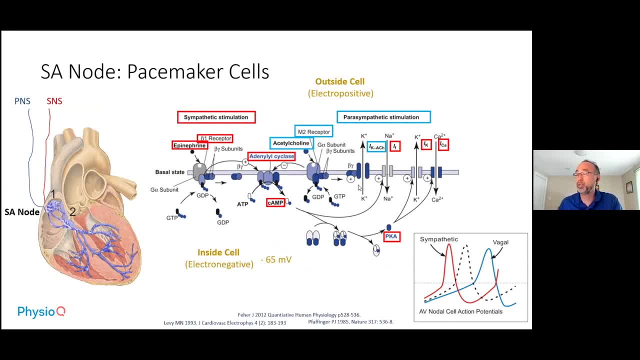 The final thing I wanted to mention in according to this graph, was that there is something called a vagal break, And when there is stimulation of the acetylcholine muscarinic receptor, there is a part here that inhibits the sympathetic, the adenylacyclase. that's part of the sympathetic. 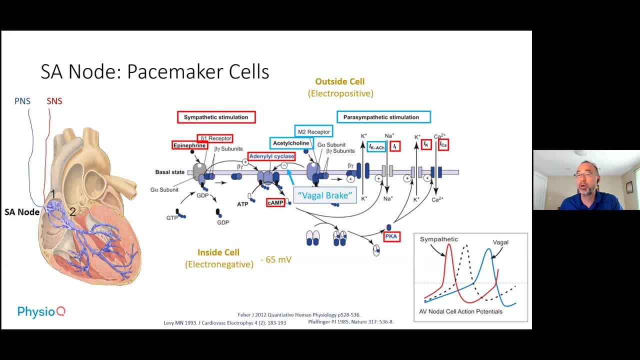 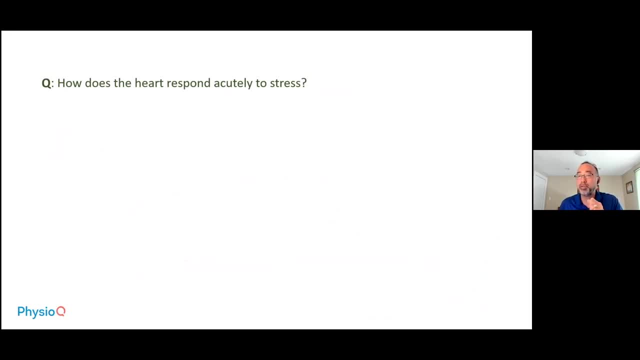 nervous system And so you have what's called a vagal break, And the reason this is important is this is related to the question: How does the heart respond acutely to stress? When I learned about this physiology of the essay, No, it sort of baffled me, because it goes. 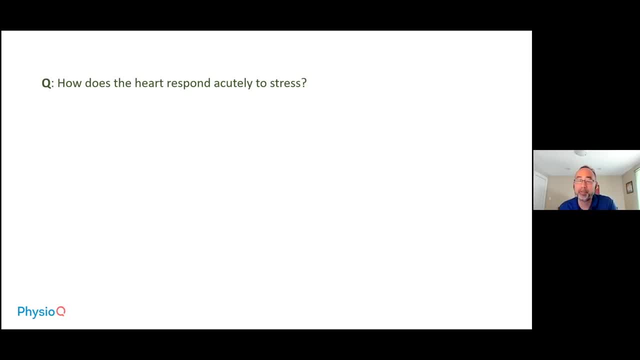 against my instinct of what would happen. from an evolutionary standpoint, You would think that if you have a fight or flight response associated with a sympathetic nervous system, that would need to act quite differently. How does the heart respond to stress? when you're feeling stress? 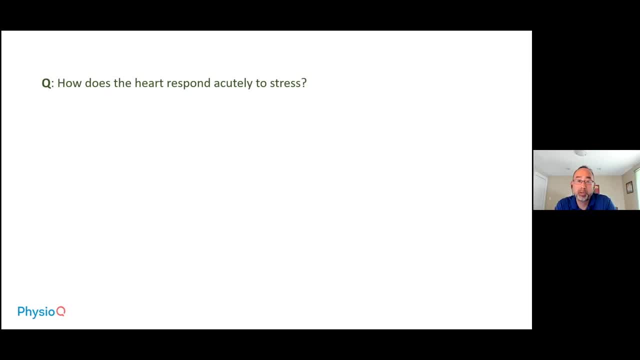 act quite rapidly and need to you know so that you respond to the threat or alarm immediately. So how does this explain our ability to respond rapidly to an acute stress? And this was assessed by a study in psychophysiology in the 1980s. They took about 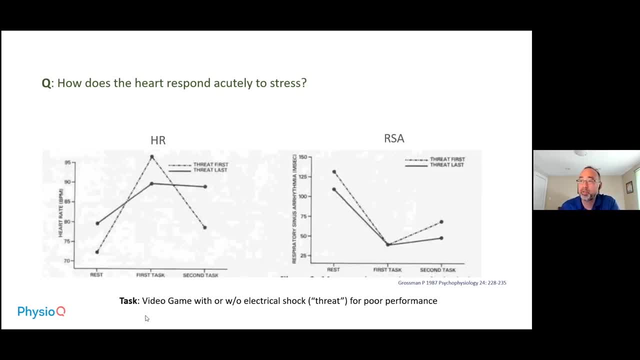 20 Norwegian undergraduate college students and they put them to a task of doing a video game, with or without an electric shock. So this electric shock was a threat when they did poorly on this video game, And you can see here these graphs on the heart rhythm and the RSA or the 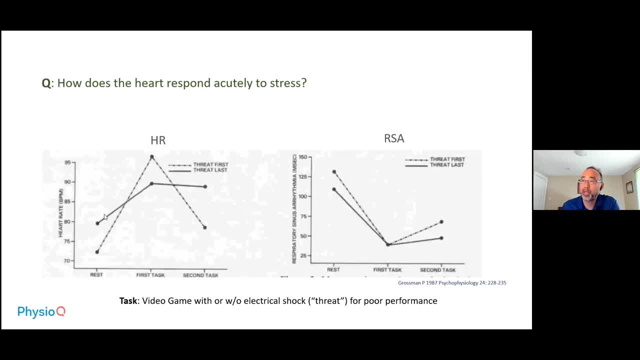 respiratory sympathetic arrhythmia. You can see that at rest their heart rate is relatively low, but when they have this threat their heart rate jumps up. And actually what they did is they randomized to either getting the shock first- you know video game with shock- either first or last, and then conversely. 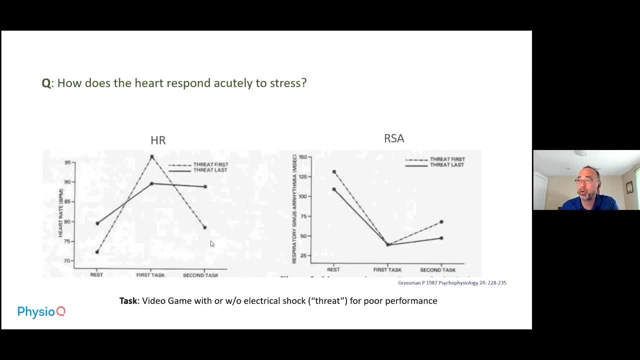 whether you get the electric video game without shock or on the second task. And then for the respiratory sinus arrhythmia, what we see is that in the beginning the respiratory sinus arrhythmia at rest is relatively high. In other words, they're 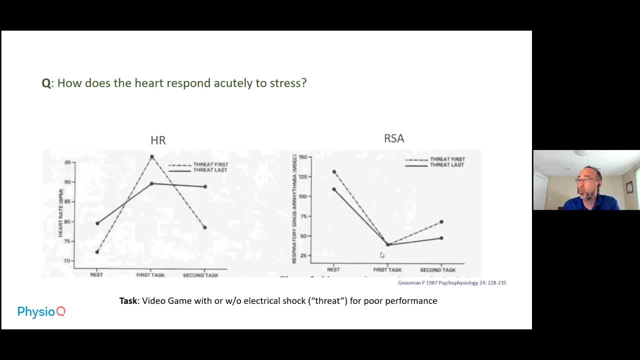 the heart rate goes up, the sympathetic nervous system is activated and then, with this threat, this RSA quickly goes down and is sustained through their second task. So the heart responds to an acute stress by removing the vagal break And the sympathetic nervous system is simply to respond to these acutely, to the stress. And I think it makes sense from a visual, physiological standpoint. why that is? it's because, um, the sympathetic nervous system does require a lot of metabolic resources and a lot of energy to make this happen. so if they, if the sympathetic nervous system, responded to every little threat, then it would be highly emotionally draining. 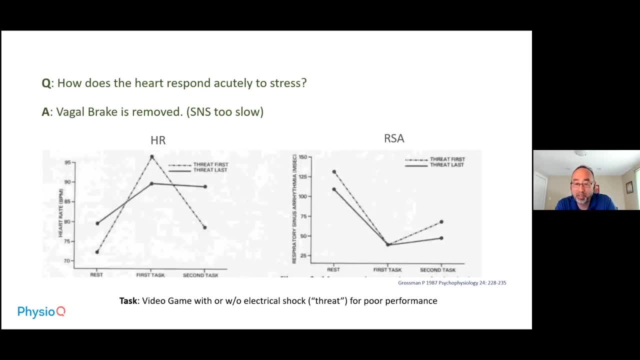 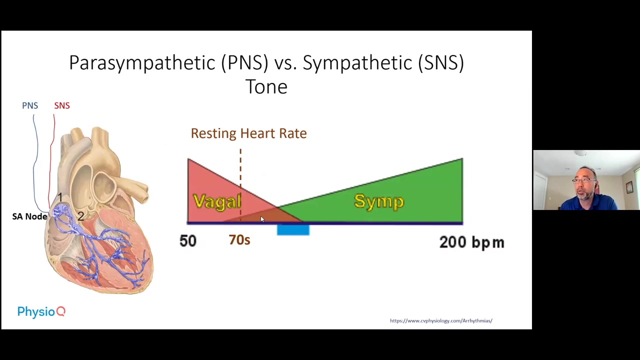 or not emotionally- probably emotionally, but also physically- draining to the organism. so the vagal system has acted as the immediate, acute function or mechanism for addressing a stress, a stressful situation, and this goes back to the prior slides, which shows that at rest we have a larger parasympathetic tone, accounting for the slower heart rate than you would see. 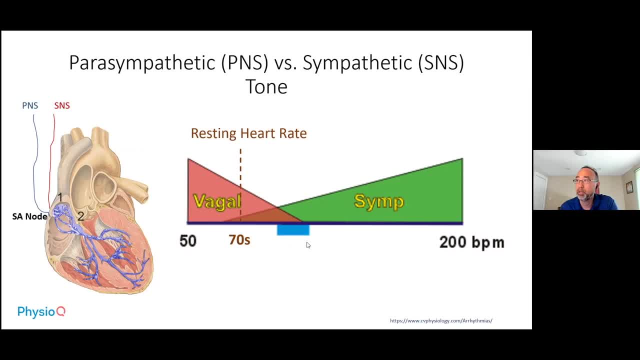 for a heart rhythm and this gives us a little bit of a buffer. so if you have a higher sympathetic tone and if you encounter a stress, you are, enable this parasympathetic nervous system to subsequently deactivate and enable the sympathetic nervous system to kick in and you can understand why. 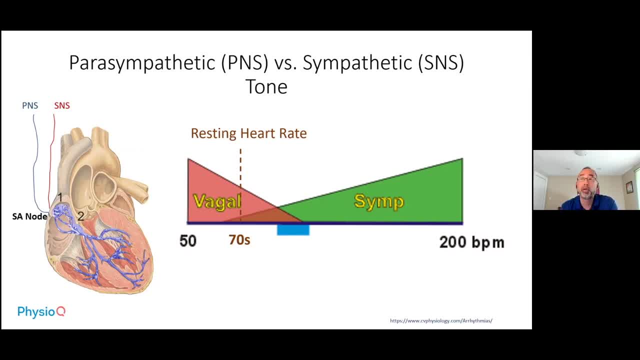 this tone is important. now, if you don't have this tone, if this parasympathetic nervous system is constantly inactivated or lacks uh significant activity, when you encounter a stressful uh situation, you don't have significant, that significant tone reserve to to inhibit so that you're able to address that stressful situation acutely. so i think this is one of 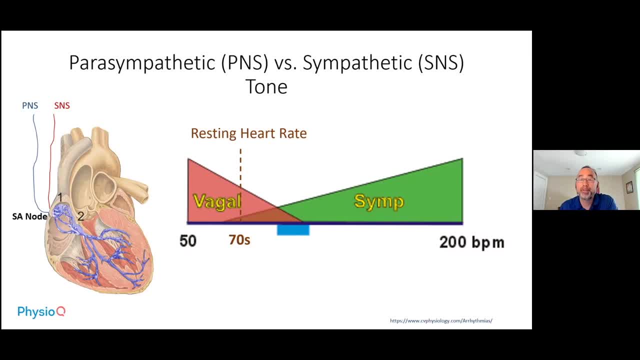 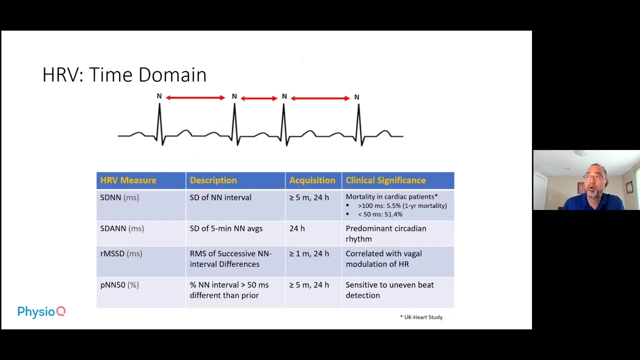 those things that it's important to know, uh, when we're evaluating the subsequent clinical studies or some of the physiological or psychological studies and we're going to talk a little bit more about the time domain and why the present effect nervous system has is so important. now we have a little bit of time to quickly go through the time domain and, as i mentioned before, 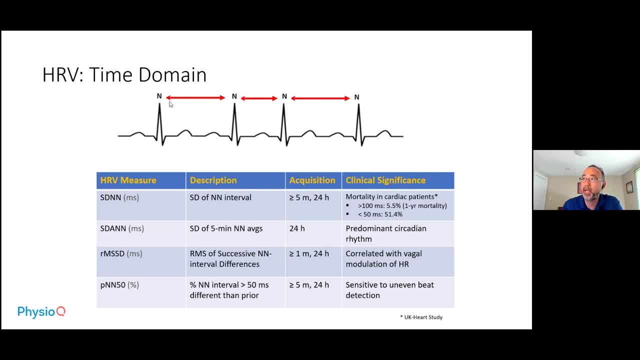 we're not focusing on the r interval, but the n and article interval, the normal rhythms that are associated with the sa notes and the four big ones that i want you to pay attention with. there are various others, but the ones that are, you know, account for the majority of time. domain measures in: 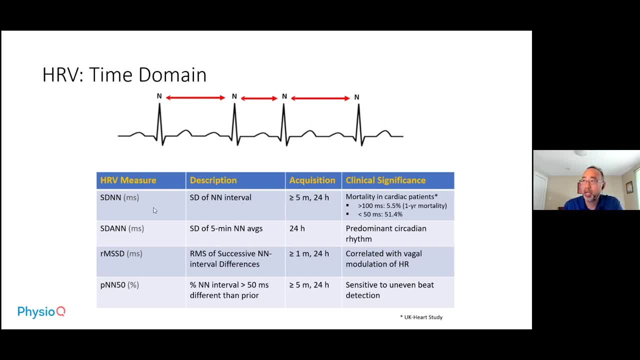 the literature out, there are these four: the standard deviation of n intervals, the standard deviation of five minute averages of the n intervals, the root mean square of successives and n intervals differences, and then pnn 50, which is the percentage of n intervals that are greater. 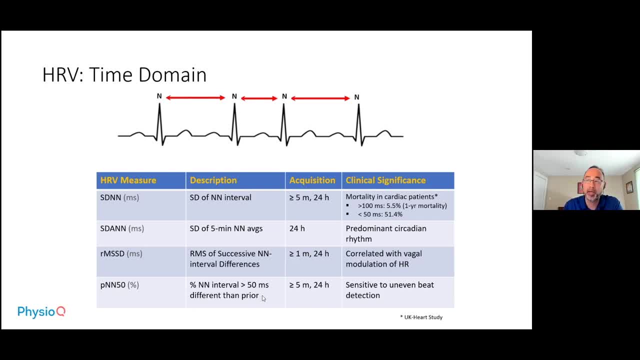 than 50 milliseconds different than its prior n intervals, and each of these sort of require a certain amount of time. um, i think, for uh, for these, uh, for these, um the rmssd pnn 50, uh you are, you could use up to five minute, five minutes. some have used as little as one minute for rmssd um for standard deviation. 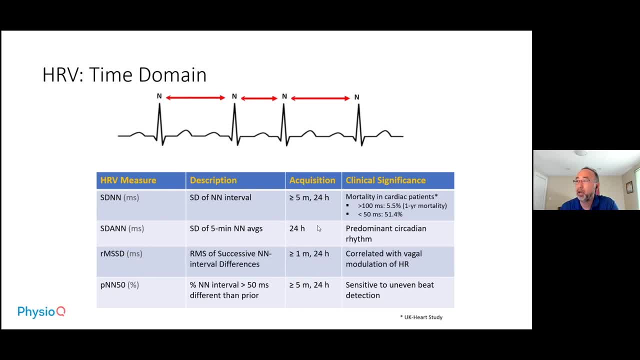 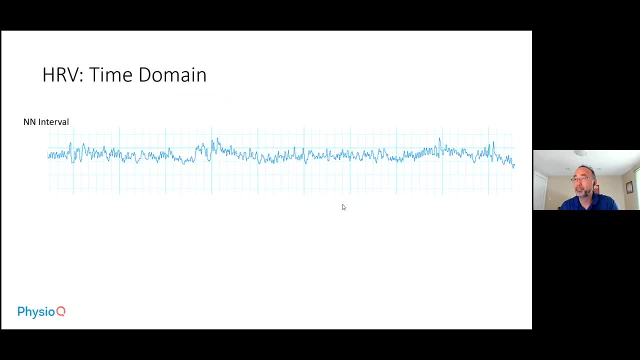 of at an interval and sdann. uh, i think a lot of them have used 24 hours and the clinical significance i will talk about a little bit later. so, um, if you take a look at the n interval over time, you can see a lot of this. 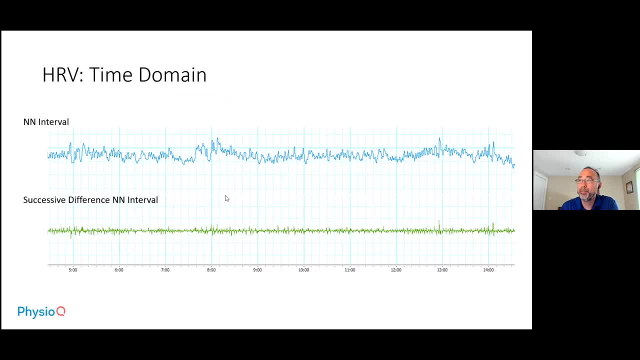 variability and um, the two of the four time domain measures- takes a look instead at the successive differences in the n intervals, and it's basically the difference between the r in an interval compared to the prior one, and this is how it looks like here. so, if it, if you're, 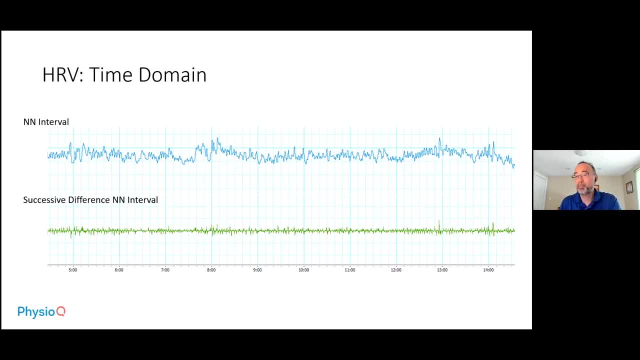 a beat was 50, if your heart rate was about, you know, 50 beats per minute on one time and then it subsequently was, or let's just say it was 50, 80 milliseconds for the first n interval, then it was 90 seconds on the subsequent interval. then you have a 10 millisecond difference between the two. 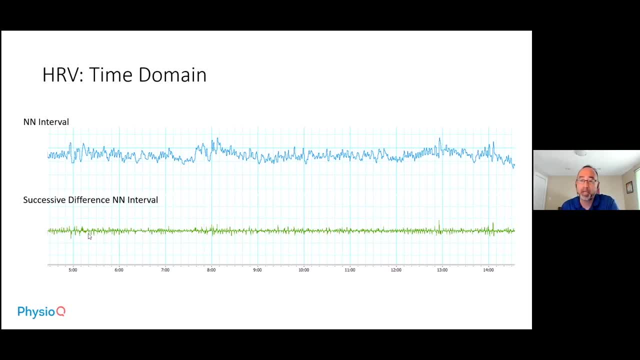 that's what they use in order to put out this time series. and you can see that this time series it eliminates a lot of this slower dynamics that you see in the nn interval and you see a lot of the faster process that occurs. and so rmssd, which is the root, 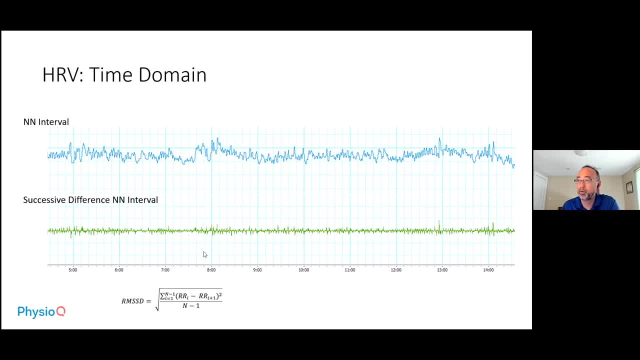 mean squared of ss of this graph here, and pnn50, which is the number of times that you have. the successive differences go either above or below. these thresholds are an indication of these more rapid events, because you lose a lot of the slower components of your heart. variability when you 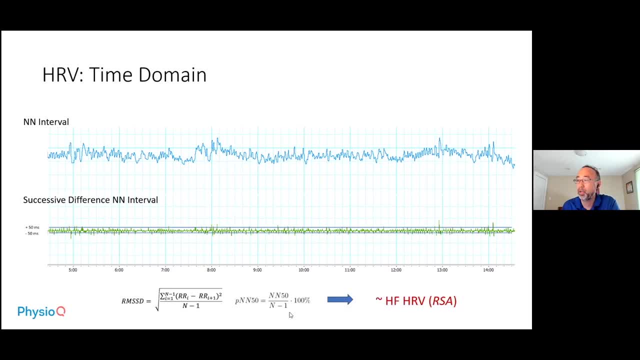 evaluate the successive differences in intervals. so, when you're dealing with these measures, you're dealing with the faster components of your heart rhythm, and so you're talking about high frequency, heart rate variability or the respiratory sympathy arrhythmias, which we recall, is largely a parasympathetic system, uh, a phenomenon. 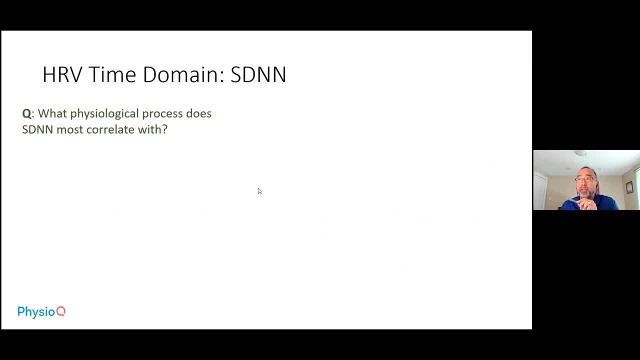 so the question is: what are the physiological processes? uh, most correlated with sdnn or the standard deviation of the nn interval? and the answer is: it really depends on the duration of the data- for two minutes, because we're doing predominantly with higher frequency information or variability, the standard deviation. 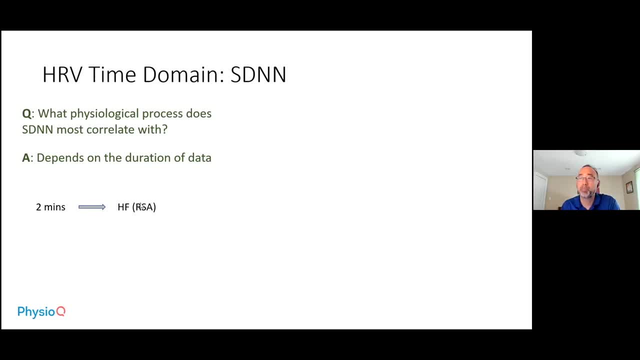 sdnn, uh reveals or represents much more variation, or rsa or fear, that nervous activity for five minutes you're invoking both the left, both the low frequency and high frequency components, so you have both the repair PEier reflex and the rsa physiological processes within that signal. and then 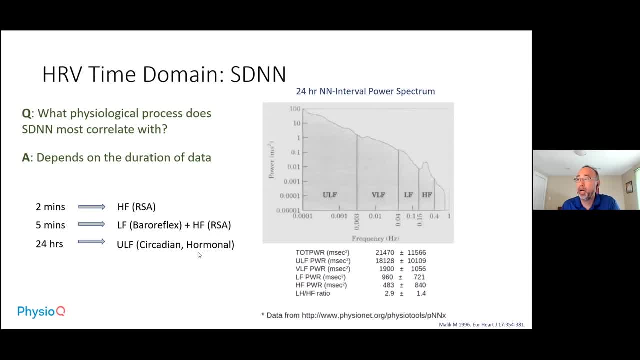 when you're talking about the 24-hour sdnn, it is predominated by much slower processes, and you canz see that of each of these frequency ranges, You can see that high frequency, low frequency generally has lower power, And so for the lower frequencies, 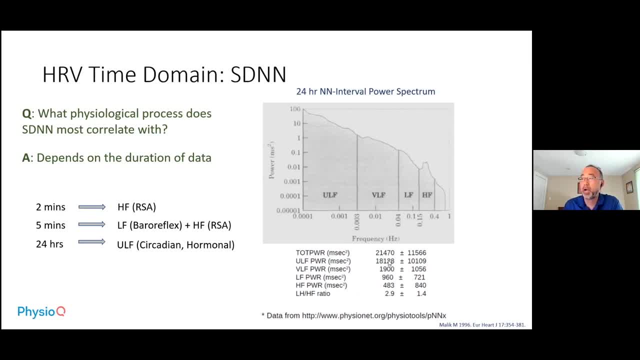 the very low and ultra low frequencies. they have a much higher power representation in this power spectrum. So when you're obtaining a 24 hour standard deviation, a lot of the variability is accounted by these slower rhythms, And so it represents the SDNN of 24 hours. 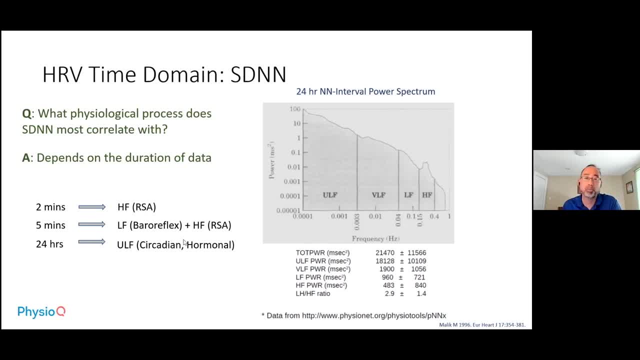 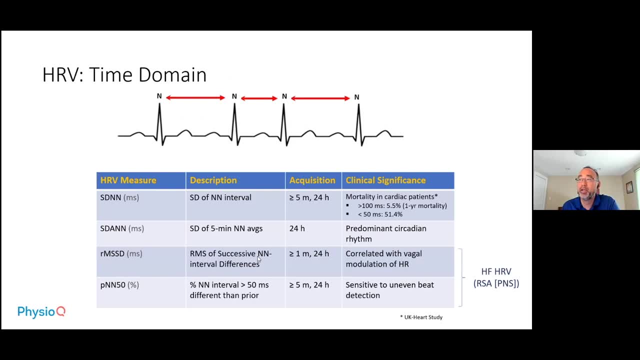 represents the circadian or slower hormonal processes. So, in summary, these two measures, which rely on the successive NN intervals- RMSSD, PNN50, represent high frequency, heart rate variability or respiratory sinus arrhythmia, And so indicates much more of a parasympathetic. 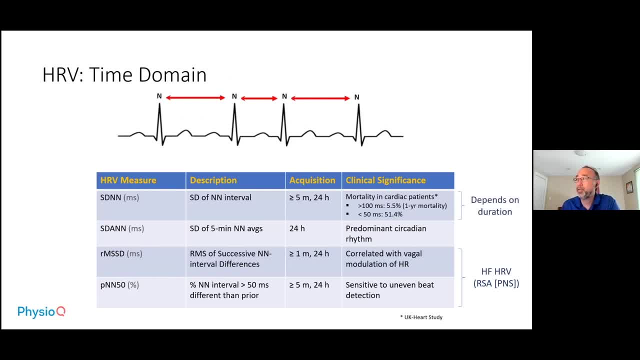 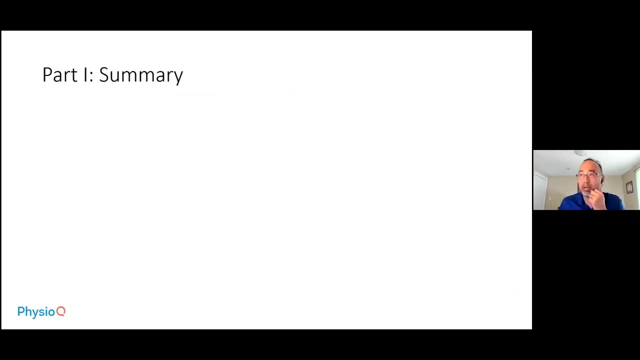 nervous activity. SDNN depends on the duration. The shorter that it is, it's more correlated with the higher frequency ranges, And then SDA, and NN here associates more with the circadian rhythm. So that is basically the end of the part one. 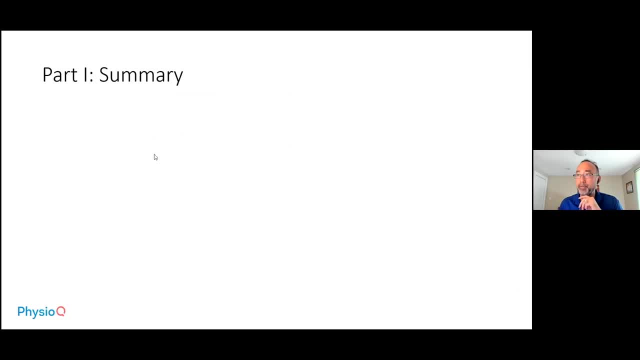 of this heart rate variability deep dive. And just to summarize, 1970s and 80s saw the major advances in heart rate variability. and just to summarize, 1970s and 80s saw the major advances in heart rate variability. and just to summarize, 1970s and 80s saw the major advances in heart rate variability, physiology and measures. At rest, parasympathetic nervous tone normally is greater than the sympathetic nervous system. tone And heart rate variability frequency domain. 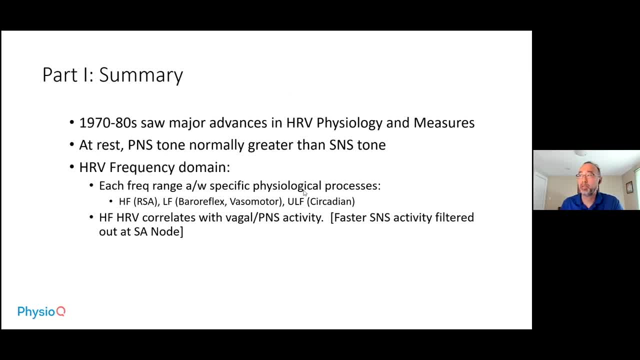 for each frequency range is associated with a specific physiological process. High frequency is associated with RSA or the parasympathetic nervous system. Lower frequency is associated with baroreflexin and basal motor, which are both have both a parasympathetic. 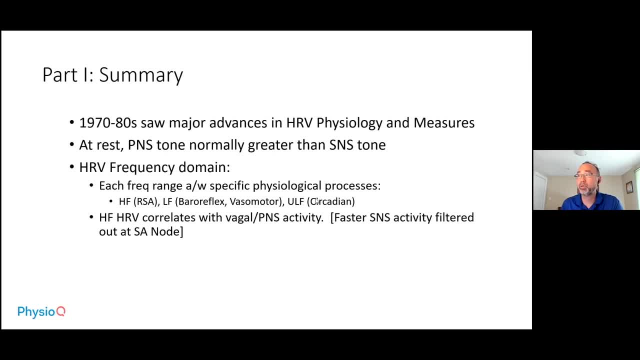 and a sympathetic component, And the ultra low frequency deals with hormone or circadian rhythms, And high frequency heart rate variability correlates with vagal sympathetic nervous system and the faster SNS activity is filtered out at the SA node. For the time domain, measures RMSSD and PNN50 correlate. 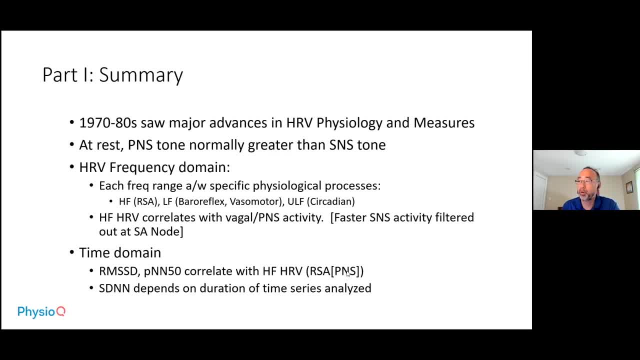 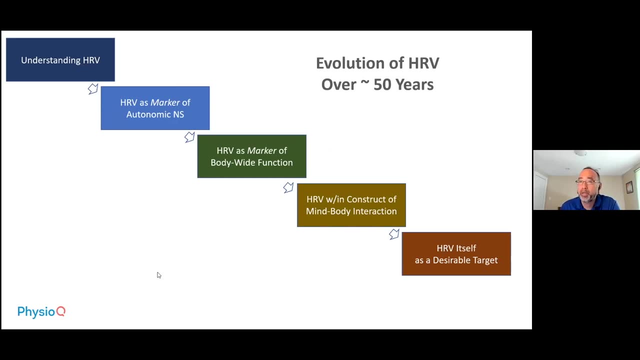 with high frequency, high heart rate variability and therefore represents our representative by the parasympathetic nervous system And SDNN. depends on the duration of the time series analysis Now, because there's so much information here, there's probably going to be two or three more subsequent. 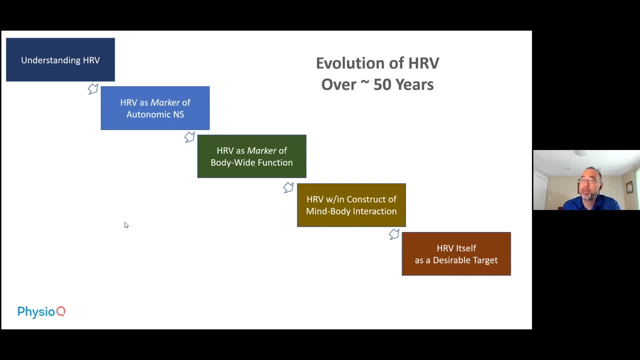 talks on heart rate variability, And some of the things that I'll talk about in the future will be the clinical studies, some of the physiological tests that are used to assess autonomic nervous system, non-linear measures and some of the applications of heart rate variability. 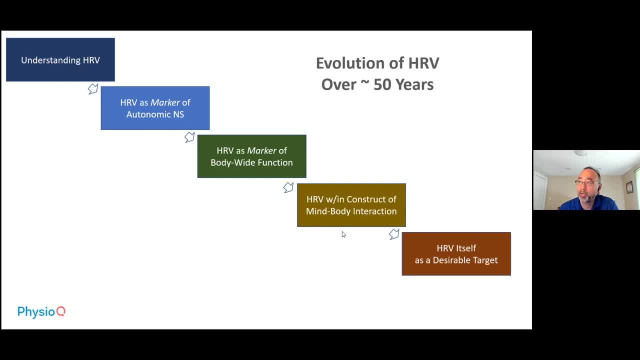 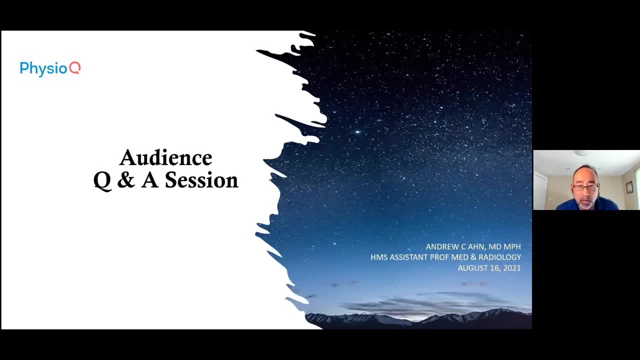 in psychological situations such as stress and sleep as well. Well, that's it, and it's time for questions. Thank you so much, Dr Ahn. that was great. Yeah, so we're going to jump into our Q&A section now. 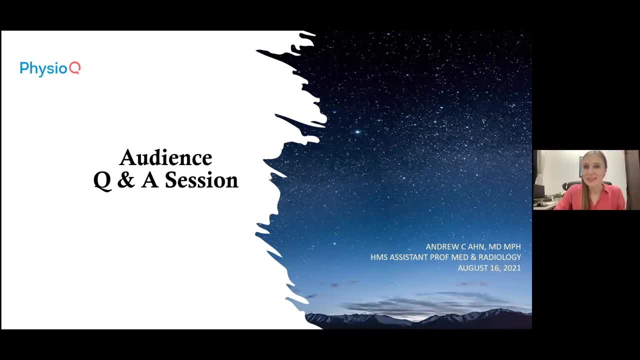 I'm looking at the chat And it looks like your talk was extremely clear and there is no questions that I'm seeing. But I'll give our attendees a few seconds or even a minute to think of any questions they have, And you're free to ask away. 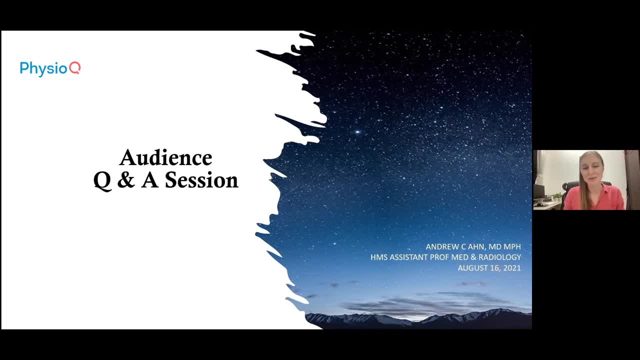 And if you have a question that pops up later, that's also fine. You can email us at support, at physioqorg. I'll write it in the chat and ask your question then. So, Thank you, Thank you, That is the email that you can feel free to send your questions to. 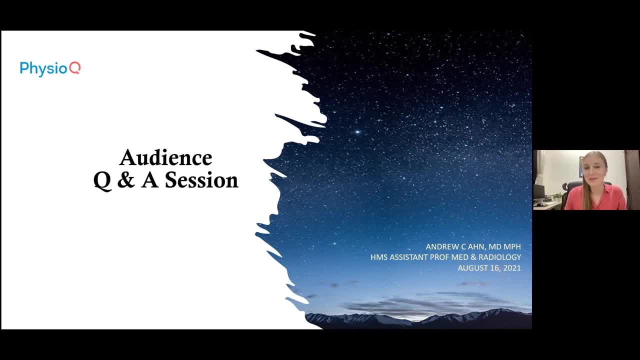 And I'm going to ask you, Dr Ahn, to stop sharing your screen, if you don't mind, and I'm going to jump on and just introduce the next session quickly. Yeah, I'm trying to do that. Let me see how I can do that. 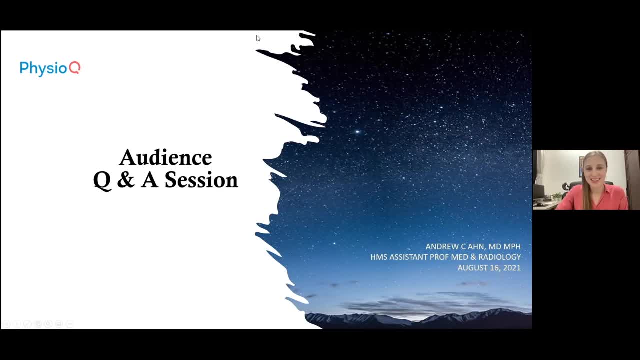 Oh, here it is, And I do want to thank everyone for coming as well. So thank you so much, Dr Ahn, for doing this session for us. It's amazing. We really, really appreciate it, And thank you so much to everyone for joining. 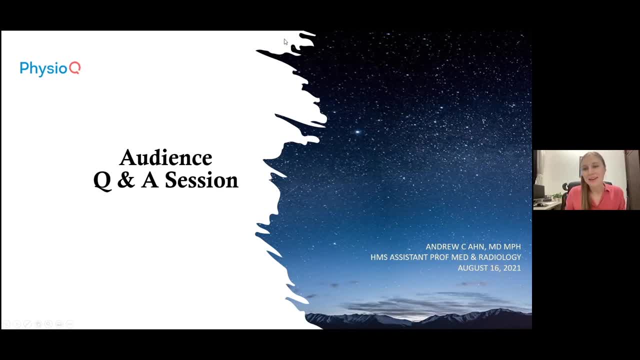 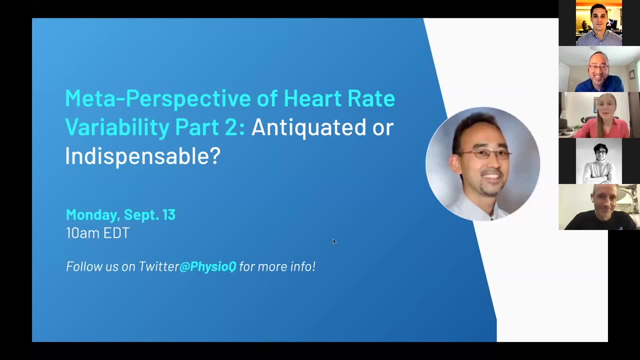 I'm seeing a question pop up. So, Dr Ahn. it says: will the presentation be available on our website? I think that's a question more for us. Yes, we will be posting it, Since there's going to be a follow-up session as well. 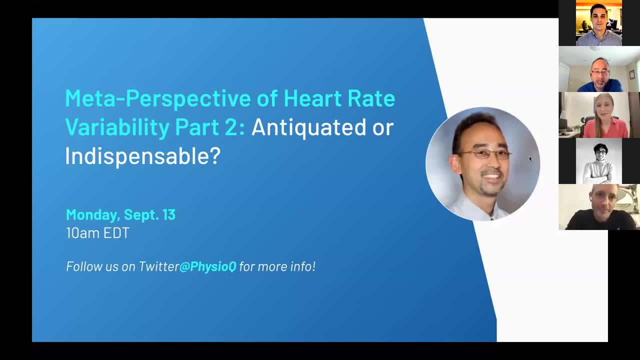 we'd love for people to have access to this. It's a free workshop, So, yeah, we will be posting it on YouTube on our channel. Dr Ahn, I'll read you the next question. I'm not sure if you have the chat in front of you. 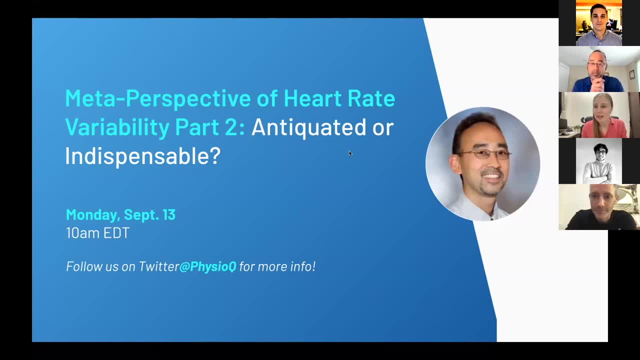 But there is another question It's popping up. It says: besides the frequency domain and time domain, are there any other series? Yeah, Yeah, I mean there's the nonlinear measures of part rate variability which I briefly talked about in one of the slides. 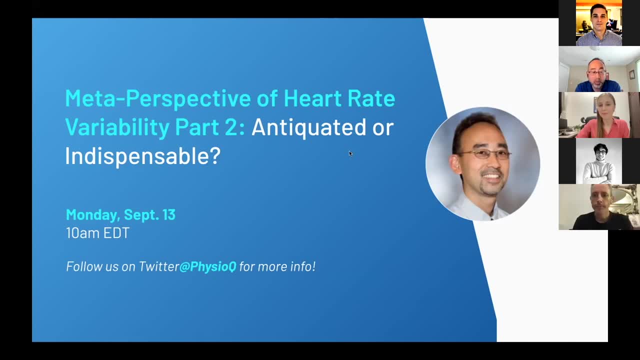 And those include a lot of the things that were developed in the 2000, 2010s, actually as early as the 1990s. It includes detrended fluctuation situation analysis, Poincare analysis, multiscale entropy. 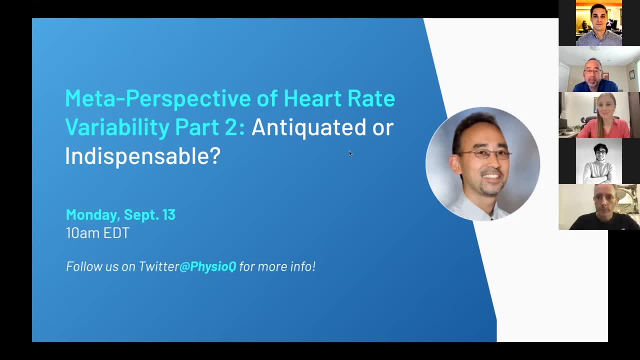 Those are a lot of the measures that are really complex And I probably won't spend too much time on them, But it gives you a good sense. It's supposed to give a universal holistic understanding of heart rate variability And I'll probably touch on that on the next talk. 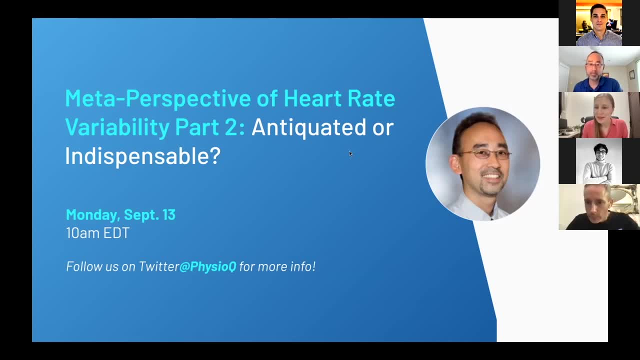 Great. thank you so much. I'm seeing some more questions popping up. That's great. We have another one. What's the main challenge for HRV to be used clinically in your opinion? Yeah, that's one of the things that I'll. 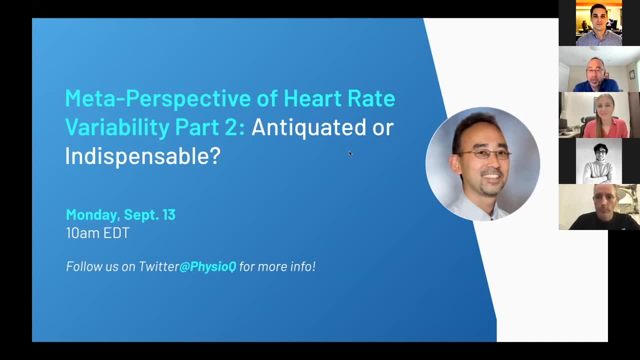 touch upon in the next talk. The challenge with heart rate variability is that it is quite sensitive to a number of factors, Like if you're stressed, if you've even drank coffee, or if you had a bad sleep the night before. those are all things that lead that. 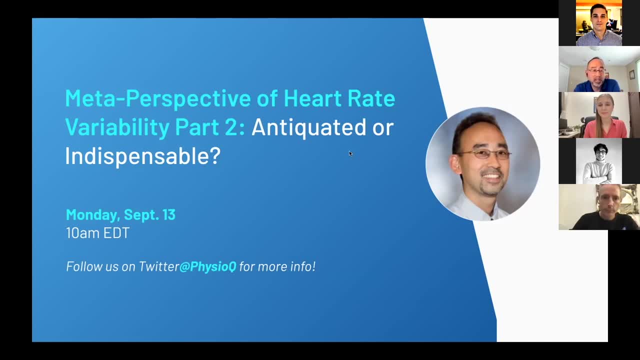 can affect heart rate variability. So heart rate variability is highly sensitive And in the clinical setting we often consider those factors as noise And that's why we generally try to. I mean, I think that's why heart rate variability is not commonly. 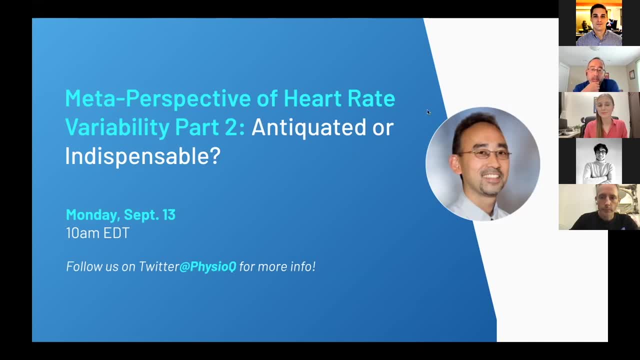 used. It's just that it is highly sensitive and makes it hard for us to utilize it. And when they do use it, it's under very controlled settings. But I will talk about that in the next setting. All right, We're looking forward to it. 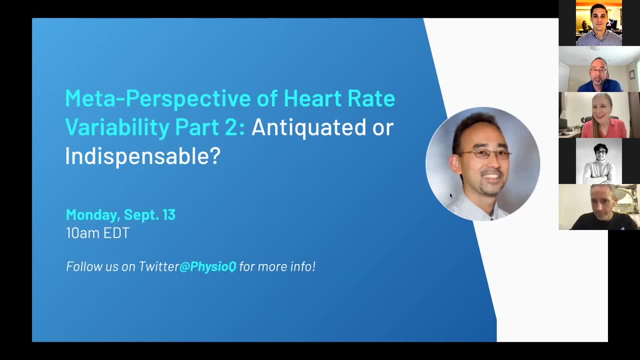 I'm seeing one more question. Lots of praise, Well done. The question I'm seeing here says: does it mean sympathetic activity cannot be captured by frequency or time domain analysis of HRV? Well, yes, you can get sympathetic activity from frequency analysis. 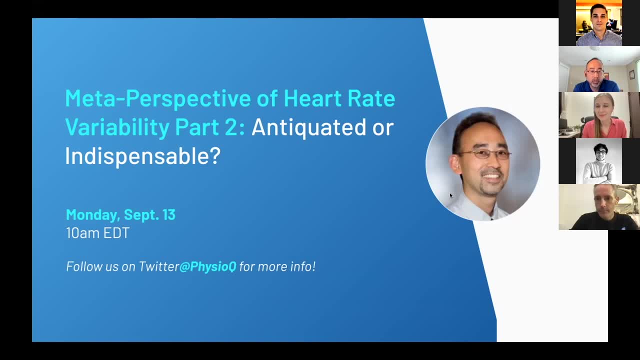 But it isn't. I mean, it's not a direct measure. So when you're talking about low frequency, where people, for example, have equated in part with sympathetic nervous system, it has a sympathetic nervous system component in it, But it's not totally clean. 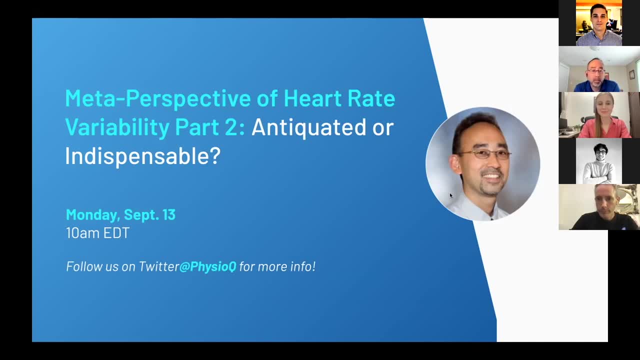 There are some vagal or parasympathetic system involved in there as well, And this is where I think sometimes what you have to do is you give a little bit of an intervention. For instance, we know that the sympathetic nervous system is activated when you go from a supine or laying down. 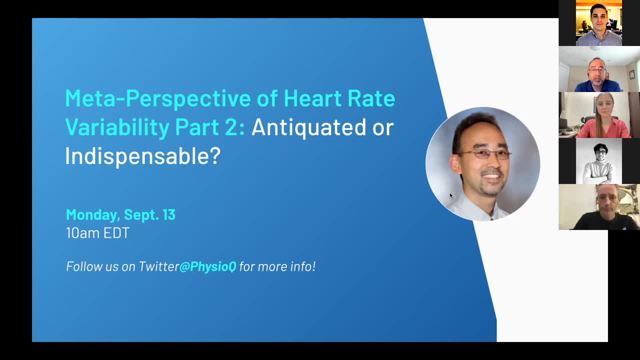 to a standing up state. So you do these little interventions that we know impact the sympathetic nervous system And you see how that affects your frequency domain analysis. So that's how they do it. Sadly there isn't a really great measure to directly measure sympathetic nervous activity using heart. 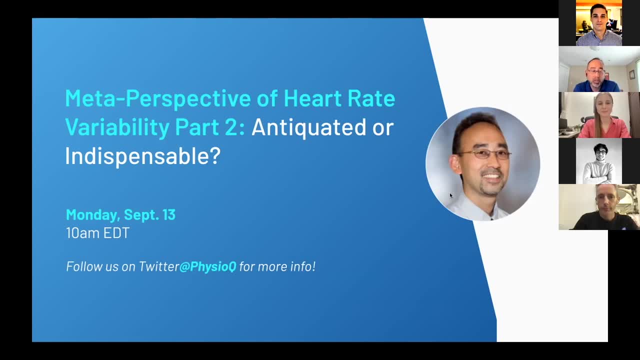 rate variability. But this is why I briefly mentioned the electrodermal measures, which may be a more direct measure of sympathetic nervous system For the time domain analysis. that has a lot of course issues when it comes to sympathetic nervous system. 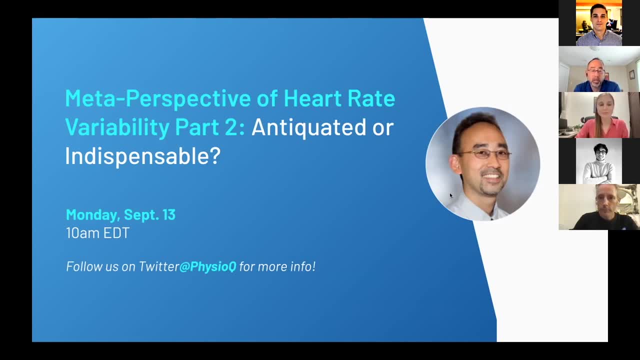 So I do not use time domain for evaluating sympathetic nervous activity. Great Andrew, I'm going to read the next question to you: How long should a baseline measure be using PPG for HRV? So this is from Joe Brandenburg. He says at Penn State we are currently 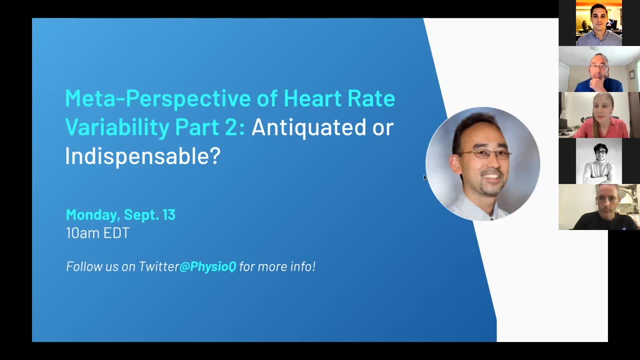 looking at intervention implementation based on live readings of HRV And we are trying to decide where an individual is stressed relative to an accurate measure of their resting HRV. I know there are a number of papers that outline standards for HRV using ECG. 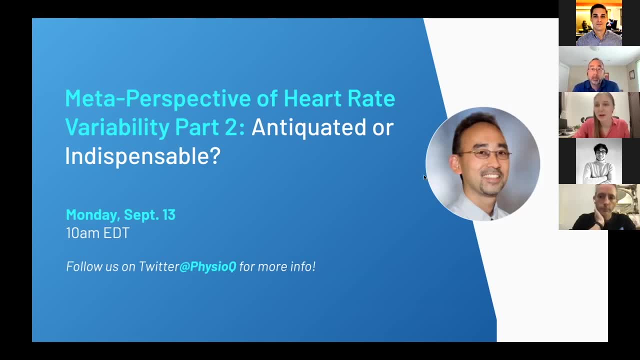 but none that I'm aware of giving general guidelines for wearable HRV research. Yeah, that's a great question And that's something that I could spend a lot of time going into much more detail, But generally when you're talking about an intervention, 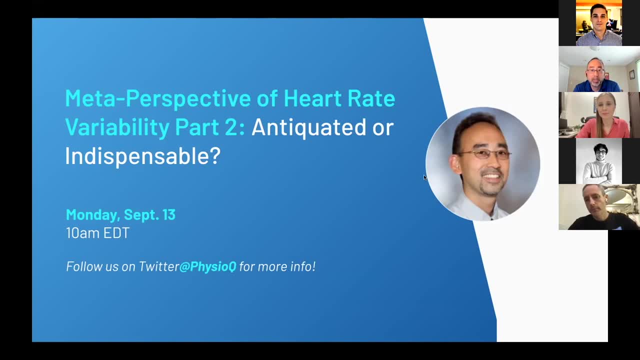 whether it's some kind of stressful task or something like that, then I would say a few minutes, And then I would say a few minutes. So I said that the Oilers, the HACS tasks would even be sufficient for that, even for PPG. And the reason is- and I think what's commonly used is RNSSD- in those situations When you have- you know, because RNSSD assesses the parasympathetic nervous system in winter- stress that parasympathetic nervous. 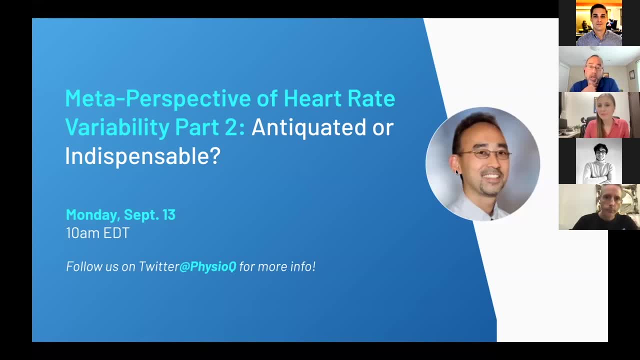 system is deactivated and you see that as a reduction in the RNSSD pulse rhythm that you get in these wearable watches. The challenge, though, is if, oftentimes, when you're doing these types of studies, they're done in healthy individuals, But if you're dealing 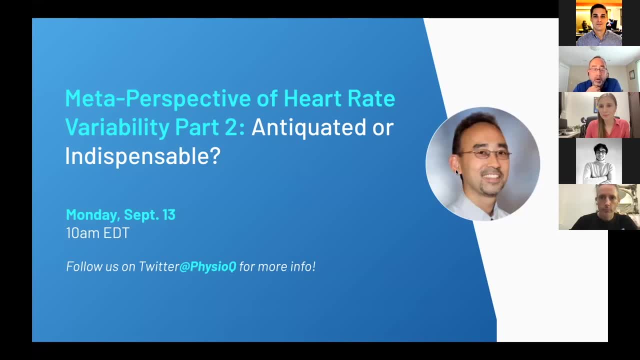 with people with chronic medical conditions. those who have heart disease, such as coronary heart disease, congestive heart failure or at baseline have atrial fibrillation. it's just really hard to use any type of wearable device to assess whether that individual is stressed or not. 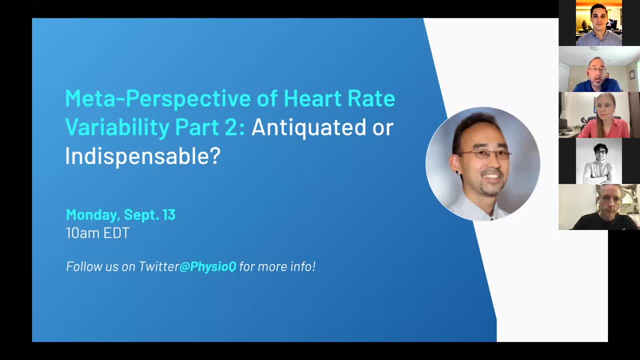 because there's a lot of ectopic beats that don't go through the SA node And, as a result, the information that you get through the PPG is not representative of the autonomic nervous system. So that's what I would say, And what I would probably also recommend is you can get a baseline. 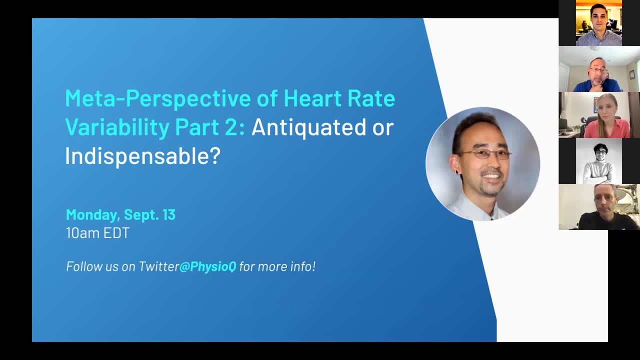 EKG, Which is not that hard to do. In fact, PhysioQ, I think, works with Polar, And Polar is another type of device that can be utilized, And you could just do that to obtain a baseline EKG to see whether that person, that volunteer, for instance, has a lot of ectopic beats And if 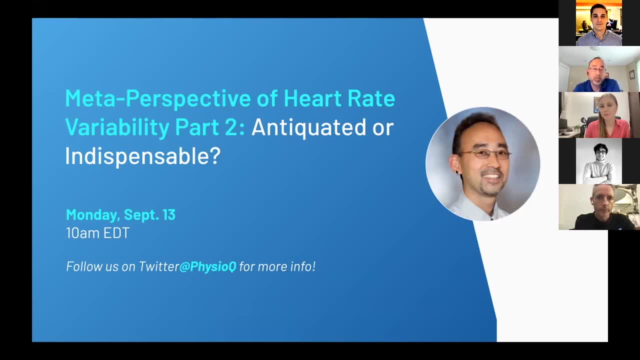 there is, then you probably don't want to utilize PPG for assessing stress response. So I hope that sort of answers the question. It's a little long. Thank you so much. There's one more question I'm going to ask before we wrap up. 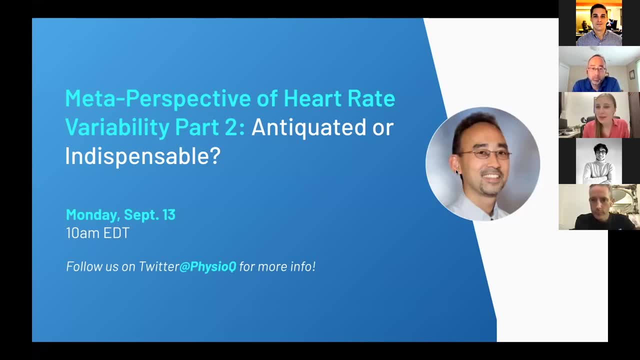 As you mentioned, there are many subtypes of HRV. Which one is the best or most important? that can imply clinical application. Does the wearable device measure, since it interprets PPG? Yeah, that's a good question. Again, that's something that I will talk about in the next. 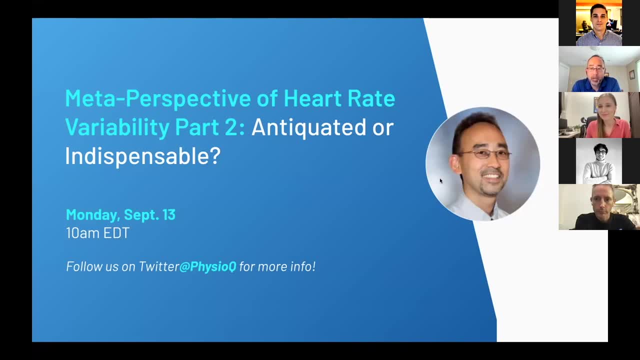 talk or next seminar series. Interestingly, a lot of the clinical studies have used a number of heart rate variability measures And this is what makes this literature so hard to decipher. It's because there are so many different measures and used in different settings, In general the ones that are most commonly used for time domain. 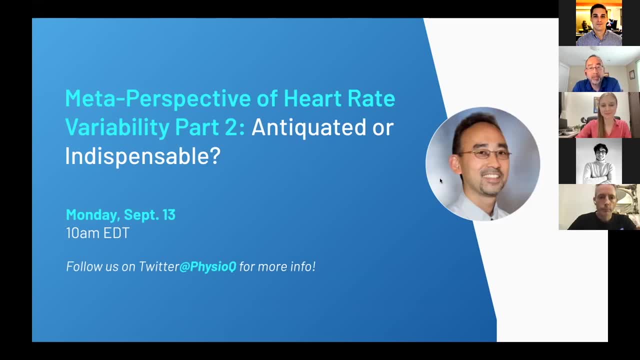 is RMSSD, PNN50, which were used in the older clinical studies, and occasionally standard deviation or SDNN. And what was really interesting is in the public health studies, like the epidemiological studies, the ones that was most useful or imparted information about prognosis, like 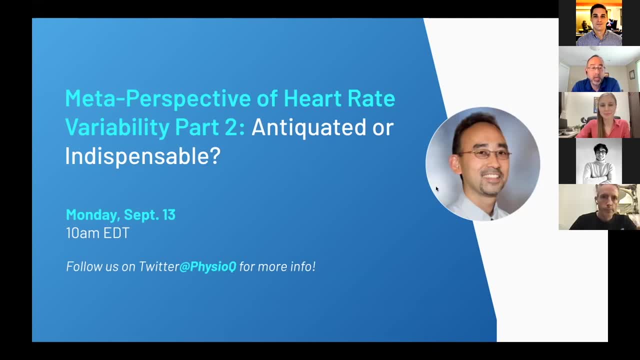 if one was more at risk of mortality, it was the very low frequency component of the heart rate variability that was the most important, And so that is something that is just not emphasized in a lot of the things that we see in sort of the wearable research field, So it's not a 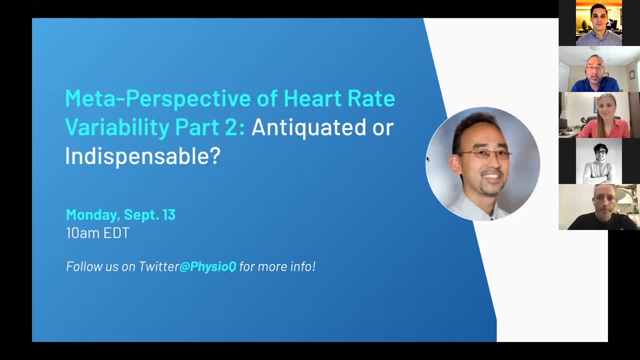 straightforward question. I wish I could give a better answer for that, But you know, it's one of those topics that I should hopefully address in the next talk. All right, I think that just about wraps up our. Oh, there's one more question, Just. 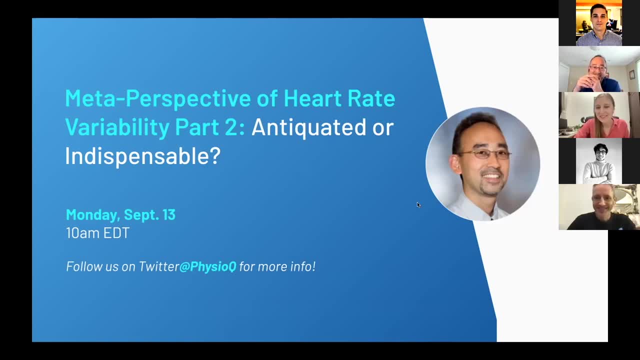 kidding. Okay, I'll allow it. Is there a correlation between HRV and oxygen saturation level? No, not yet. Okay, Okay, Not directly. So oxygen, so heart rate variability is basically the change in the heart rhythm, So you know how fast or slow the heart beats. Oxygen saturation deals with the amount of 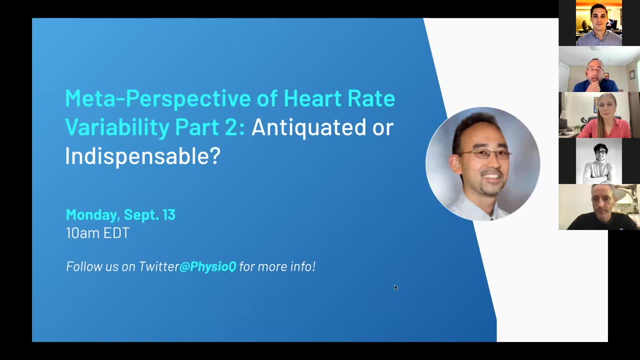 oxygen that's within the blood And the way you obtain heart rate variability. like, just to say, for a wearable device. the wearable device uses a single frequency light. It's often green. The green is the light that's used to reflect off the hemoglobin in the blood system, And 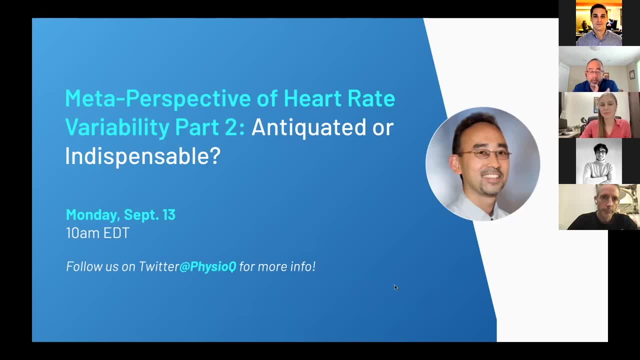 so you have one light that's shown in from the watch. You can see that there's a green light that comes off the back of the watch. It uses that one light in order to assess rhythm, So you can see how much flow that goes through the small vessels to determine. how fast your heart is beating. Oxygen saturation, on the other hand, requires two frequency of lights, Because that's the way you could determine how much oxygen is in the system. So the oxygen saturation functionality in wearables require much more battery. So you don't see that in. 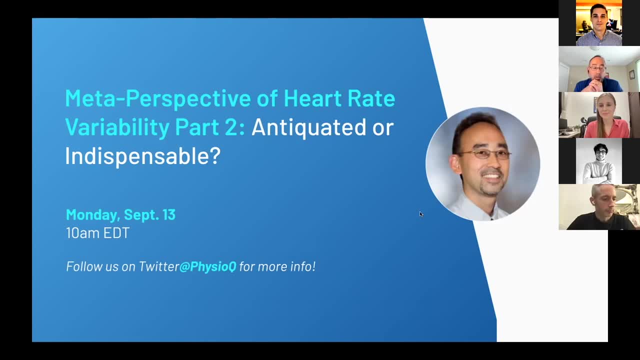 all wearable devices, And so it could- you know it could- wear off the battery life for your device. It provides completely different information, in other words. So you know that's something that you know. certainly I could talk in the future as well, but it's. 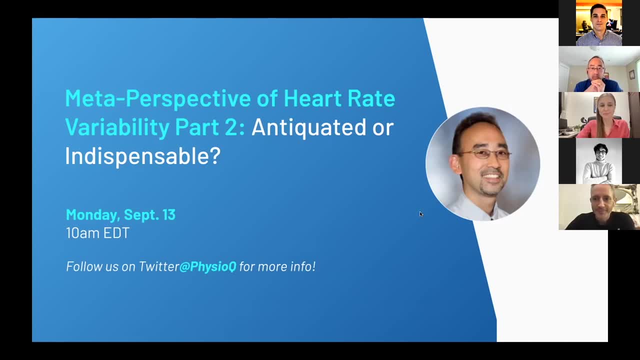 probably not going to be part of the heart rate variability series, All right, So thank you so much, Dr Ahn. again, We really appreciate it. Thank you for everyone else for joining us today. I do want to steal another 30 seconds of your. 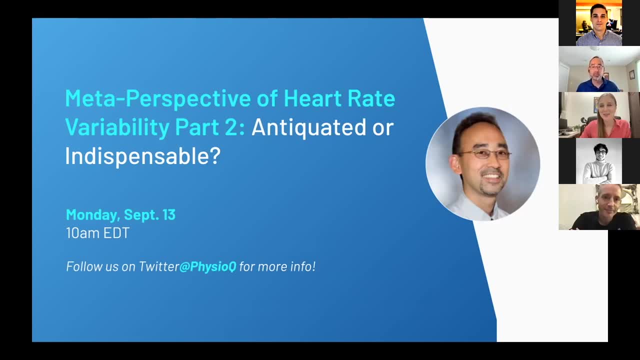 time. if you don't mind, I've just launched a poll. There's two questions. If you could please complete this little feedback survey, that would really help us be able to better tailor these kinds of sessions to you in the future. We're always looking to provide. 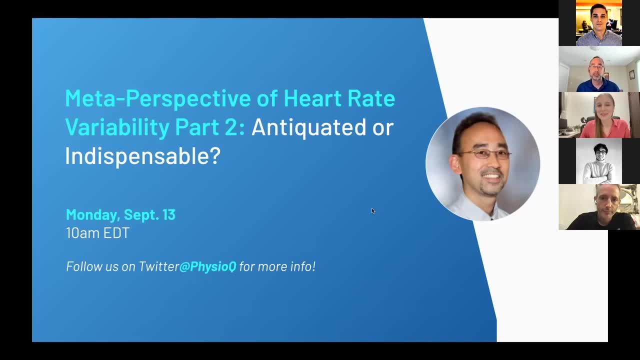 relevant and helpful information. Your feedback is invaluable. It's all anonymous and we'd really appreciate it, And I also want to state that this is the end. We're wrapping up, but we will also be on after once we say bye, So we'll be on for another few minutes to have 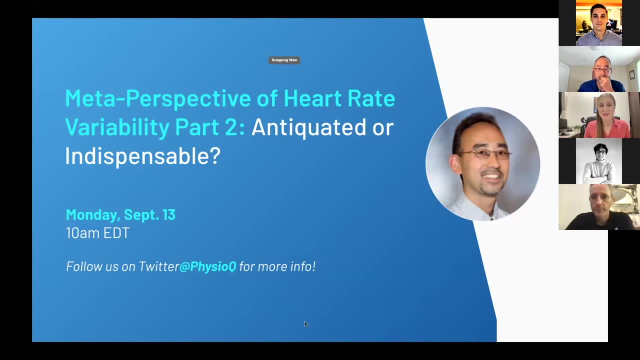 a chat or if you have any additional questions, you're free to ask those, And if you have any questions about our organization, you're also free to stick around and connect. Besides from that, I'm seeing a lot of answers in the chat, So if you have any questions, you're. 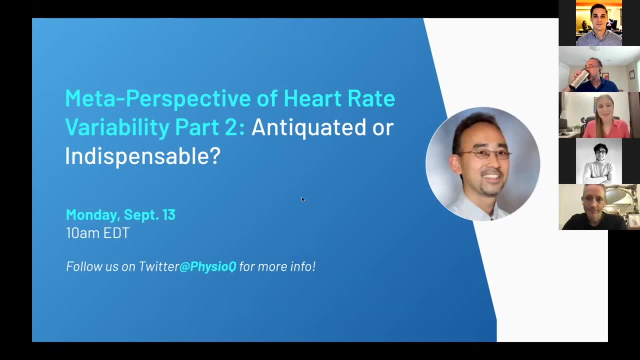 welcome to put them in the poll. Thank you so much. Other than that, I will say thank you so much for coming again. Have a wonderful Monday and goodbye everyone.